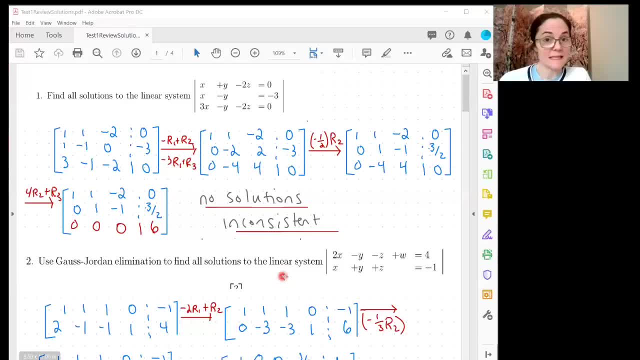 Okay, so I'm going to make this minus 2 a 1.. This is problematic. Whenever we see a row of zeros, the dots something non-zero, immediately we know the system is inconsistent because, in effect, the last line, as it reads right now, says: 0 equals 6,, which is, of course, not true. Okay, so I'm going to make this minus 2 a 1.. This is problematic. Whenever we see a row of zeros, the dots something non-zero, immediately we know the system is inconsistent because, in effect, the last line, as it reads right now, says: 0 equals 6,, which is, of course, not true. Okay, so I'm going to make this minus 2 a 1.. This is problematic. Whenever we see a row of zeros, the dots something non-zero, immediately we know the system is inconsistent because, in effect, the last line, as it reads right now, says: 0 equals 6,, which is, of course, not true. Okay, so I'm going to make this minus 2 a 1.. This is problematic. Whenever we see a row of zeros, the dots something non-zero, immediately we know the system is inconsistent because, in effect, the last line, as it reads right now, says: 0 equals 6,, which is, of course, not true. 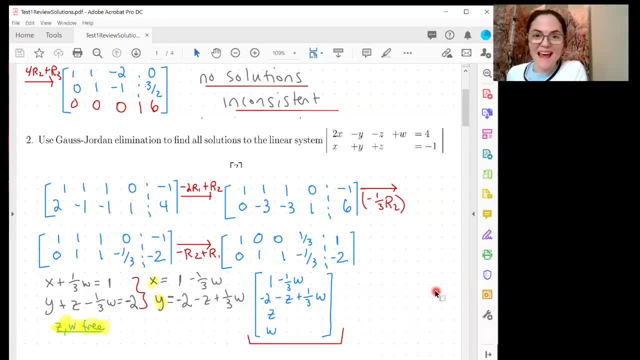 Okay, so I'm going to make this minus 2 a 1.. This is problematic. Whenever we see a row of zeros, the dots something non-zero, immediately we know the system is inconsistent because, in effect, the last line, as it reads right now, says: 0 equals 6,, which is, of course, not true. 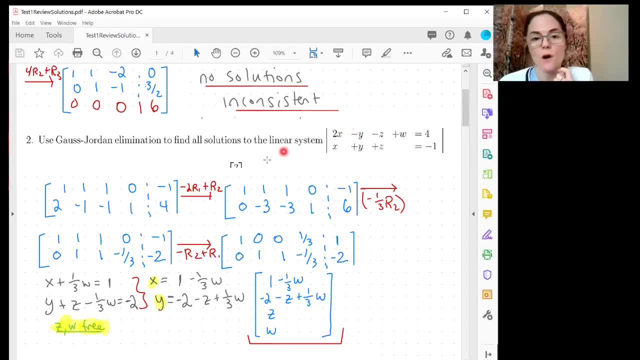 Okay, so I put the second row as the first row and the first row is the second row. I could have written it down exactly as I see in the system and then interchanged the two rows. but this is also fine, namely because I wanted to have a 1 right here, and so I just wrote the second row first and then the first, and then I want to get this to a 0, so I just take negative 2 row 1, add it to row 2, and here is what I get. 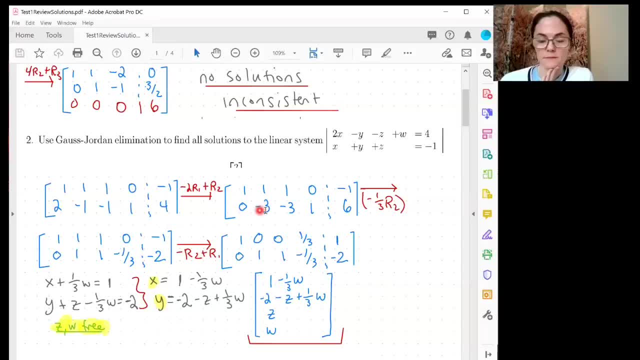 Now this is the next non-zero entry, or the first non-zero entry in this row, I should say so. I want to make this a 1.. I multiply row 2 by negative 1, third, and I get this. and then I only have one more step here to get this matrix in reduced row echelon form, and that is to make this 1 here a 0, so minus row 2, add it to row 1, and then we see leading 1,. 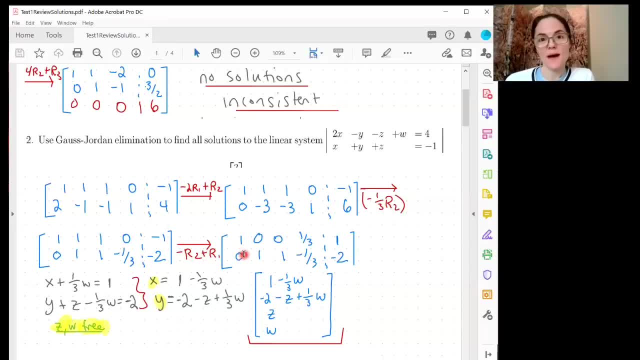 leading 1, and then 0 is everywhere else in those columns. so this matrix here is in reduced row echelon form. Now we have two free variables. You see them here. I wrote them in light green and highlighted it: z and w. right, I'm using the same. This is x y z w, x y z w, so z w. 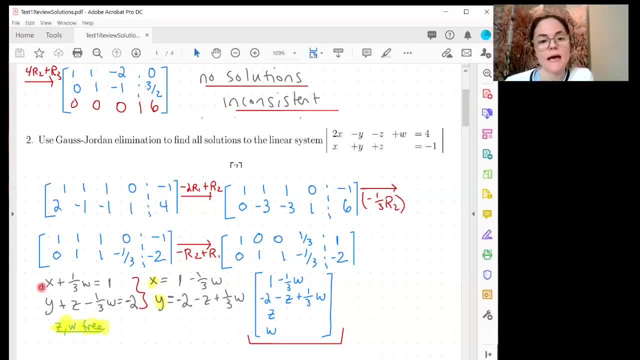 These are free, And then I just write down: this first line says x plus 1 third, w is 1.. The second line, oh, it says y plus z minus 1 third w is minus 2, and then I solve for x and y, and these are written in terms of z and w and then in vector form. this is my final answer. 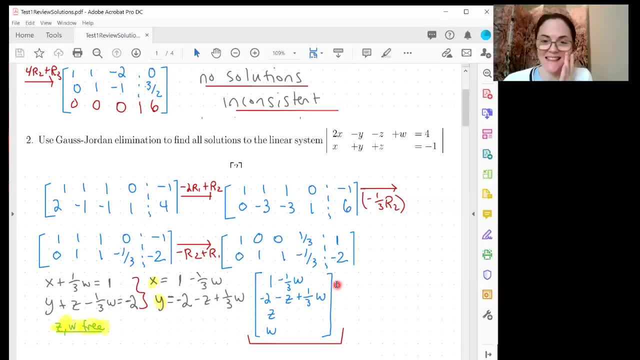 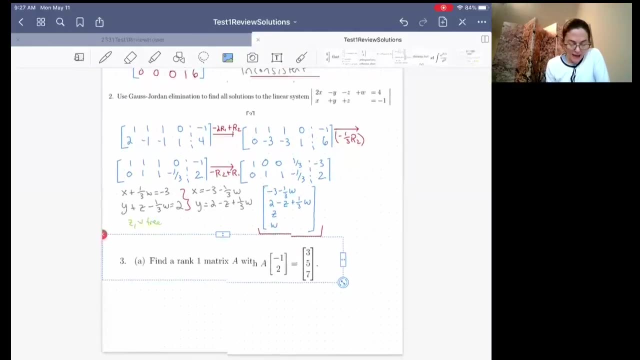 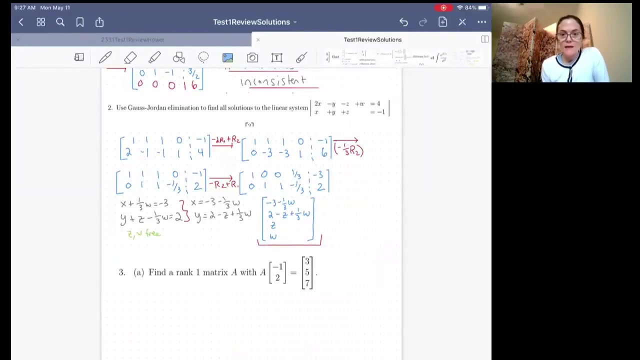 I could have called z, t and w, r or something like this, but they're already letters. So, anyways, this is my final answer. This is all solutions, and we have infinitely many of them, so I have space here just for 3a, and then I'll move to the next page, uh-oh, where we can do the rest of 3, but okay, don't make this harder than it is. 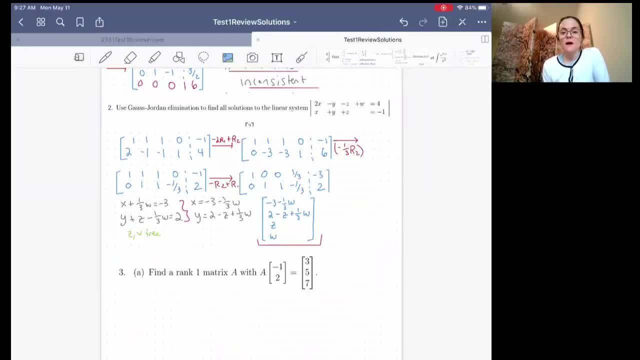 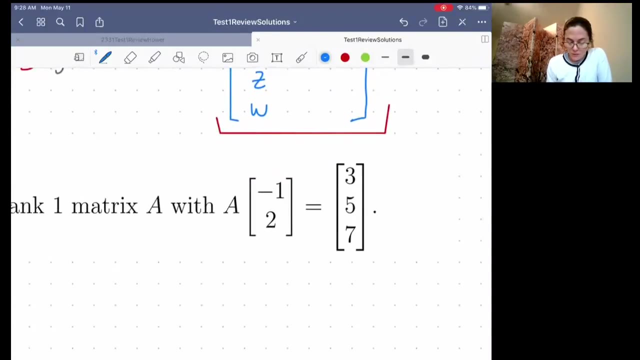 Find a rank 1 matrix with a times minus 1, 2, is this vector 3, 5, 7.. Well, first of all let's think about the size that a must be. I'll zoom in. Okay, this is 3 by 1, 3 rows, 1 column. 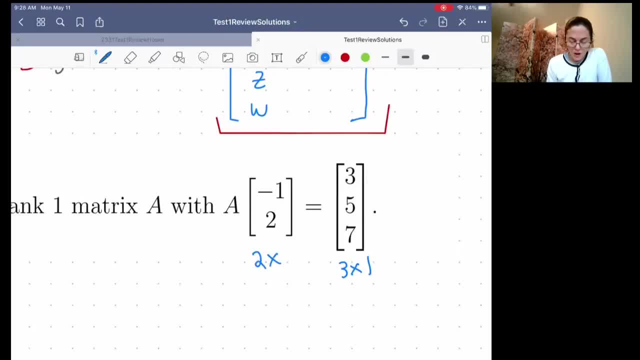 Okay, this is 2 rows, 1 column. So what size must a be? Well, it's going to have to be, it's going to have to be a 2.. Okay, Okay, Okay, Okay, Okay. 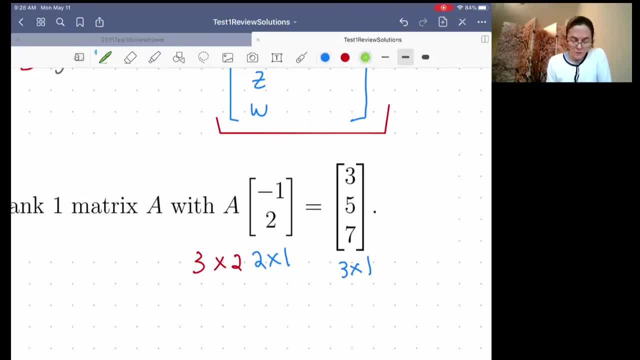 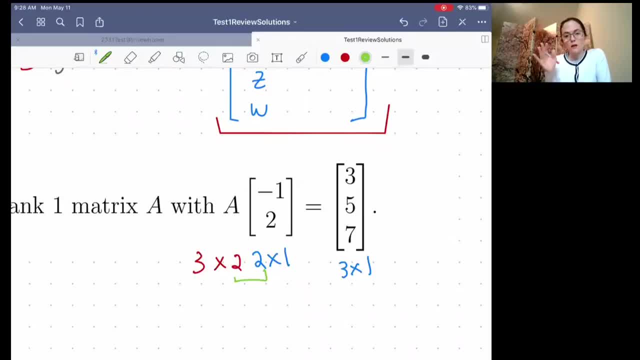 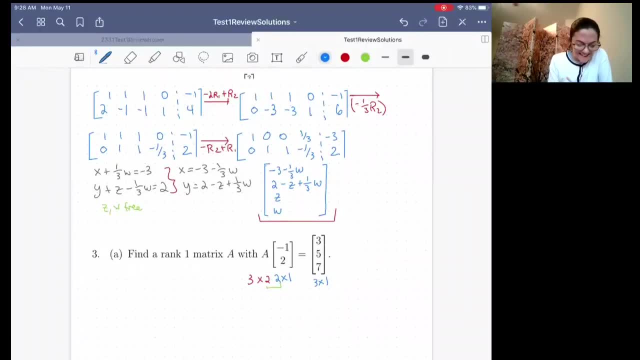 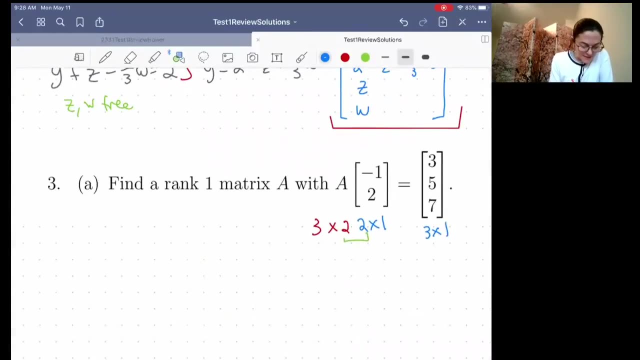 So what we need is 3 rows, 2 columns. Okay, Looks good. So now let's start this. We want 3 rows and 2 columns, such that a times minus 1, 2 is that vector, and we need. 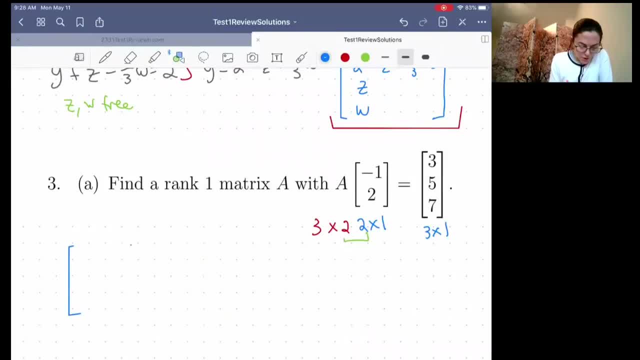 a to b, rank 1.. 3 rows, 2 columns would be something like this: Now, there are multiple things you can do. You could make the columns the same. You could make the columns one a multiple of another right. 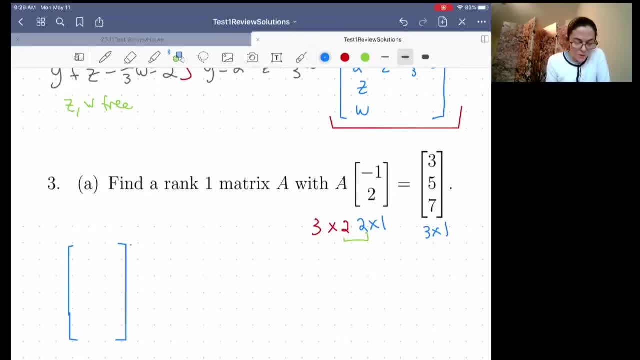 And that would both give you rank 1.. The easiest way to make a rank 1 matrix, in my opinion, is just make a column of zeros. Okay Now, as long as I put something non-zero in the first column, I'm going to be rank 1.. 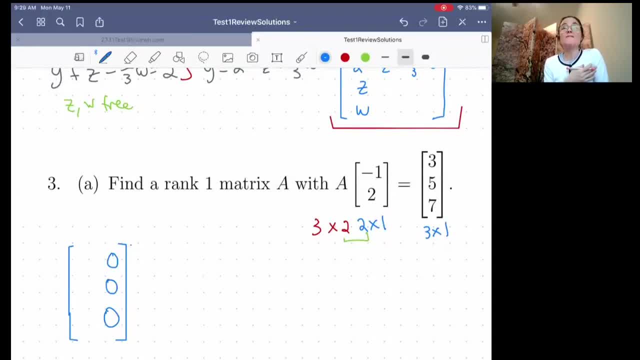 But now, if you think about what does matrix multiplication do? so I'm filling this out by columns, which means I want to think about a times a vector as a linear combination of columns. So whatever is happening here, this matrix times 1, 2 will be, if I just for the moment, 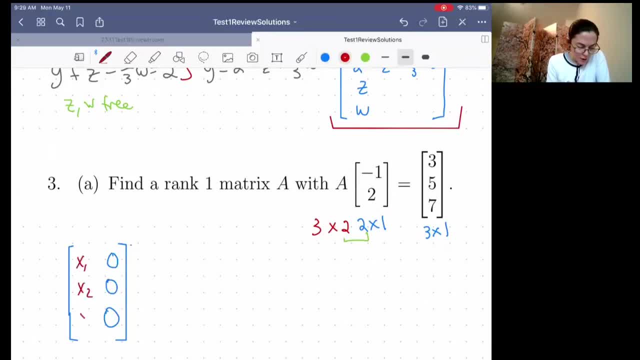 and I'm going to erase. put x1,, x2,, x3, then when I multiply by minus 1, 2, look at what happens. Linear combination of columns is minus 1, x1,, x2,, x3, plus 2, 0, 0, 0, right. 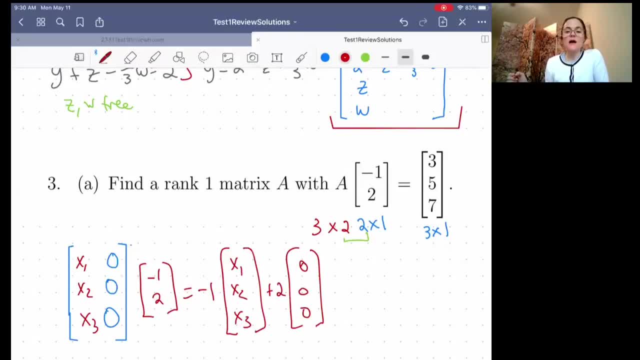 This is the way we think about matrix times a vector. when it's a linear combination of columns, We can see already. in fact, it's kind of easy to see what the values need to be If we look here. if we want this to equal this, I can just take x1, x2, x3 to be negative. 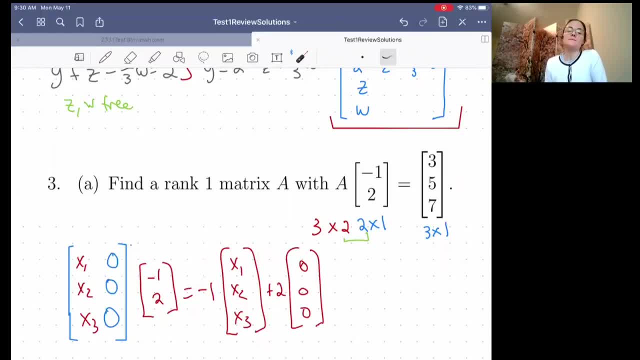 3, negative 5,, negative 7,, like this, and that's what I'm going to do. So now let me erase my thought process, which is all here, Okay, So I'm going to do this, Okay. 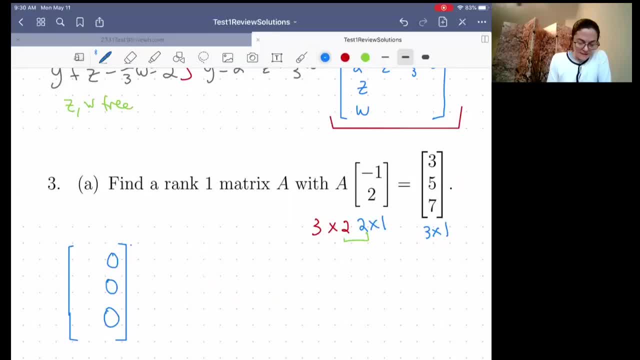 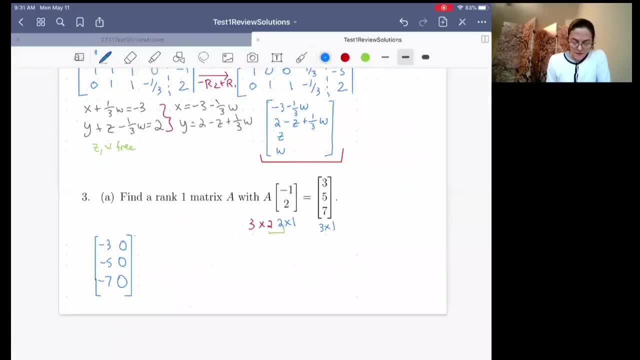 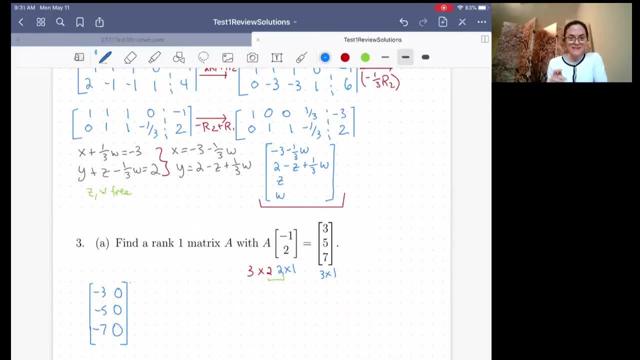 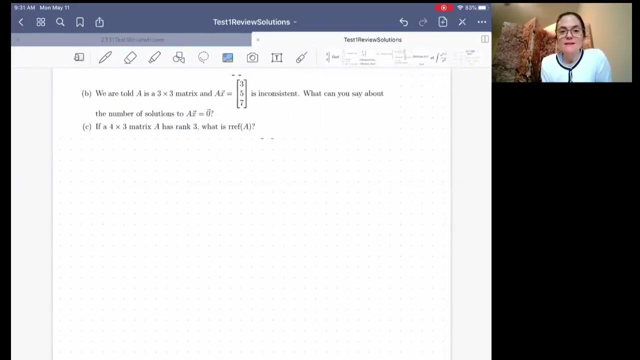 And then this is negative 3,, negative 5,, negative 7, and then, well, this is our answer. You can definitely check, although we discussed why this works just moments ago. Okay, Now for this is 3b and c. I have moved on to the next page, which is why I split the. 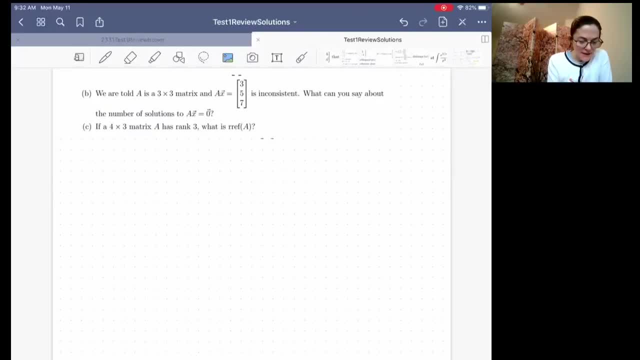 problem like that. Okay, Great, We are told some information. I'm now on b and then we need to figure out the number of solutions to ax equals 0. So let's think about this: ax, I should say, equals 3,, 5,, 7, okay, inconsistent. 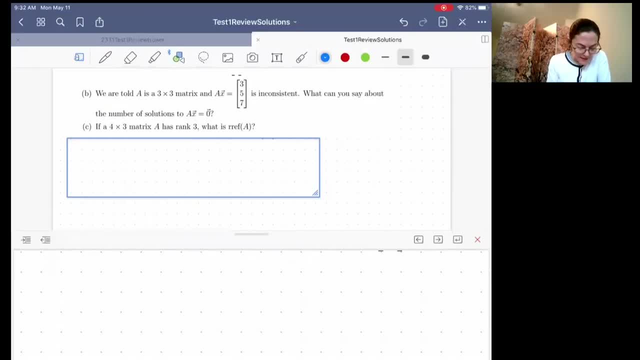 What does this mean? Let me think about this sum here, What this means. We put a: Okay, Okay, Okay, Okay. We put 3,, 5,, 7.. Okay, Then we reduce row operations to reduced row echelon form, or maybe just row echelon. 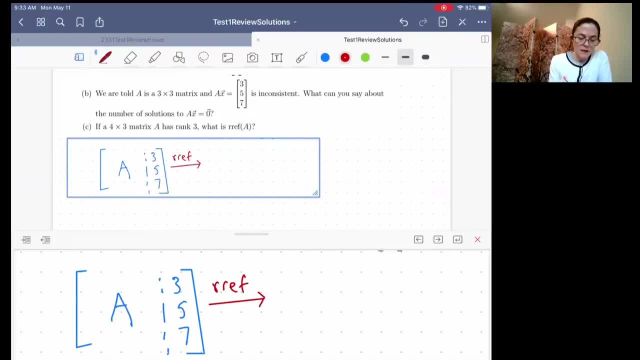 form. I'll just go ahead and write reduced, because it's fine to think that way. And now, what do we have? Well, it's no longer a, and I don't know what's happening over here, but this is going. 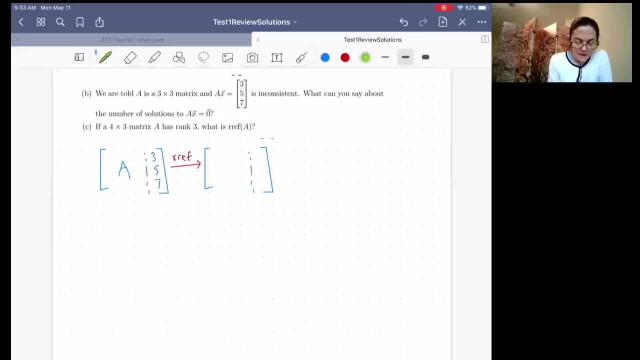 to be sum. I don't know anything about. here. This could be anything really. And similarly, here, this could be anything, no problem. but I'm guaranteed if it's inconsistent this is going to be a row of zeros, and then this is going to be, say, c where c is not. 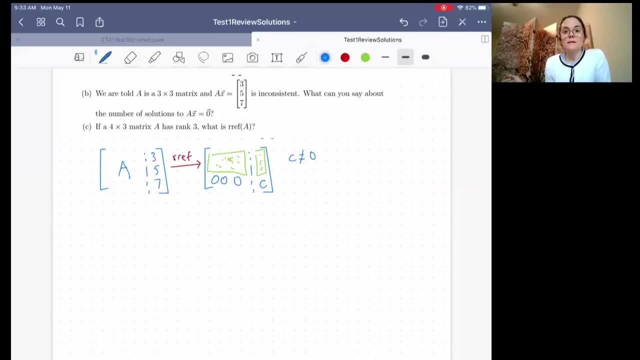 equal to 0.. Right, That's what it means to be inconsistent. Okay, So what does this mean? It means that the rank of a is going to be less than or equal to 2, because, well, what's left? 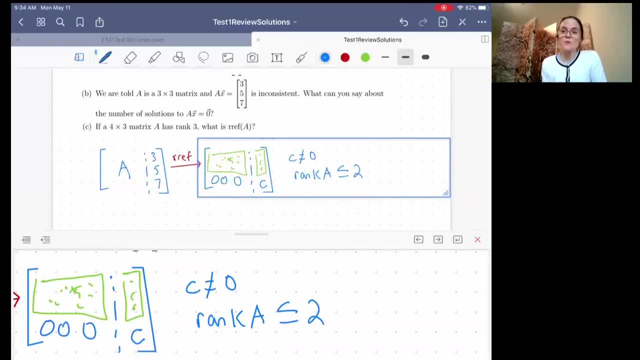 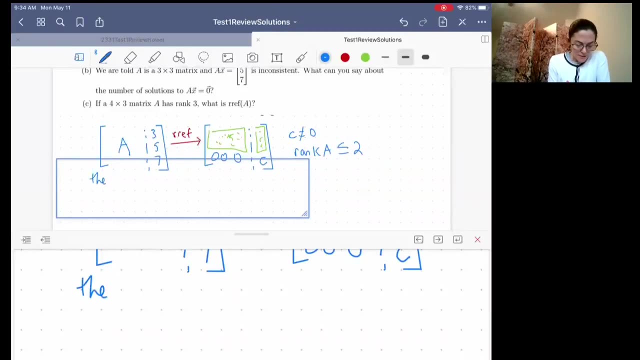 Up here, this green, which I'm not sure what is, has only two rows and there's no leading ones in the bottom row, so the most the rank can be is 2.. We also have three columns, so therefore there is at least one free variable, because 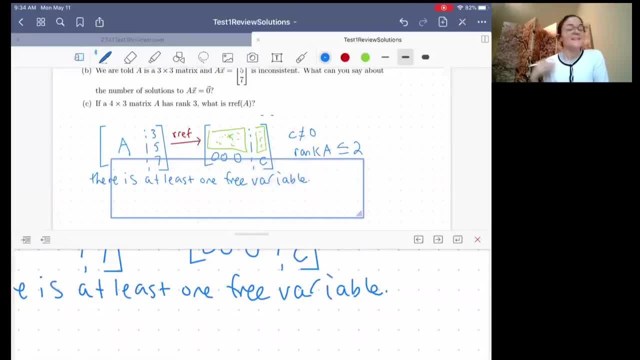 a is 3 by 3 with rank less than or equal to 2.. If you have at least one free variable, you can then conclude: ax equals 0 will have infinitely many solutions. Okay, Very nice, This was b, Okay. 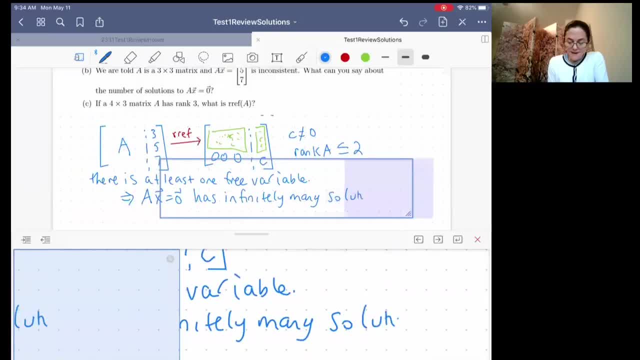 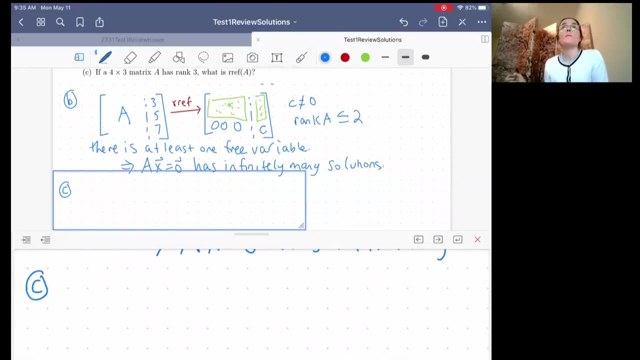 Now c These problems I'm doing now. I think they were in 1.3, they're really good for making you think about rank and understanding the kind of things that happen. Okay, Now c These problems I'm doing now. I think they were in 1.3.. 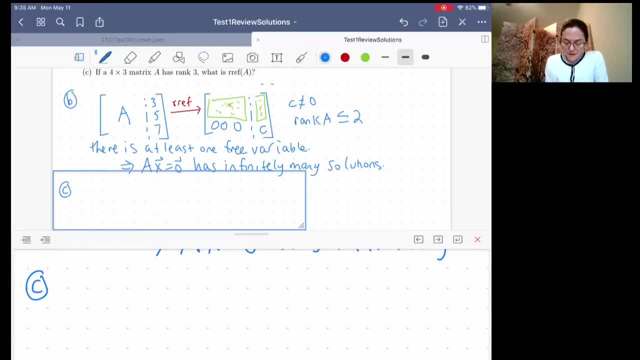 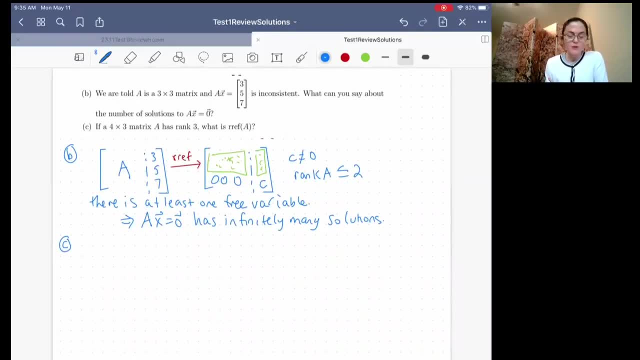 They're really good for making you think about rank and understanding the kind of things that happen. We have a 4 by 3 matrix has rank 3, what's the reduced row? echelon form? We have four rows, three columns and we have rank 3.. 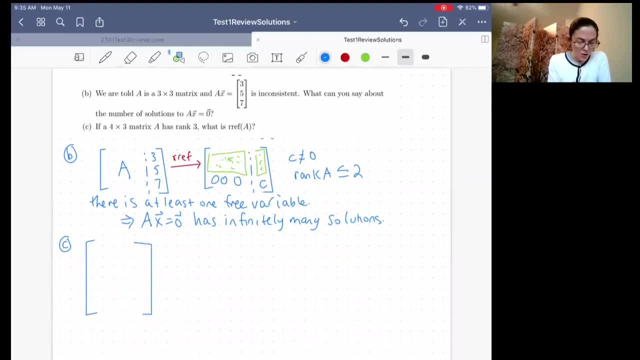 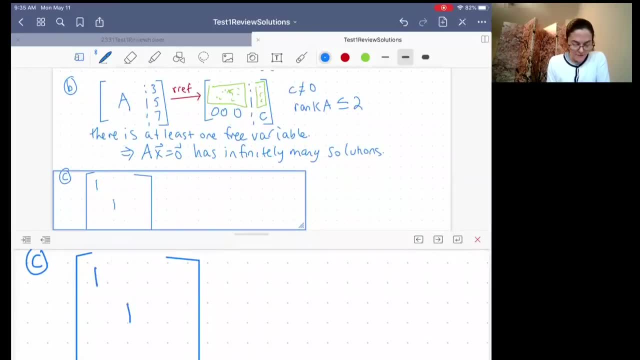 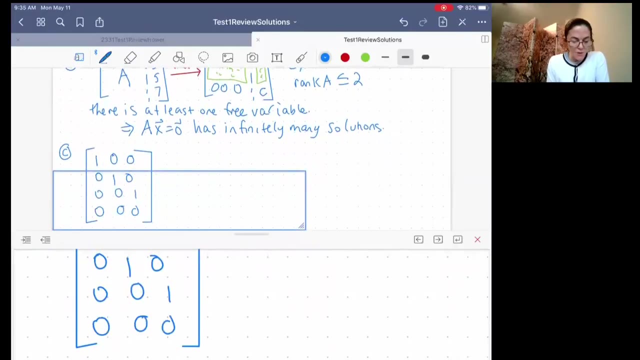 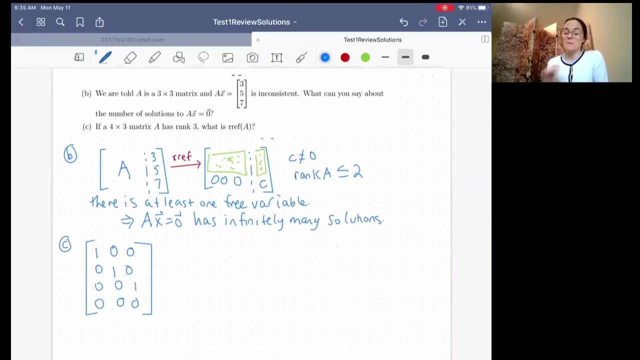 Well, there's only one option here for the reduced row echelon form We have to have like this, and then here, This is the only option. One feature of reduced row echelon form is if there's a row of 0s, it must be at the very. 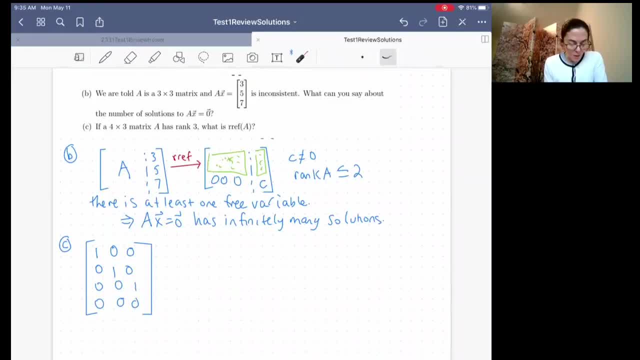 bottom. That's because every time you have a leading 1,, every row above it must have a leading 1 and 2 left. So there's no way that you could have, for instance, this row of 0s could not be above. 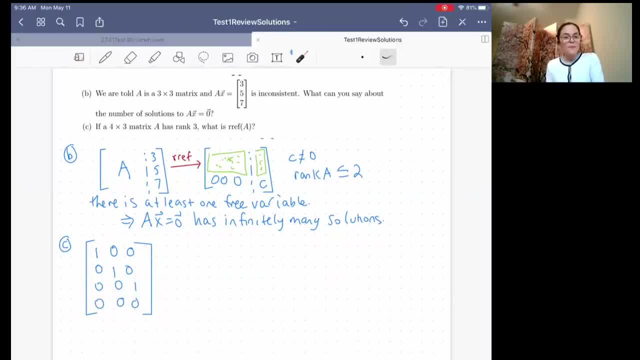 somewhere, because that would fail. I think that was the third property. So if you are 4 by 3, rank 3, this is the only option for the reduced row echelon form. Here's number 4.. We're given a transformation. 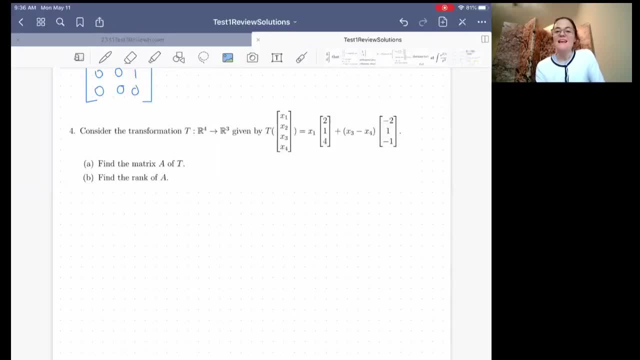 T of x1,, x2,, x3, x4 is. well, you can read, but this is a linear transformation. In fact, I can prove that by finding the matrix. but we're just told: find the matrix, so you. 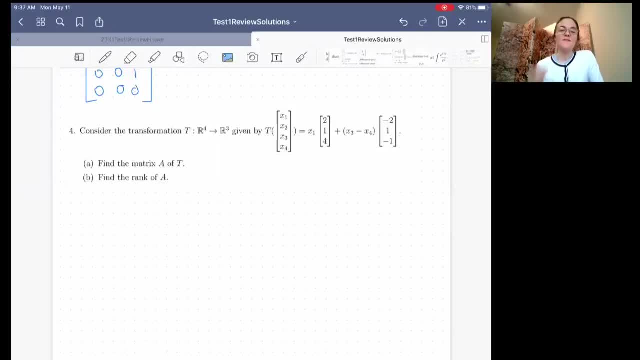 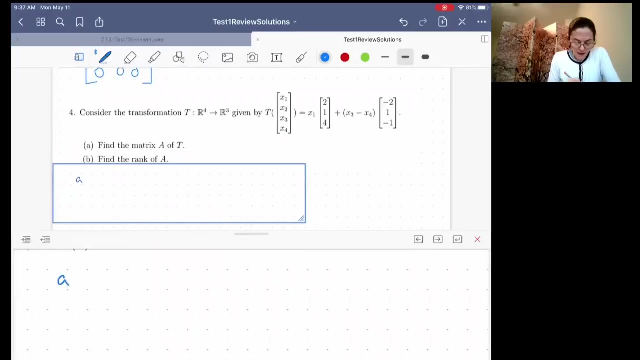 can assume it's going to be a linear transformation. If instead, it asks: is it, then you'd have to think It's not linear, Okay, Well, this goes from R4 to R3, four columns and three rows. In fact, the way you can know that, I was just trying to remember, but that's probably not the best way. 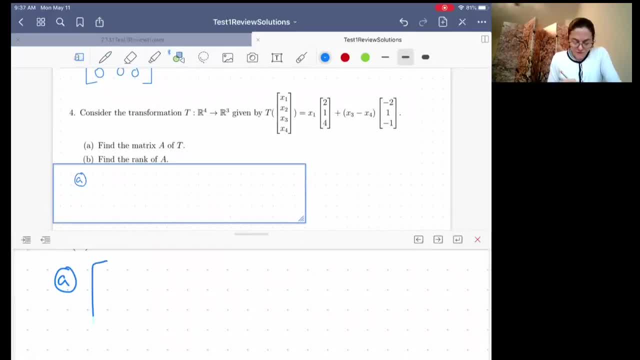 What we know about the matrix for the transformation is as follows. Maybe I don't need quite as big of a bracket, So the matrix for linear transformation we're starting off in R4.. So this will be T of E1, T of E2, T of E3, and T of E4. 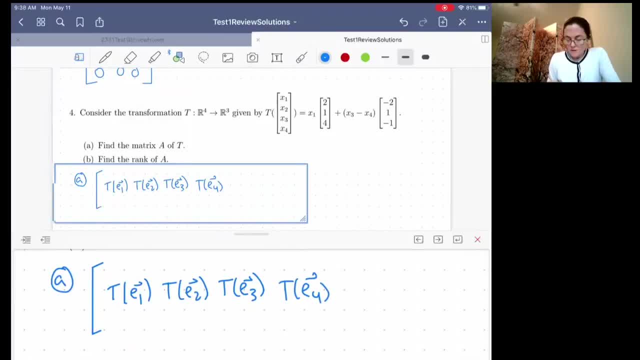 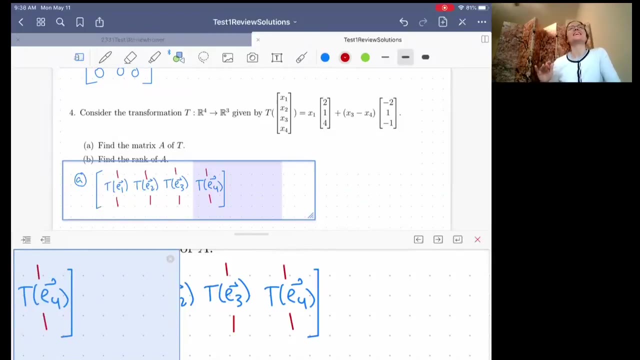 And this is really how you see. it has four columns, Because this is generally how do we find the matrix for a transformation. If you start off, let's say, with domain, If you start off with domain R N, then you're going to have, or say, R M. 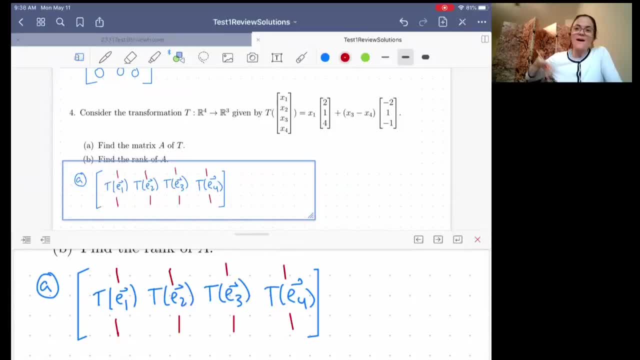 You're going to have M columns, because it will be T of E1, T of E2, T of E3, like this. This is the matrix for a transformation, So all I have to do is just see what happens to the standard vectors under this transformation. 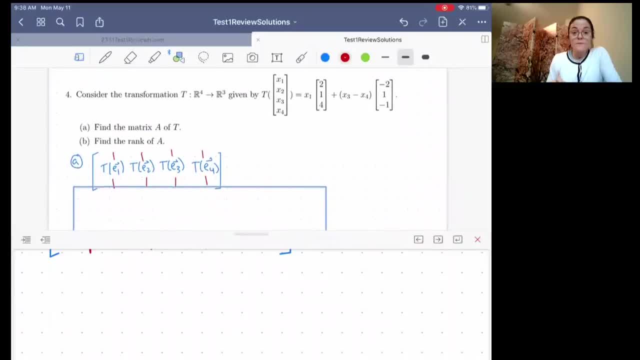 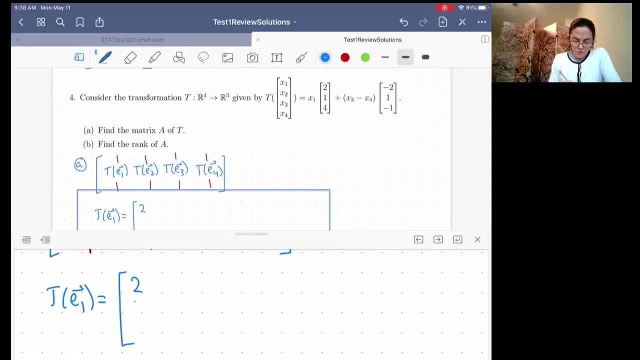 Okay Well, maybe I'll do that underneath, Make sure we can still read the problem. Very nice. T of E1.. Okay, Well, this is the vector that has. okay, this is pretty easy to see. 2,, 1,, 4.. 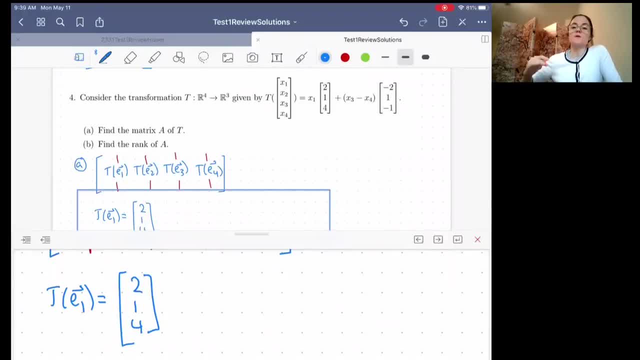 Because this has a 1 in the first coordinate. 0 is everywhere else. Okay, Now let's keep going. T of E2.. Well, you notice in the formula there's no X2 appearing, So T of E2 is just the 0. 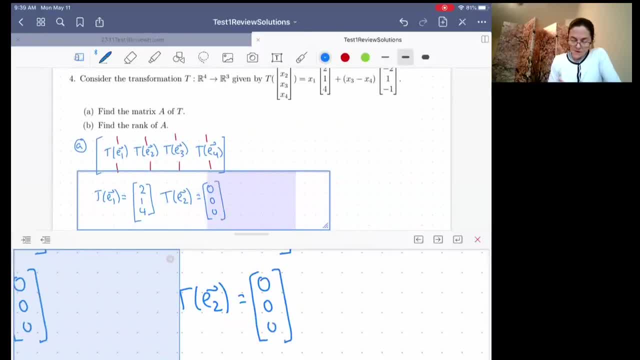 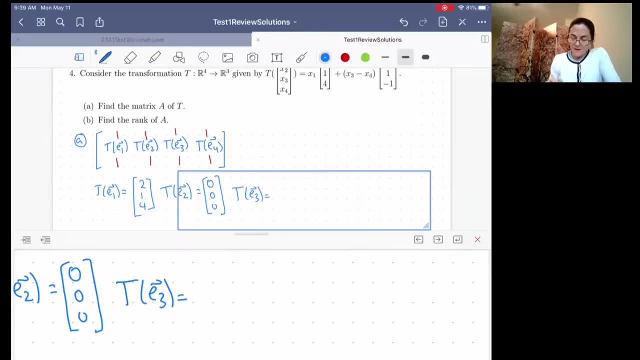 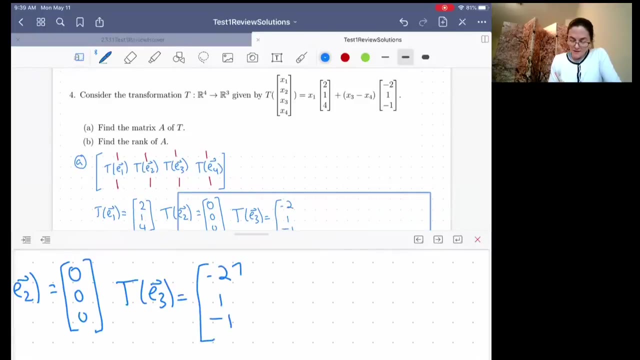 0,, all 0s And finally, well, we have 2 more, don't we? T of E3.. Okay, This is minus 2, 1, minus 1.. And finally, T of E4.. 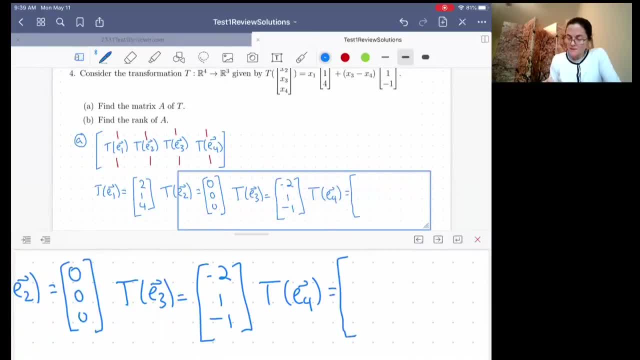 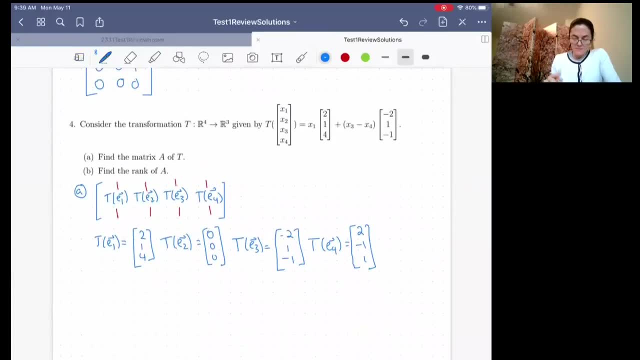 This has a 1. in the fourth component, 0 is everywhere else. It's going to be 2, minus 1, and 1.. So now we see our matrix. This is part A. This is the matrix for the transformation. 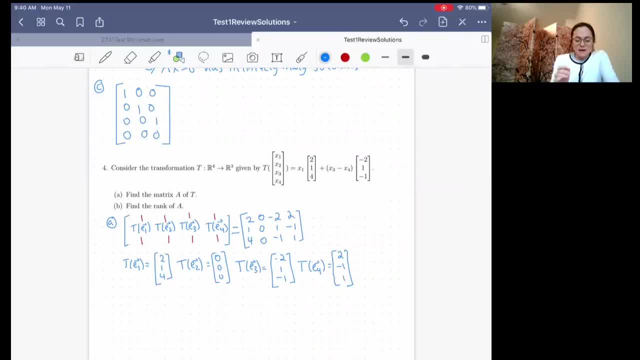 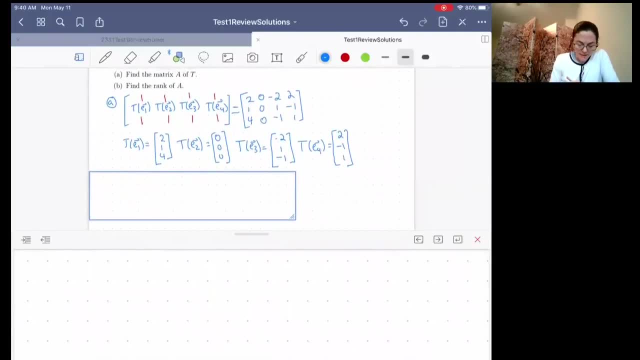 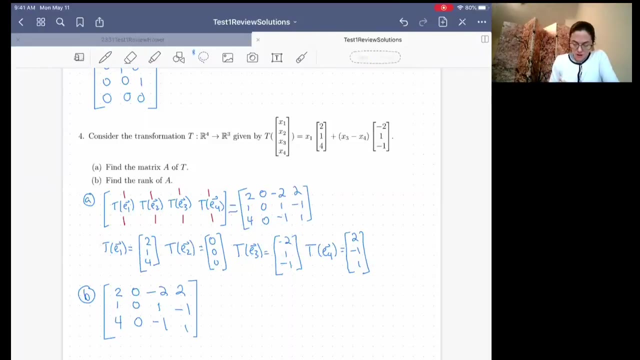 Okay, Well, part B, the rank. we could do this, in fact, very quickly, But maybe I will take two moments to say some things. What happens when I start performing elementary row operations? Well, let me see if I can make this actually a little smaller. 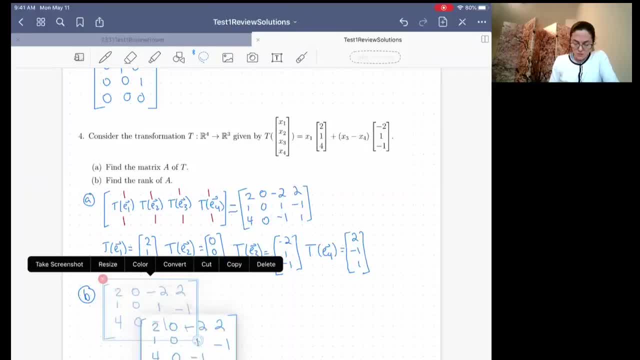 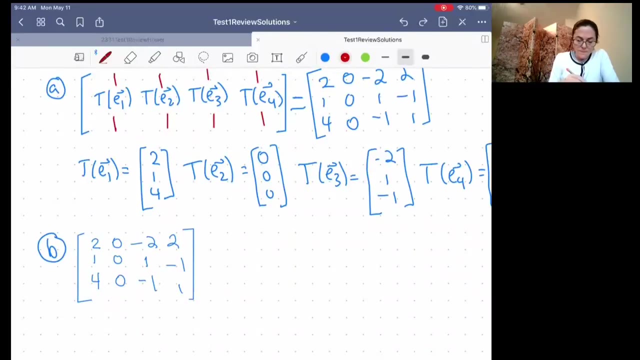 This will help us identify the. Okay, It's not going to take very long to figure this out. The first thing I can do, I'll just interchange Row 2 and Row 1.. And the first thing I can do is I'll take all the times and tails 1 and 2än. 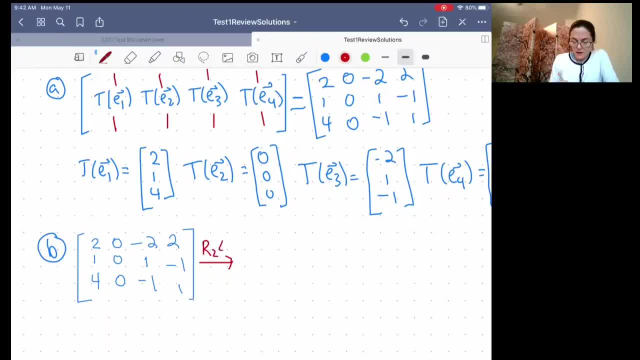 I'll put those around over here in ranked space because there's a few ways you can start, but you notice that row one already has the ones there. I could, as equally, just multiply through by row one, by a half, as my first step. 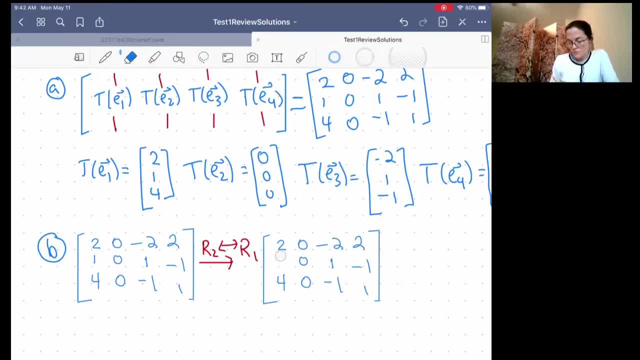 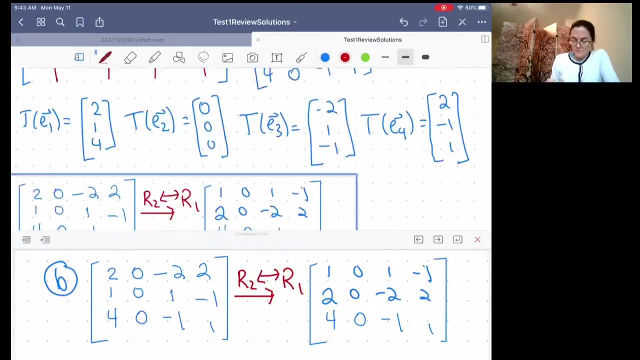 That would have been okay too. It would have been the same number of steps. I have one zero, one minus one. Okay, then I'm going to take two row. Now I'm going to have two things that I do. 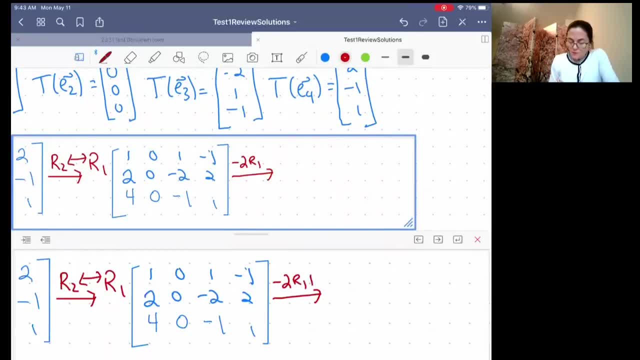 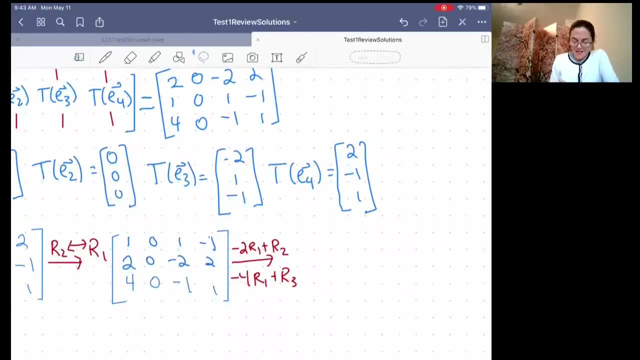 I'm going to take minus two, row one. add it to row two. I'm going to take minus four, row one. add it to row three. Okay, doke, Okay. so this is zero, zero minus four and positive four. 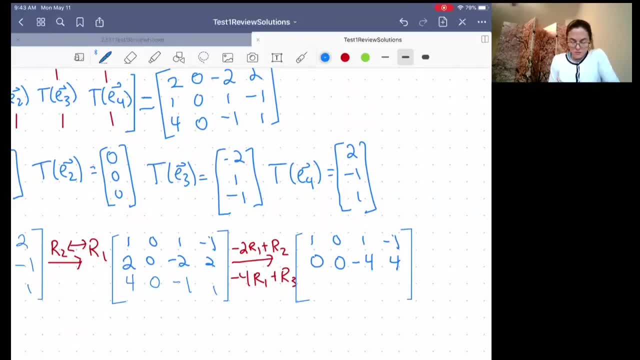 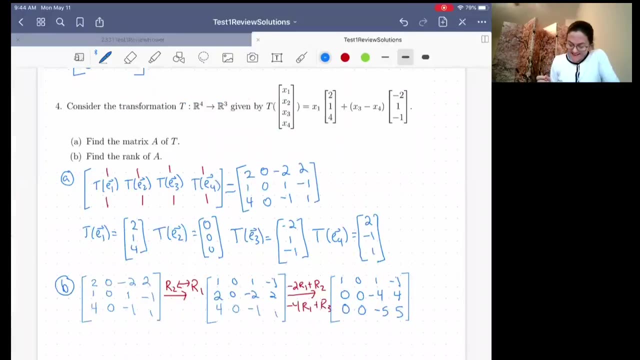 And then this one is zero, zero. Okay, Oh my goodness, Can you see already what the rank is? Do I need to show one more step? Maybe I'll make this all a little bit smaller and show one more step, because hopefully, look. 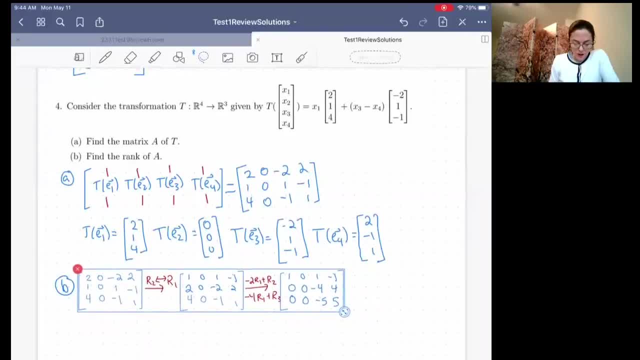 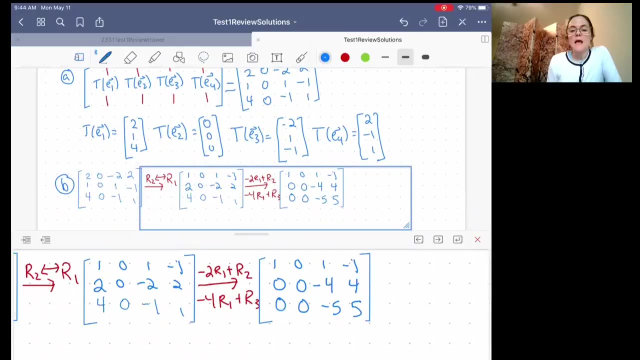 What do we see? We see row three. Row three is now a multiple of row two, So we should be expecting that the rank is only two. But let us. I'm going to do one more step to convince us of that. Normally, if I was going to go all the way to reduce row echelon form, I would be multiplying. 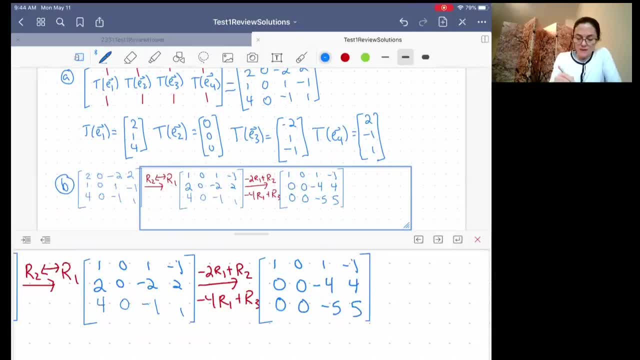 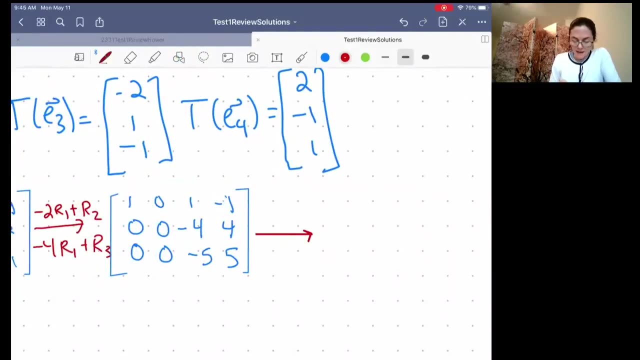 row two by negative a fourth at this moment. What I'm going to do, though- because I want to be done with this last step- is I'm going to Okay, So I'm just going to take- Let's see, I'm going to take minus five over four. row two. add it to row three. 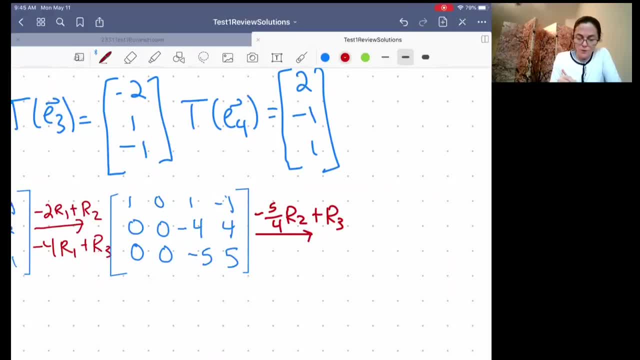 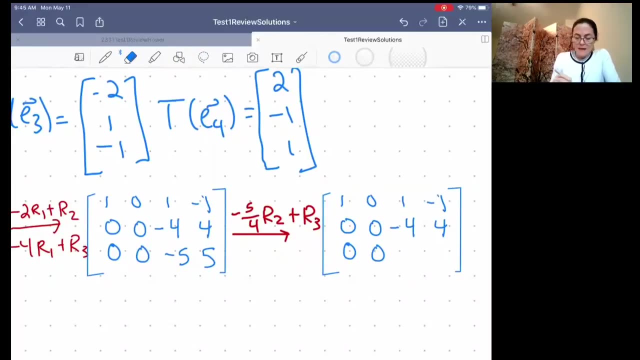 Yes, that's the right multiple. And then what happens? Copy: Okay, Just enough space. we get zero, zero. and I'm going to stop here because I was just to determine the rank. you don't have to go all the way down to reduce row echelon form and I'm 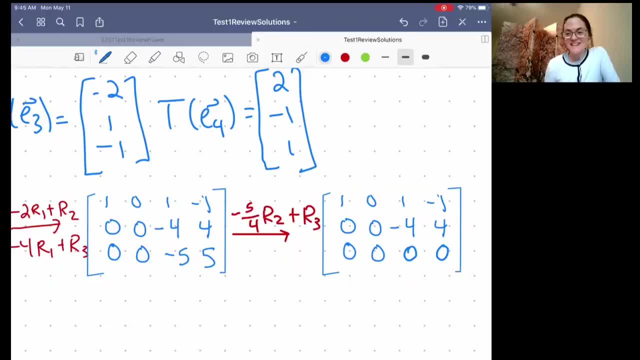 not trying to solve a linear system, for example, but you see, now we see the rank. immediately the rank is two. if you wanted to go to reduce row echelon form, I'd have to- just, let's see, make this a one and then make this above a zero. but 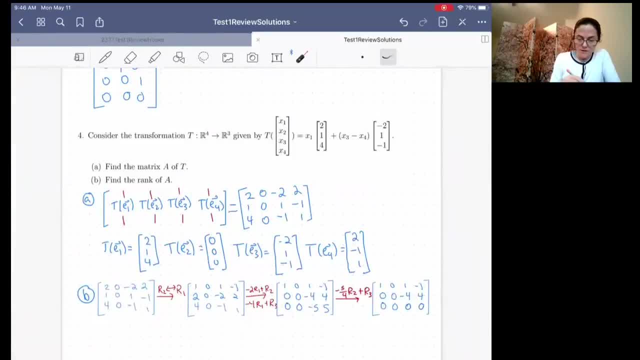 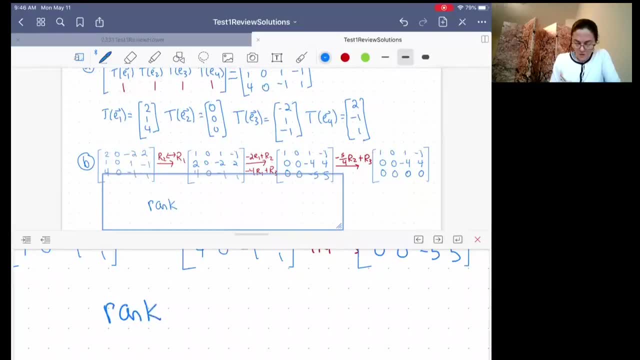 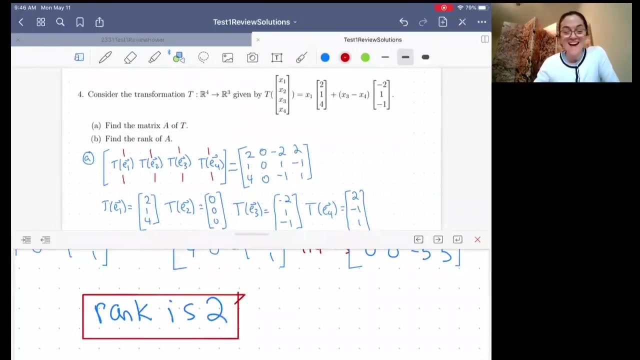 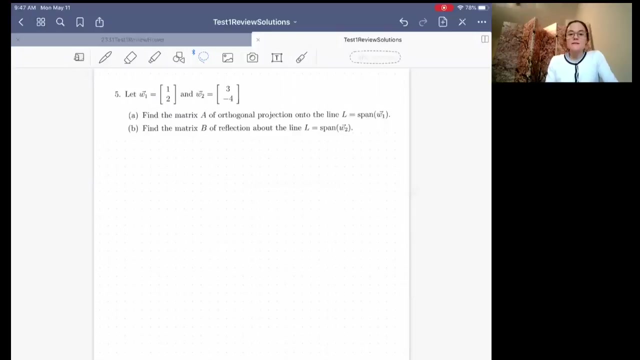 I don't have to do that to figure out the rank. so I know the answer here: the rank is two. okay, so this is the end of number number. number number four. now we will move to number five. okay, we need to find the matrix. well, we have to find two different matrices. we. 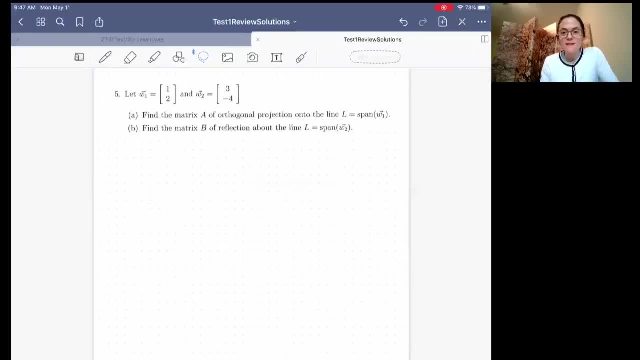 have an a and a b. first we want to project onto the line um span by this w1, and then we want to reflect about the line span by the w2. okay, wonderful. so we can have a few choices here. we can use the w1 and the w2. 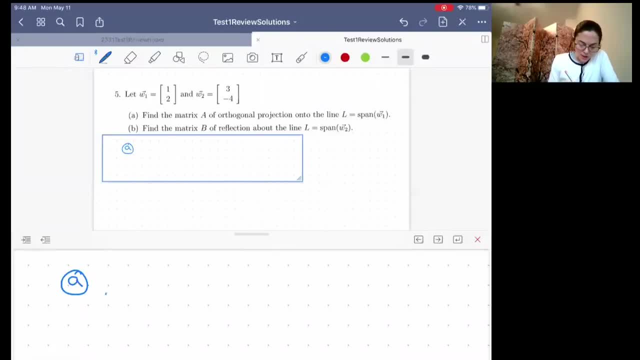 so this one must be a place somewhere to start豈, and that would be pigeonék swan. w2 and w2 squared, and this is projection. when you get a, you use an, a, ez or рi equinal structure. that'sべてghетаų to the matrix of projection is one over w1 squared and w2 squared, and then this was w1 squared, w1, w2, w1, w2 and w2 square. 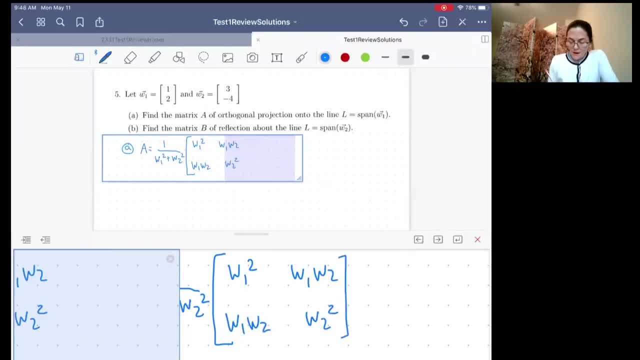 this projection, if kita is um projection, when you use a project, when you use a any vector as long as it's non-zero, and you want to project on the line, that is, and this, this meant all multiples of that vector. this is one option. another option is to make the 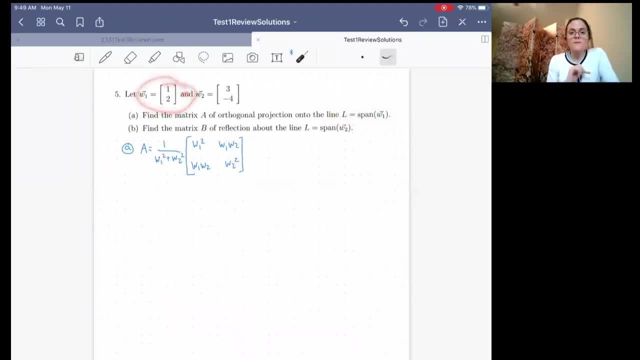 vector unit. this is not a unit vector. we would take and take this vector divide by its length and if you're working with a unit vector that is along the line, then you can leave off this, or, in effect, this is one when you have a unit vector. so you have really two choices. maybe i will just 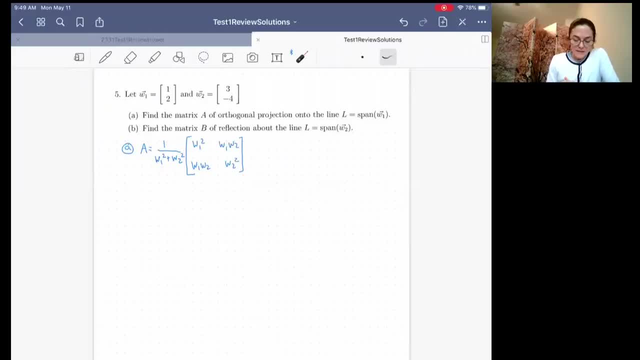 work with this vector directly because, because this formula is not too bad and this is all i'm doing with it. if i were doing more- which we are going to come back to this a lot in chapter five- then i would definitely make that vector unit because i would have more things to do with it. 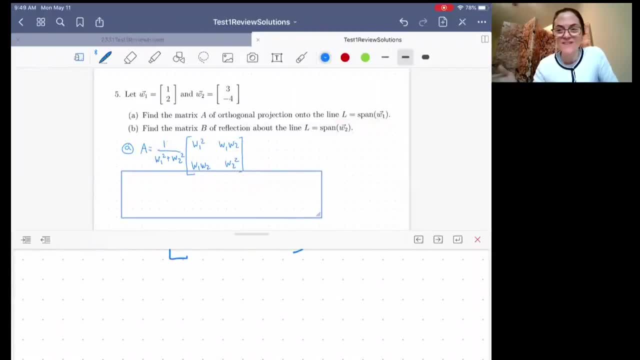 but for now, i'm just gonna, i'm just gonna use this formula and i'm gonna use the vector w1. i just hand you, you to me. okay, very nice. so what is this in this case? this is well, it's one over one plus four, and then i'll try to make my straight lines w1 squared, w1, w2, w1, w2 and w2 squared. 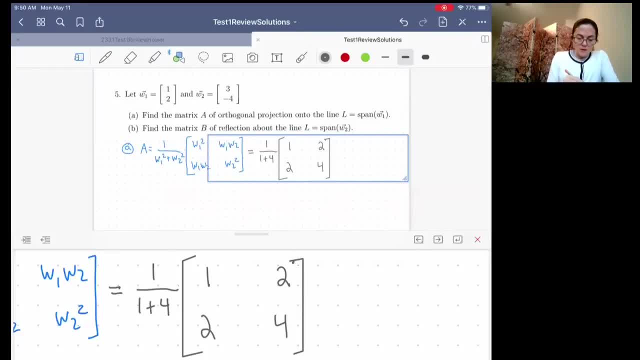 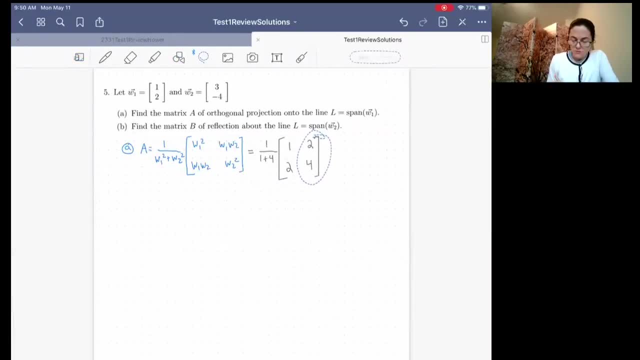 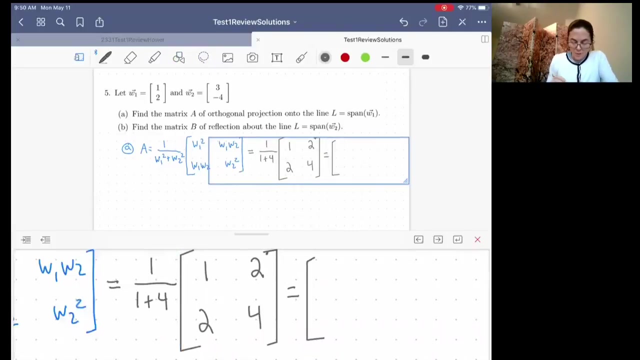 and then if you just um, pull this inside, let's see, i didn't need to make that so far. oh well, i guess that's okay. if i just pull this one-fifth inside, then my final matrix looks like this: it's just a fifth times each coefficient, so this will be one-fifth. 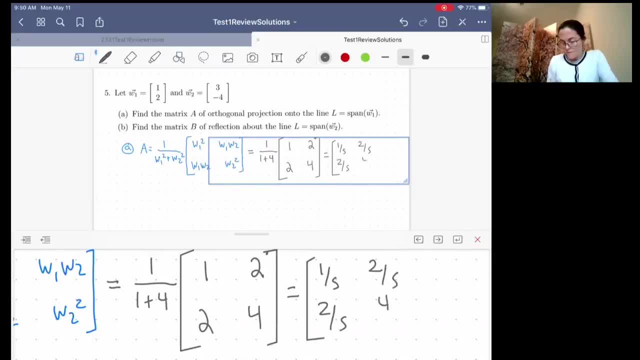 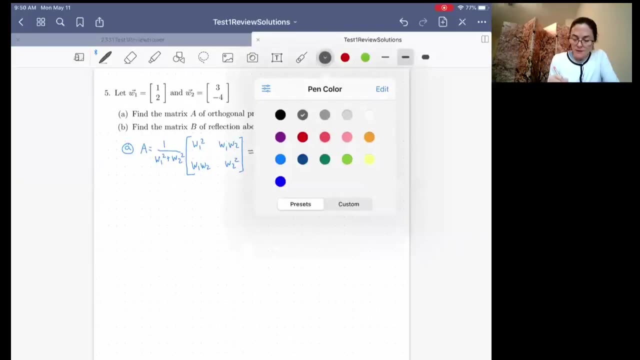 two-fifths, two-fifths and four-fifths. so this is the answer to part a. this is the matrix of orthogonal projection onto this line. okay, now b? there's also, or similarly, a few ways that you can do b? um, if i'm not projecting onto the line first and finding that matrix the way? oh, i didn't mean. 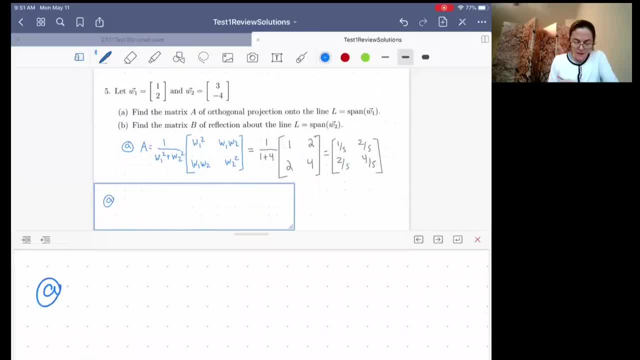 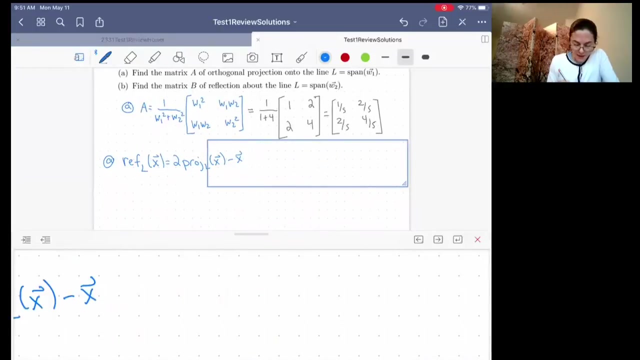 to make that in the middle, the way i would remember it. so the formula for reflection of some vector x, it's two times the projection, or this is one way to write it: it's two times the projection onto that line minus the vector. okay, and we also discussed that to find the matrix. so the matrix has the form a b, b minus a. 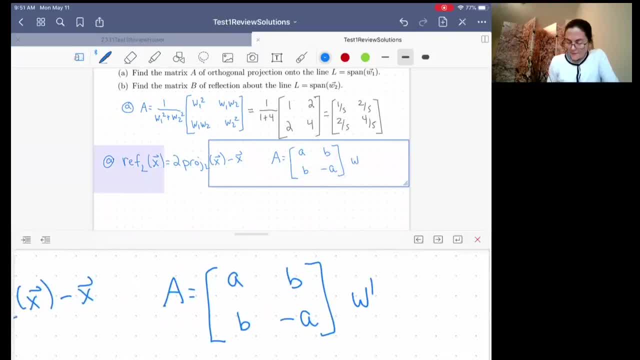 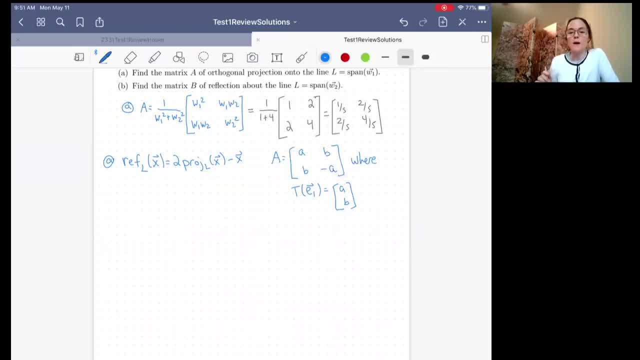 because that's, by definition, this matrix for the transformation. But we can use. in fact I did in part A, I used what I know that the matrix looks like for reflection. So this is here. this is what I want to do. 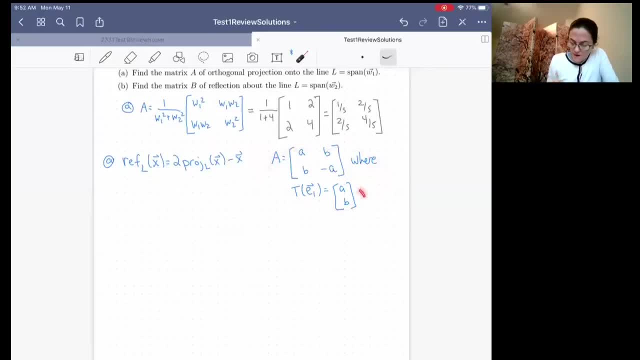 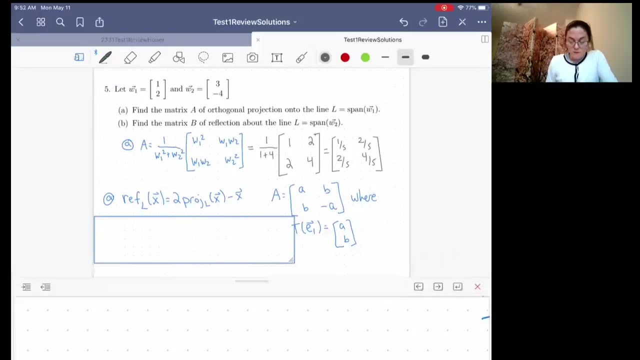 So all I need to do is figure out T of E1, and then I will have my matrix A. Okay, this is my strategy, But now it's I have a new vector, right, maybe I need to move this down. 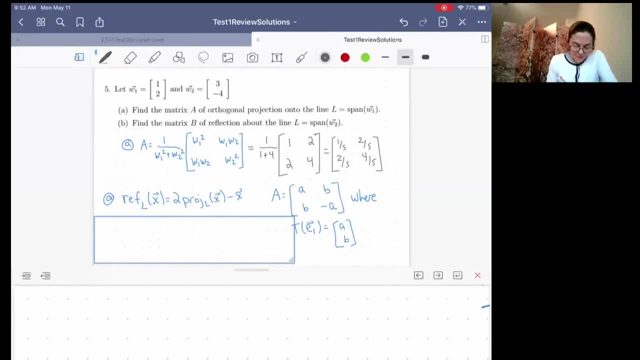 You can see everything. it looks good. So the reflection- this is in B on the line T of E1, is going to be two times. well, okay, this is not unit, it's fine. So this coefficient is multiplied by W2, and then maybe I'll write out the formula. 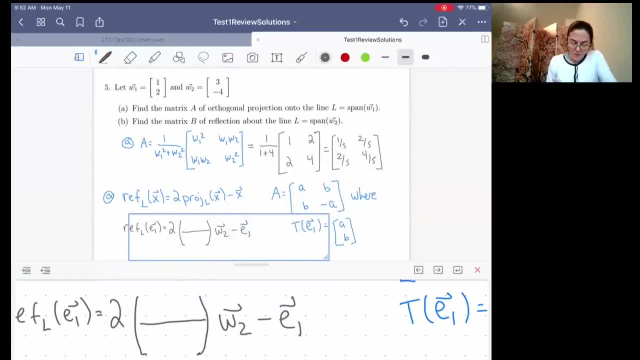 and then we'll compute it, and then minus E1.. And the coefficient is E1 dot W2 over W2 dot W2.. This was the formula for our projection. well, two times the projection, and then we subtract off the vector. 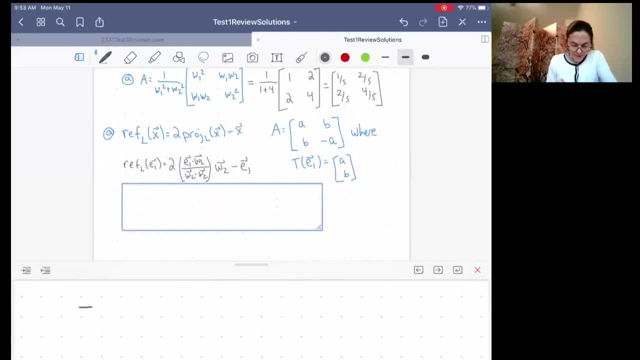 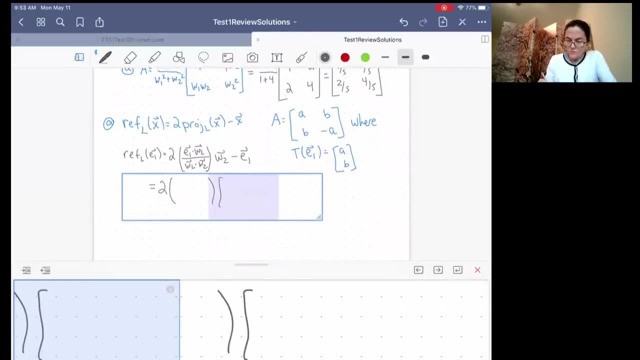 Okay, so let's do this. here: We get 2, and the W2 is 3 minus 4.. Oops, This is 3 minus 4.. And then minus Minus E1 is just 1, 0.. 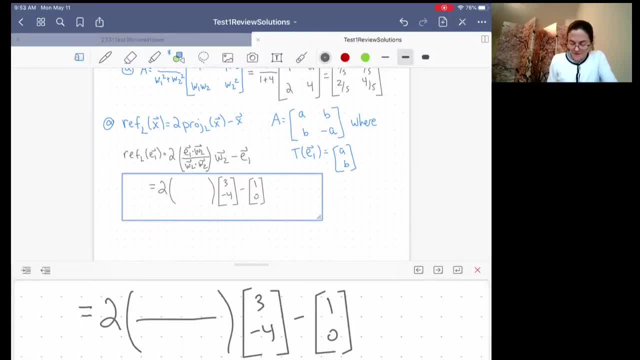 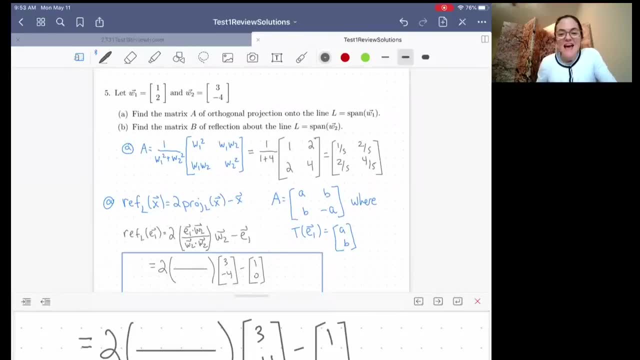 Okay, And then we also have this divided by Okay. so now let's look. Okay, we can see everything good. Well, when I take E1, dot, W2, I just get 3 times 1. So in the numerator here I have 3.. 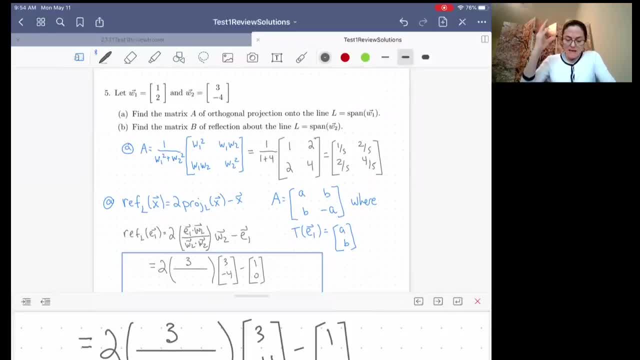 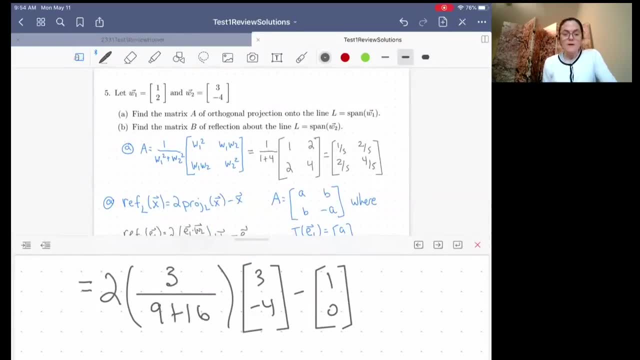 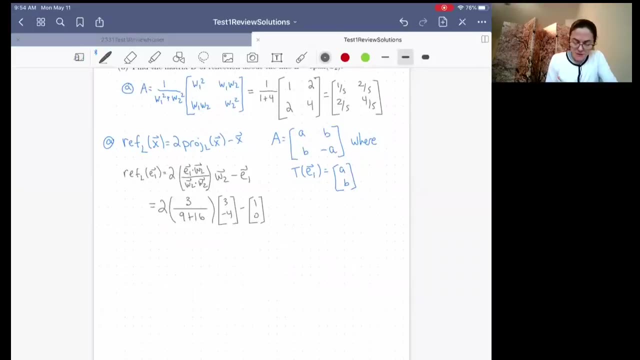 And then W2, dot W2, I get a 9, maybe I'll write that here. I get 9 plus 16, that's 25.. Okay, so now maybe I will do this in two more steps We get: 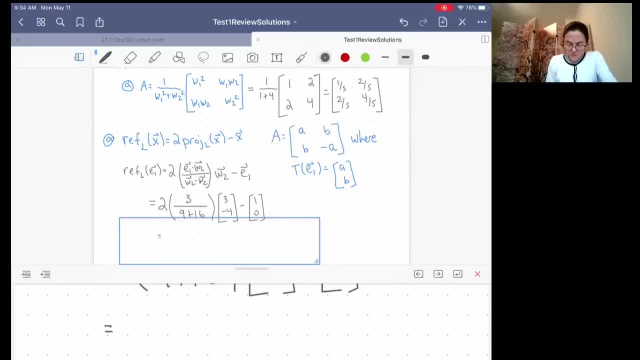 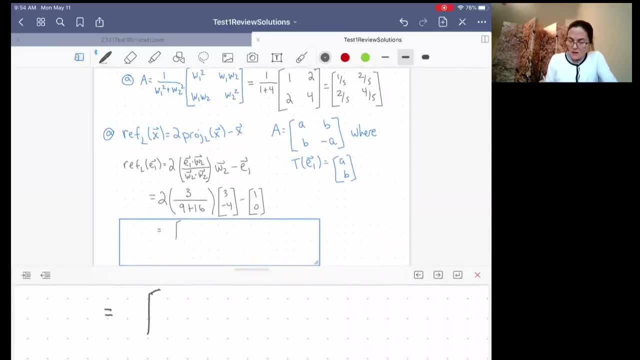 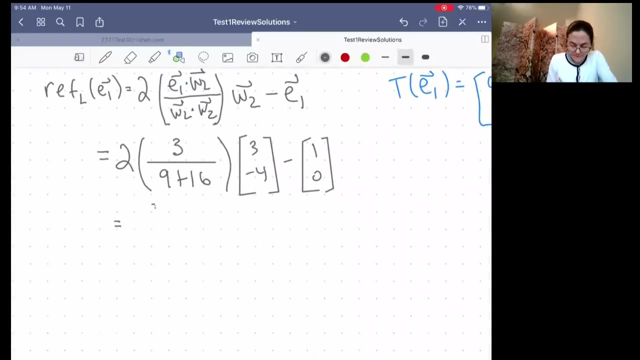 This is 6 over 25.. Oh, let's just make this first vector. I think that would be A nice way to go about it. We'll zoom in for this part. Okay, great, Okay. so here we have 9, and 2 makes 18.. 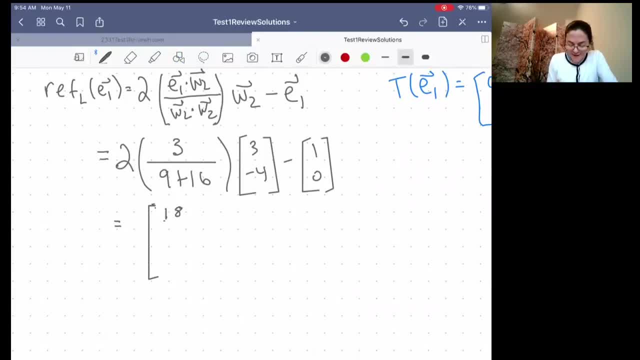 Oh, 18 over 25.. And then the second component: we see it's 12 and 2 minus 24.. Over 25. Over 25.. And then we subtract off 1, 0. And We get. 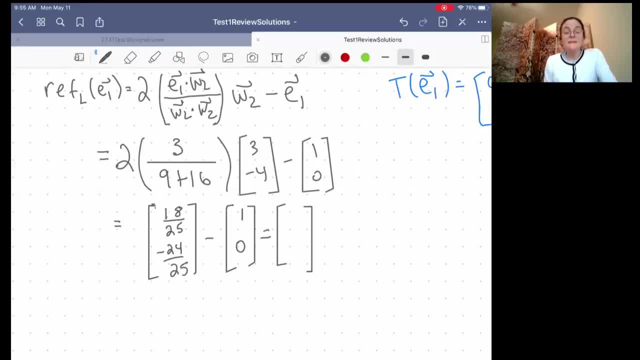 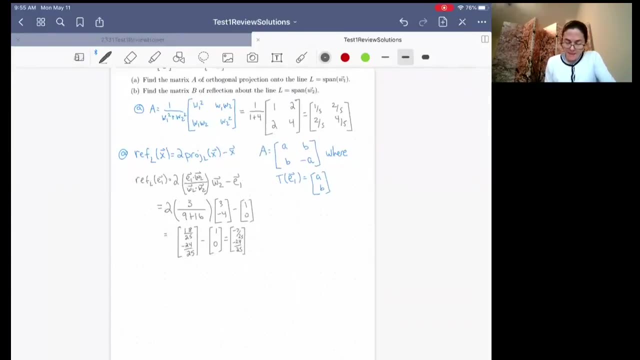 Well, 18 minus 25 is negative 7.. Okay, And then we have negative 24 over 25.. Okay, so this gives us the A and the B. So now let's write down our matrix. Right, We have everything we need. 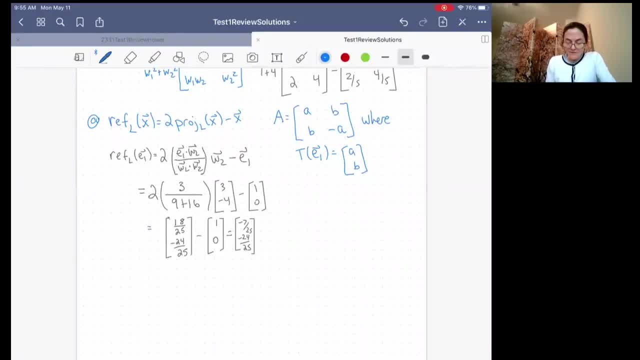 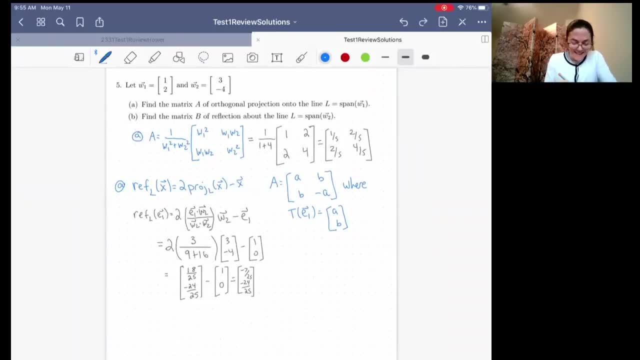 Maybe I will go back to blue The matrix of reflection. Now we can still see the problem. So A Let me get this actually. Oh no, Now we can't see the problem anymore. But that's okay, We have all the work. 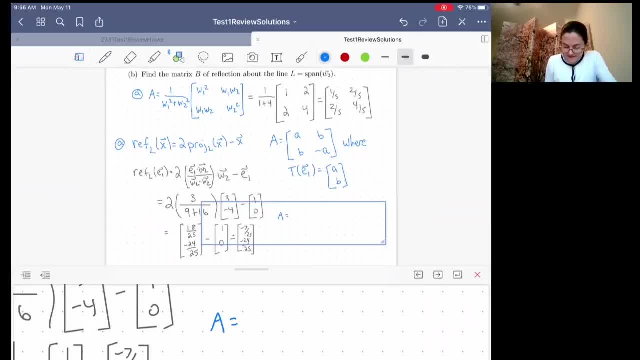 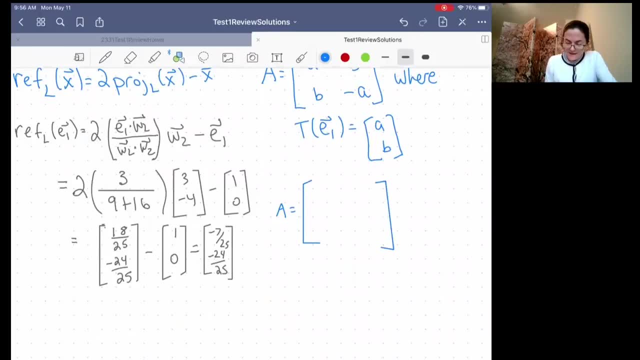 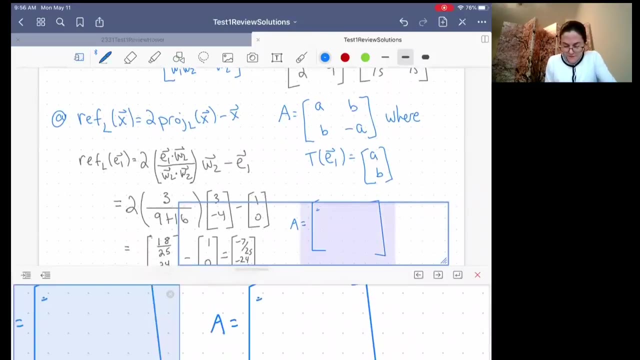 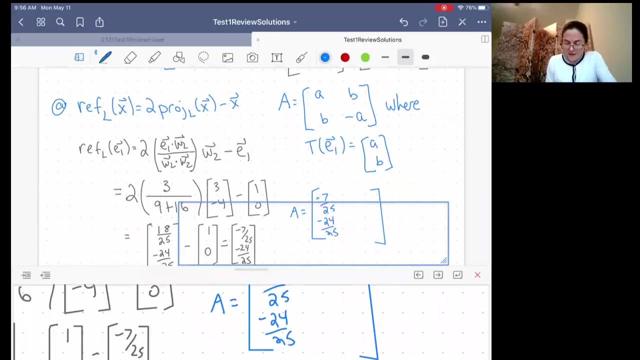 We can see. Actually, here It is, Let's fill it in: Minus 7 over 25.. Minus 24 over 25.. That's A, B And then B minus 24 over 25.. Minus A. 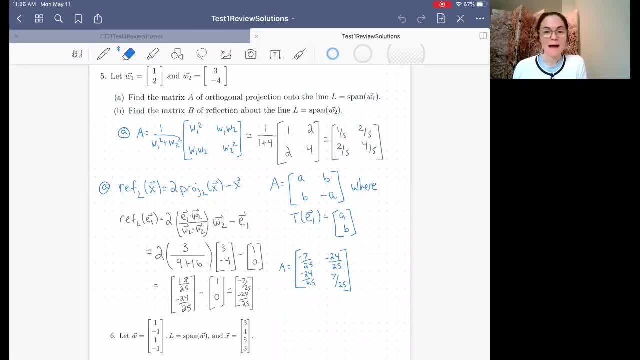 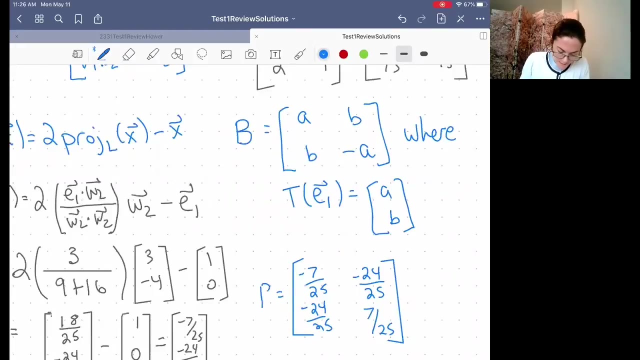 7 over 25.. My apologies, Of course. And B, The matrix is supposed to be B, Not capital A, So let me just change this: This is B And this is B, And now this matches the problem. Okay. 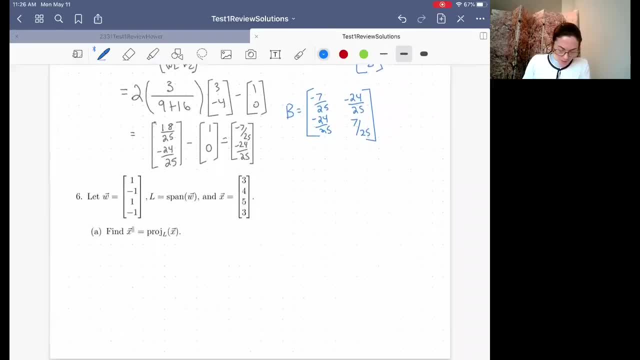 Sorry about that. Well, I don't have all that much room here, So let's do 6A And then we'll move to the next page and do 6B and C. Here we have two vectors in. Well, we have a vector in R4.. 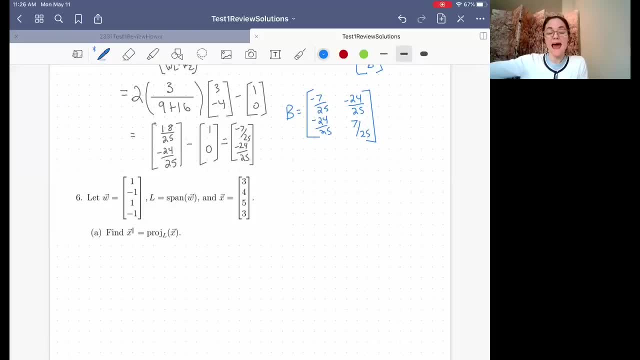 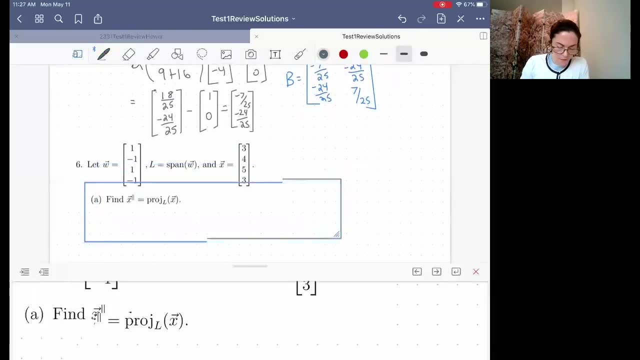 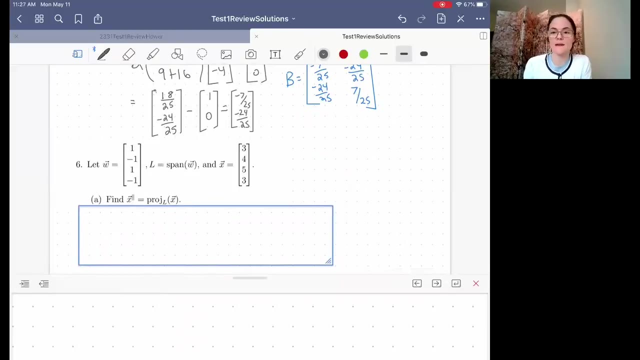 And L is a line in R4. And we want to project X onto this line And, as I was saying when we worked the last one, we're going to spend a lot more time with orthogonal projection in Chapter 5.. But this we can in fact do now. 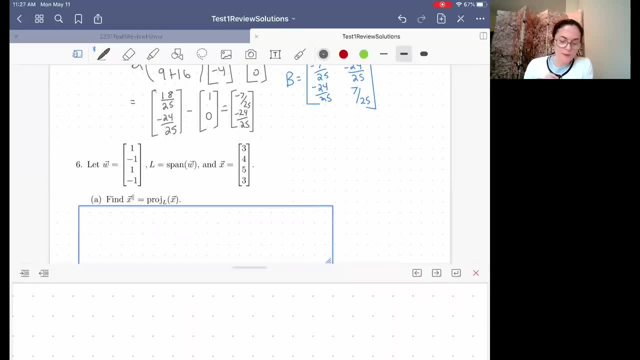 I will. well, first of all, W is not unit, But this is okay, We can do this without. So the formula for the projection, one way to write it, is, as we see, like this: It's the projection of this vector X. 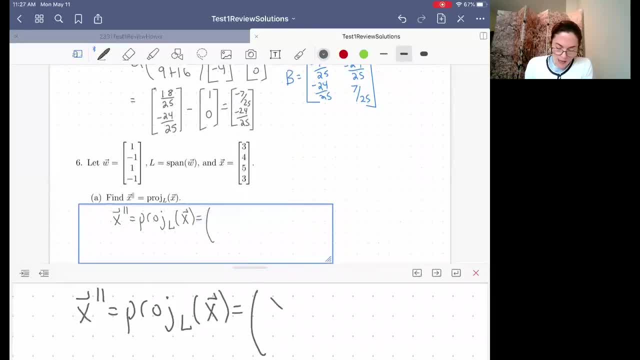 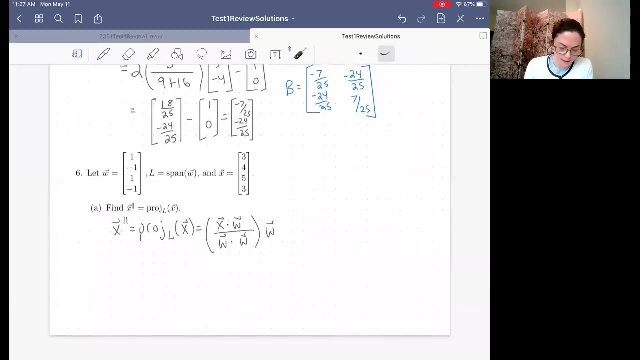 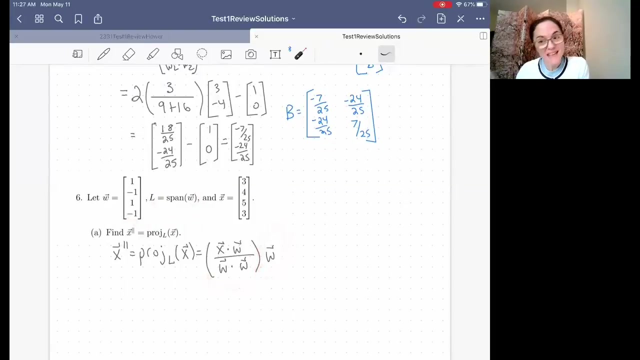 We take XW over WW and then times W. So you see, It is the projection onto a line. if the line is all multiples of this vector W, Well, look, I'm creating a multiple of W And the multiple is: well, you take this original vector XW over WW. 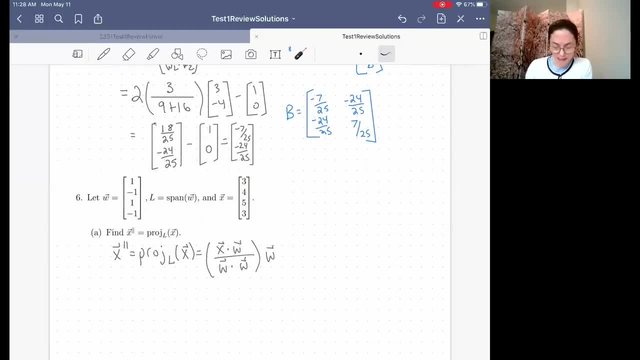 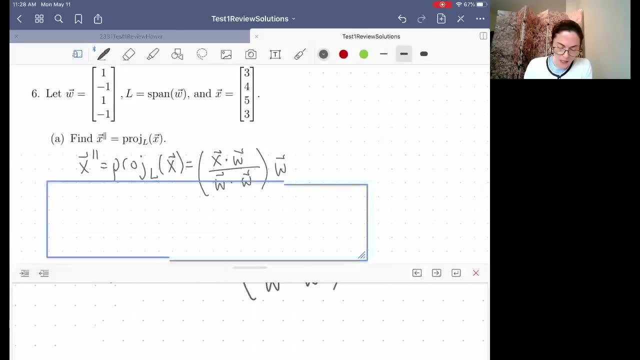 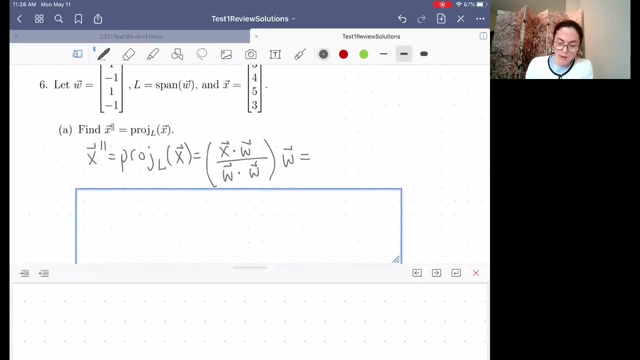 And this simplifies some- if W was unit. But I will just do it this way: W is not unit And this formula works just fine. Okay, So maybe I will go here What is? maybe I will come down here and do the side work in another color. 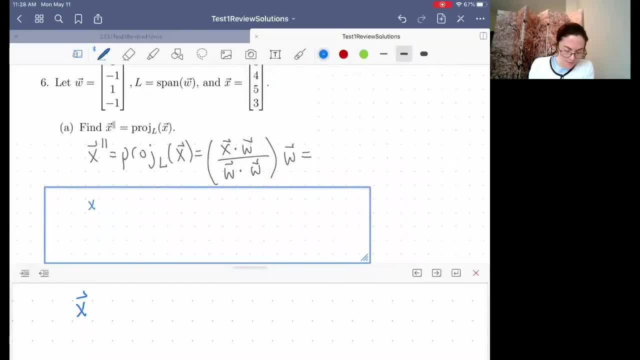 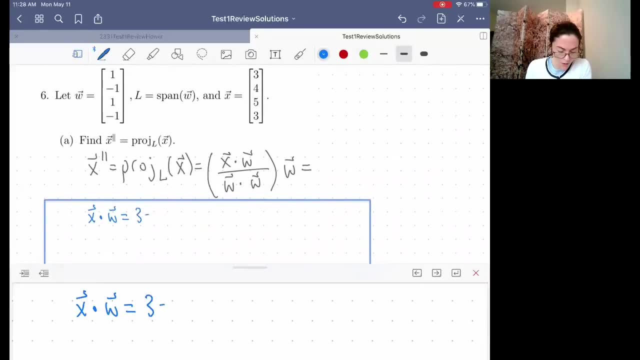 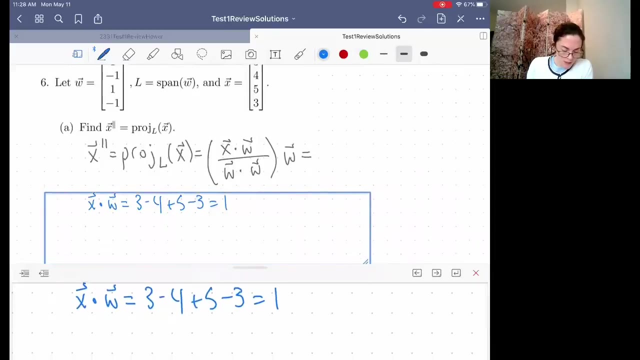 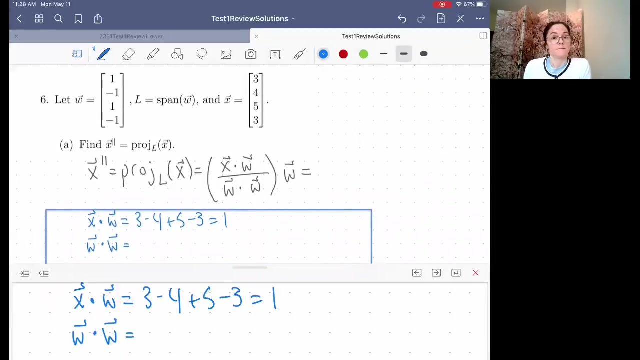 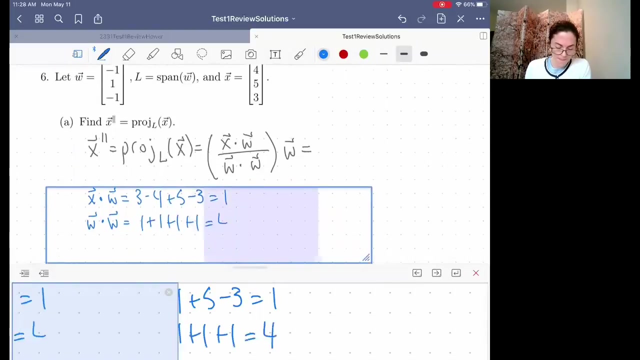 So what is XW? Okay, We can see our vectors. Well, it's 3 minus 4 plus 5 minus 3, which is 1.. And then WW is just, you look, It's 1 plus 1 plus 1 plus 1,, which is 4.. 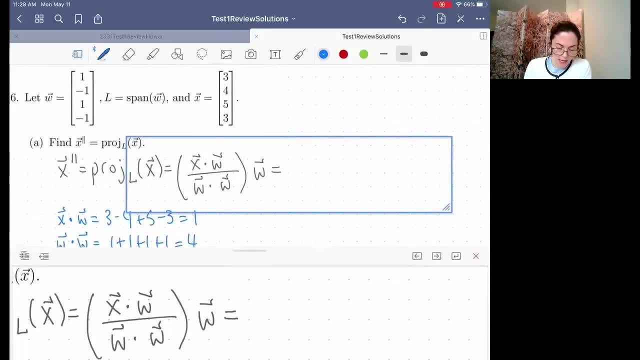 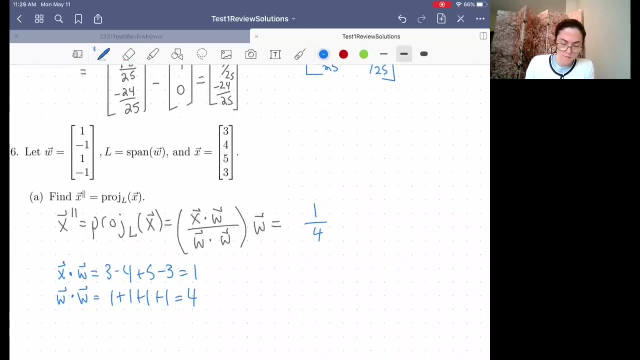 Okay, Great. So here we go. This projection is going to be 1 over 4.. Oh, I don't need quite that much Times this vector W, which is 1 minus 1, 1 minus 1.. And we can write that: 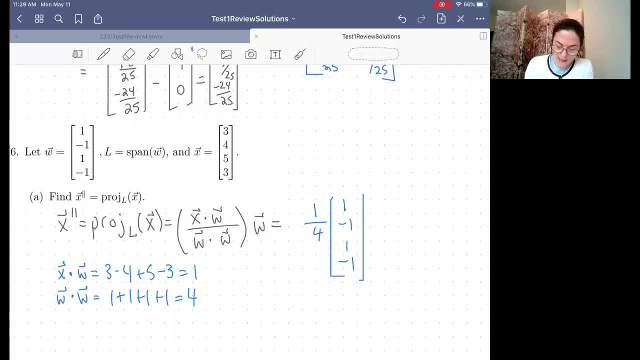 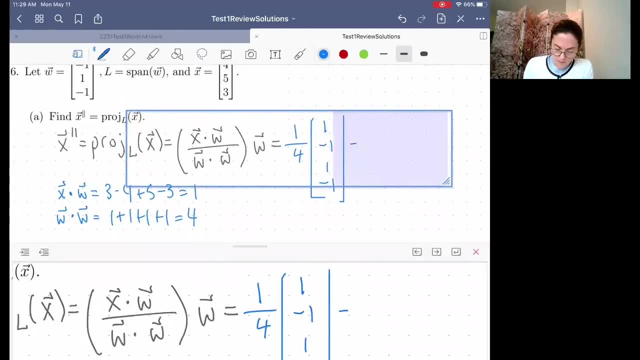 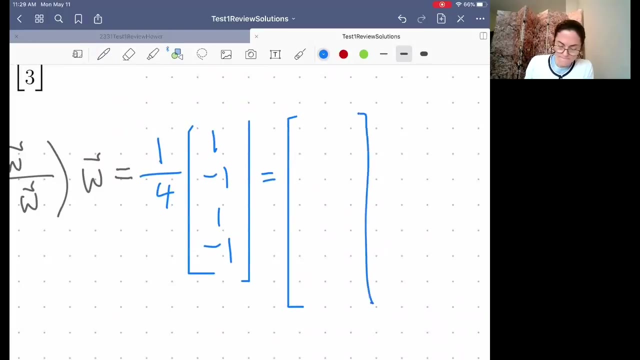 Well, you can just bring the 4th and the 1 over 4 inside. Let's move this over. Maybe I will. This is One fourth minus one fourth. one fourth minus one fourth. And now let's copy this: 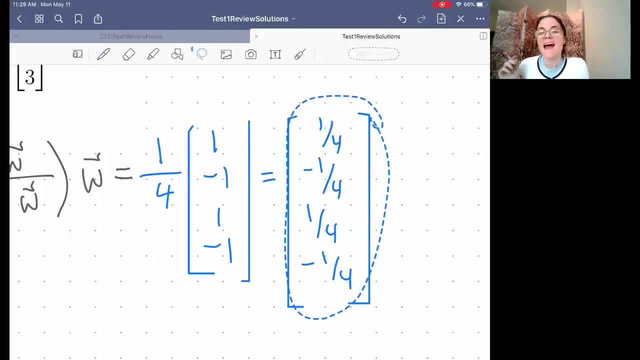 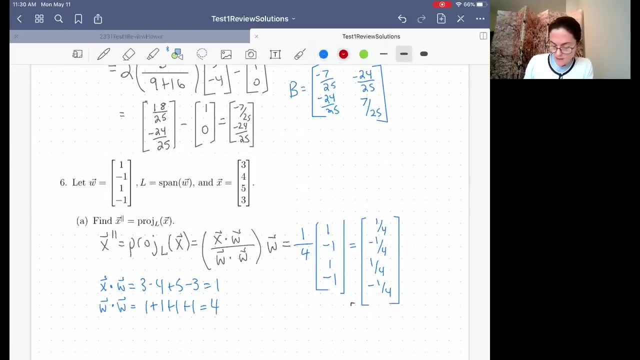 And we will move to the next page Copy And we will do the rest of problem 6.. So this was just to be clear. this is A. Okay, Now we're going to move here. Look, We have B. We have C. 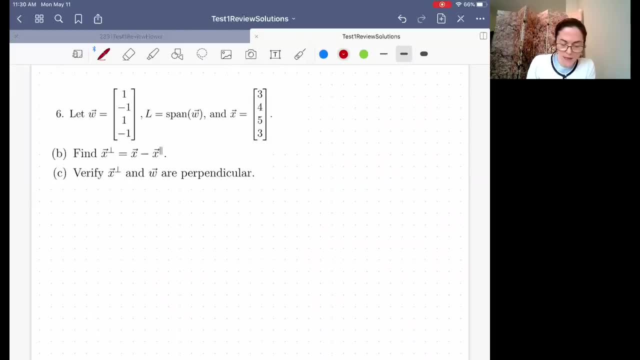 So the first thing is: let me just recopy what we have found. So we found that this, which is the projection, is here. Okay, So now let us begin. part B. This is part B. This is the component of X. 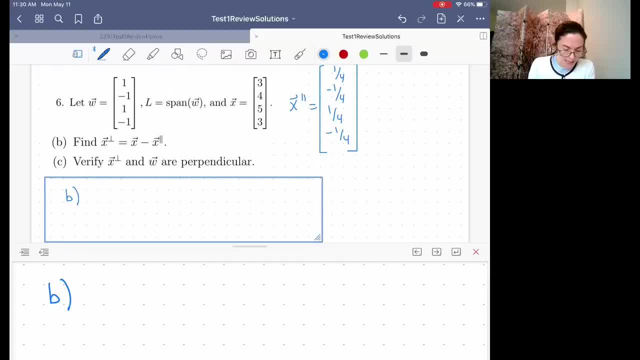 That is orthogonal to the line. That's what this notation is, And it's X. Let me write X, Which is 3, 4, 5, 3.. 3, 4, 5, 3.. And then minus. 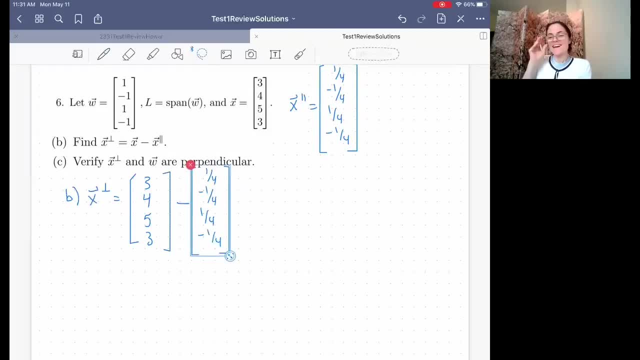 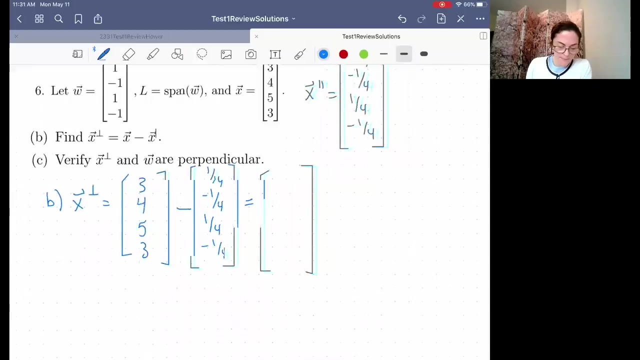 Let's see if I still have it saved. Oh, okay, Great, Minus this projection. Okay. So let's see what we get when we take this vector difference. Let me make a little Okay, Well, okay, This is fractions. 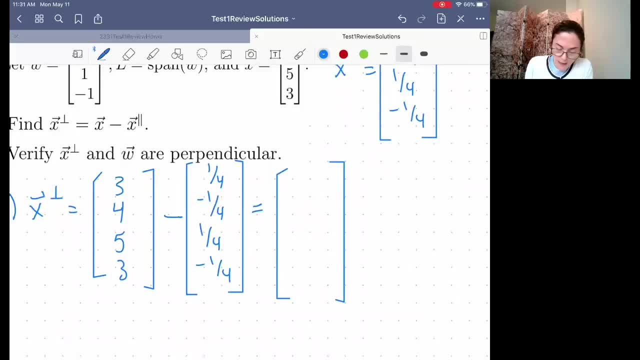 But it's okay: 12 over 4.. This is going to be 11 over 4.. And then this is going to be 17 over 4.. And then this is going to be 19 over 4.. And the last one is 13 over 4.. 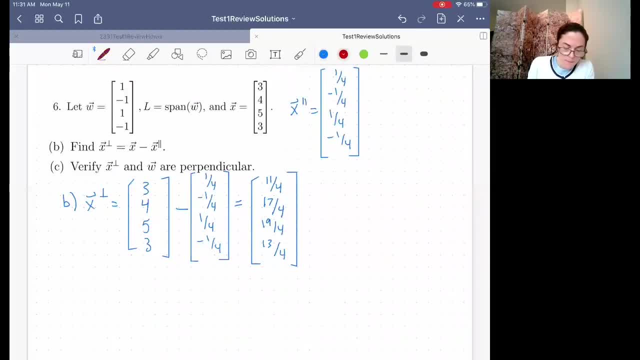 Okay Now. so let me do this. This should be at least if we number one did the problem right, And number two if we understand the theory. This should be perpendicular to the whole line And, in particular, perpendicular to W. 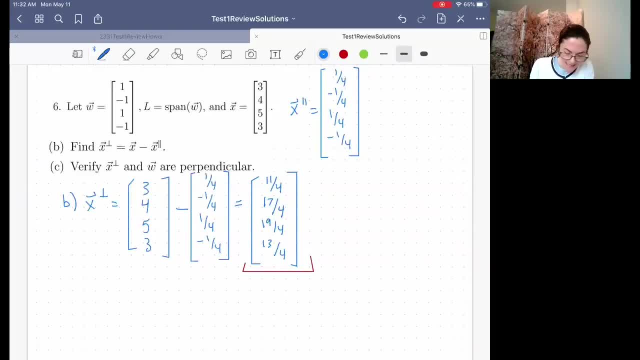 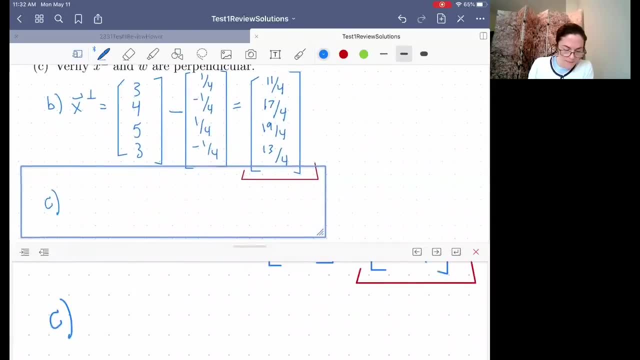 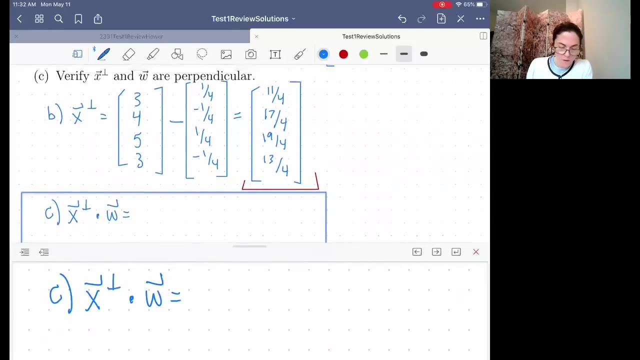 Okay, So let's do that now. That's what part C is asking us about. So part C Here What we want, Verify. We want to take this Dot W, And I need to be able to see them all. 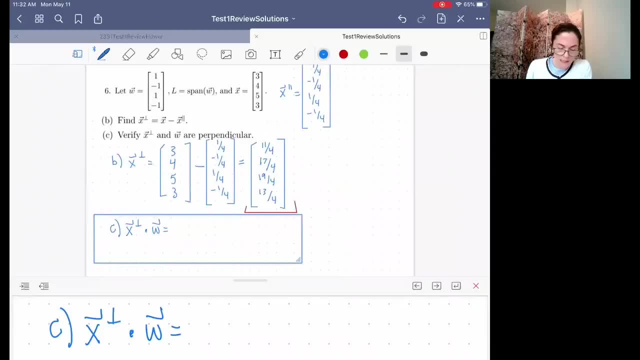 Maybe I'll just move this down. Okay, Here we go. This is If I take the dot product of these two vectors, you see I get 11 over 4.. I get minus 17 over 4.. Plus, I get 19 over 4.. 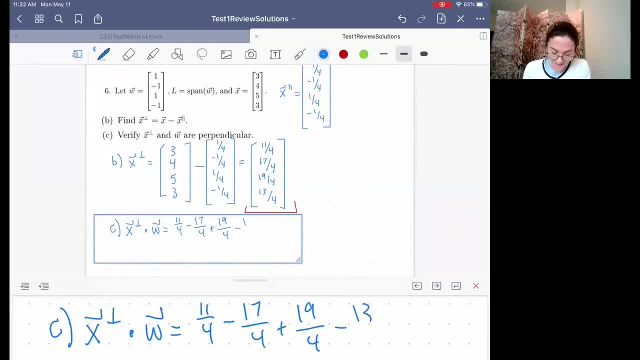 Minus 13 over 4.. Okay, So all together, how many pluses do I have? 19 and 10.. 30 over 4.. And then how many minuses do I have? 17 and 13.. Oh, okay. 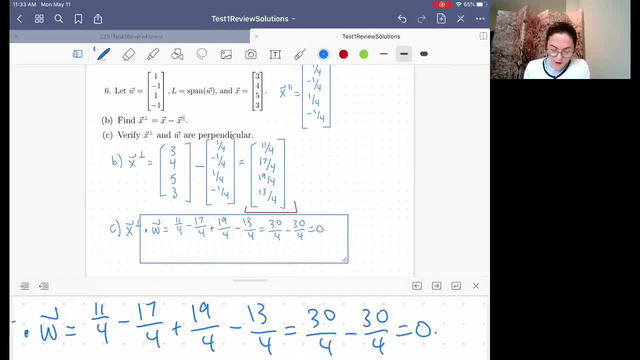 This is going to work: 30 over 4.. In fact, 0. And so this shows that this component of X that's perpendicular- Yeah Okay, Orthogonal to the line or perpendicular to the line that we found in B, is in fact perpendicular. 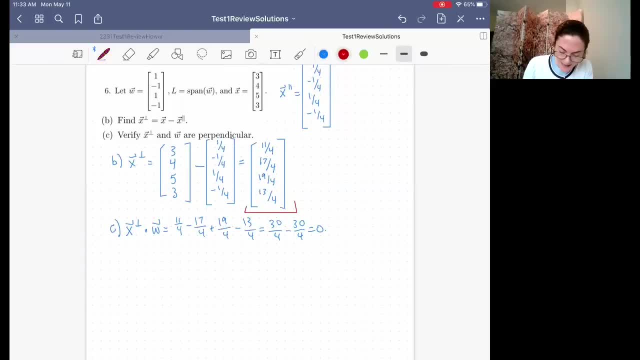 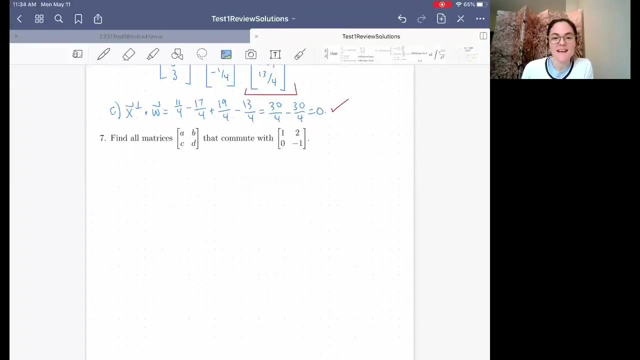 to W, Which is it should be. That's what we created. Okay, This is great. So we have completed number six. Now number seven: Find all matrices that commute with this particular one. Okay, We had several like this in the homework. 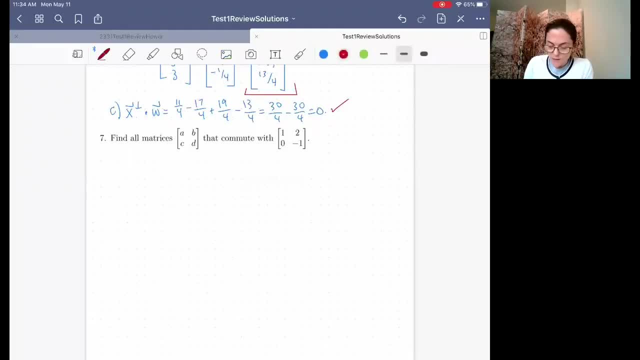 But this is a good exercise, And so let's do this one now. Commuting means the following: So what we want, maybe I'll write over here. We want- let me label some things: If this is capital A and this is capital B, two matrices commute. 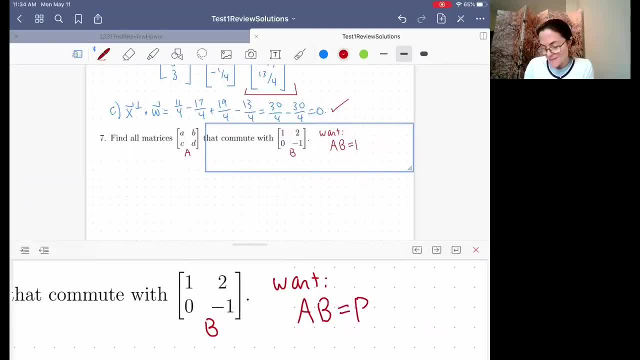 What it means is that AB equals BA. Okay, Well, this only happens when the matrices are square And of the same size. It's the only possible way it can happen, And we see that here. So that's going to allow us to solve for A, B, C and D. 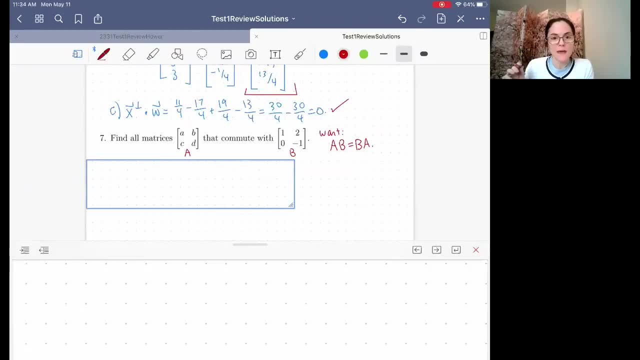 So what I'm going to do is multiply in each direction and then set them equal. We know two matrices are equal, provided well, their corresponding IJ entries are all equal. So I'm going to have four equations that come out of this. 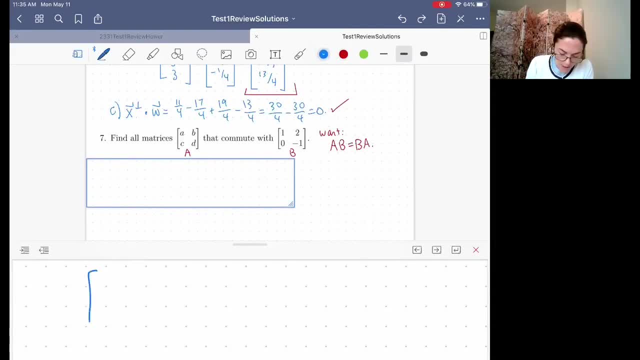 But the first thing I'm going to do- Oh, I don't want to be in red- The first thing I'm going to do is just multiply in each direction And then I have one two zero minus one. After I made this problem for the review, I realized I think one two zero one. that matrix is one that's in the homework. 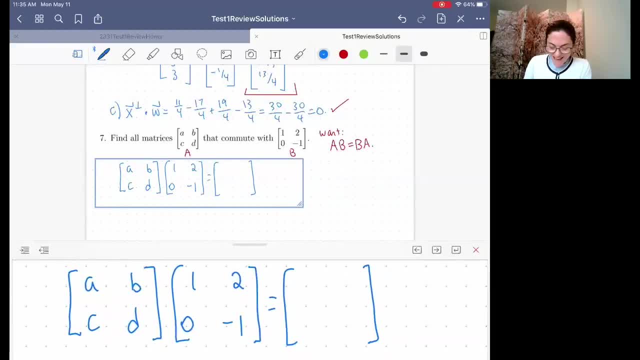 But we wound up getting a different answer. here It's a different matrix. Okay, Here we go. So when I multiply- oh, maybe I need a little more space- I'll just multiply and then I'll figure it out- I get A. 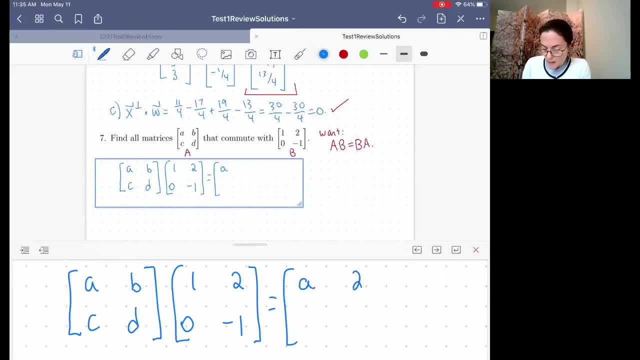 I get 2A minus B, I get C, And then I get 2C minus D. This is multiplying in this direction, And now maybe I can just copy and paste. Let's take this one, Put it here. Oh great. 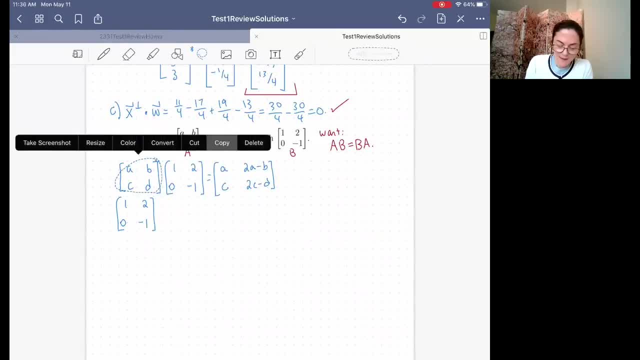 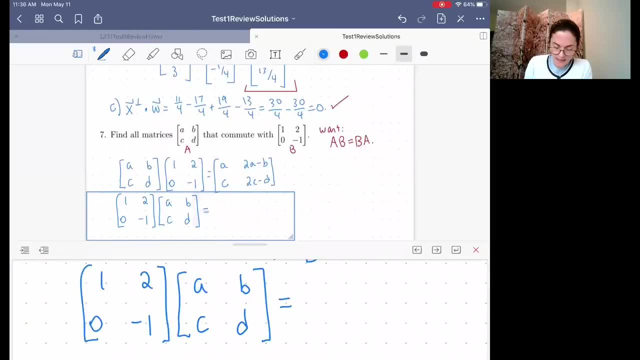 And then take this one Copy, Put it here: Okay, Equals. Now let's do the matrix multiplication in this direction, And then I will set the two results equal. So in this direction, I get A plus 2C. I get B plus 2D. 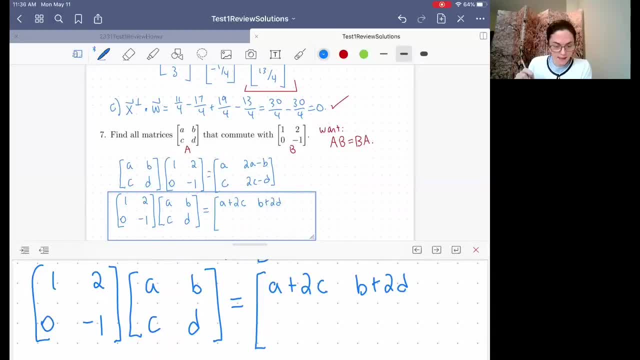 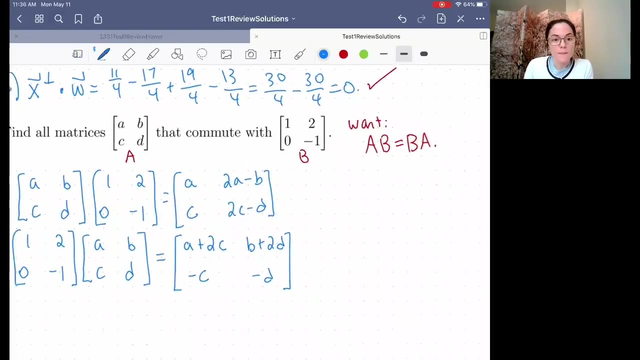 And then for the bottom second row, I get minus C And I get minus D. Okay, Looks good so far. Now let me zoom in some, because as long as we can see what we're working on and we can, Okay. 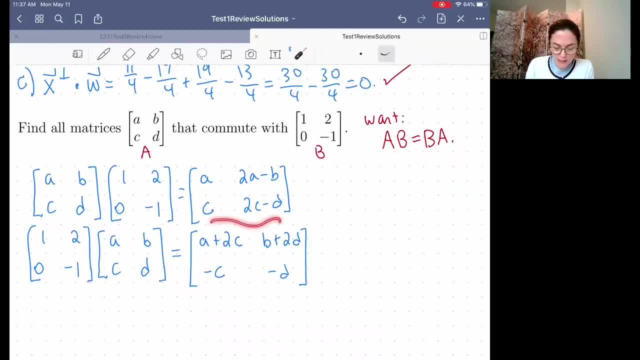 So, as I was saying, for this matrix to be equal to this matrix, we must have: this is equal to this. We must have this is equal to this. Similarly, this one is this one And this one is this one, Like this. 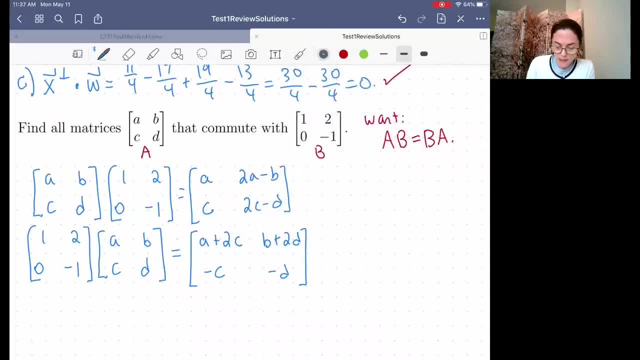 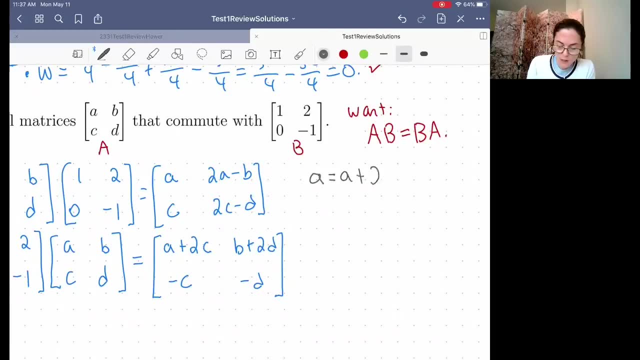 Okay, So what are the four equations that we get? Maybe I'll do it in a different color. We get that A equals A plus 2C. We get that C is negative C. We get that 2A minus B Is B plus 2D. 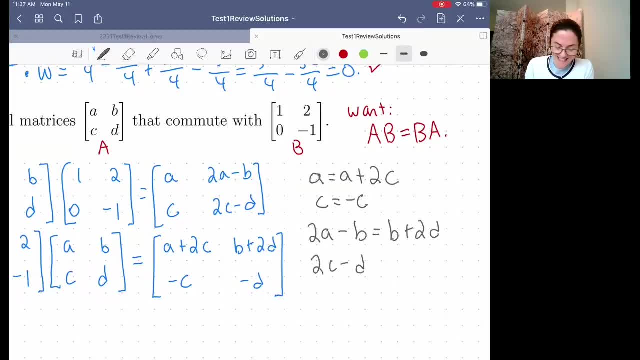 And we get that 2C minus D is minus D. Right, Okay, Now, immediately, we can conclude. well, three of the equations are saying the exact same thing. Maybe I'll underline them in green: This equation, this equation and this equation all say the exact same thing. 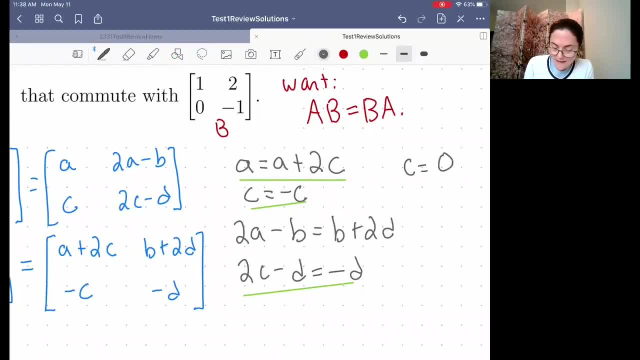 And, moreover, that A and D can be anything. So so far C is zero. And then, for instance here: A can be anything and D can be anything. Okay, So the only thing left to do is figure out what B must be. 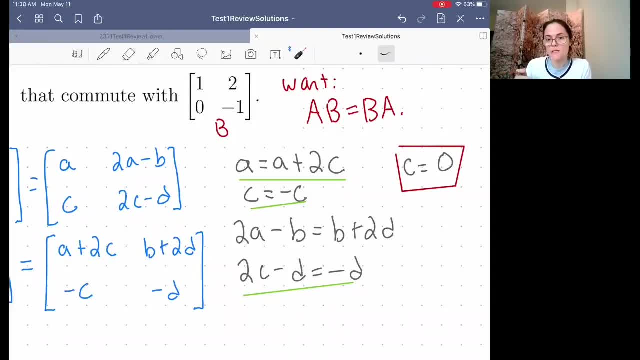 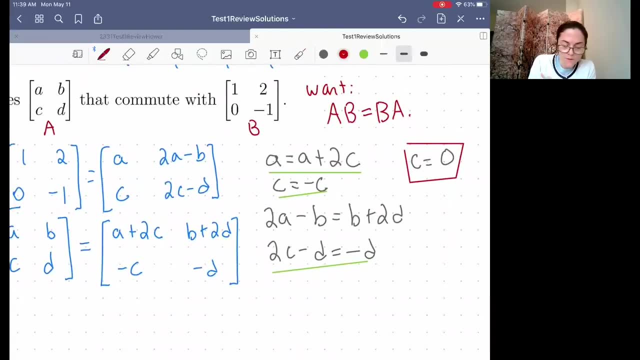 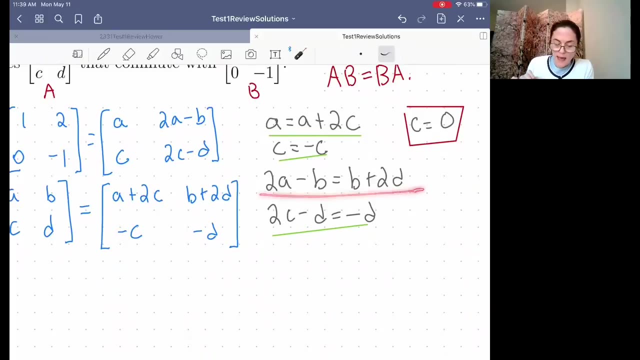 Because A and D from the three equations we have. Okay, So the only three equations we have can be can be any real numbers. So let's move to this third equation here, This one, And I need to figure out what B must be. 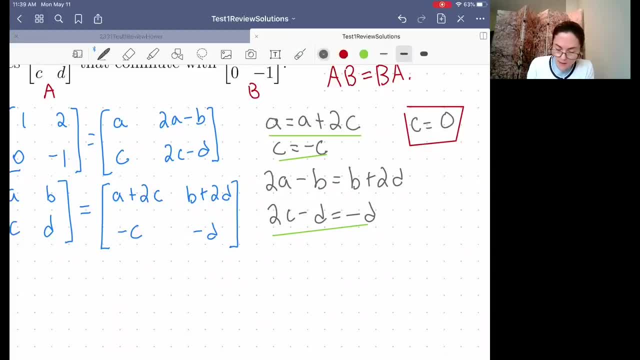 Okay. So what I'm going to do is just solve for B. Okay, So I'm going to bring everything with B on one side. I'll do it here. 2B- I'll do everything without the B. I move to the other side, which will be 2A minus 2D. 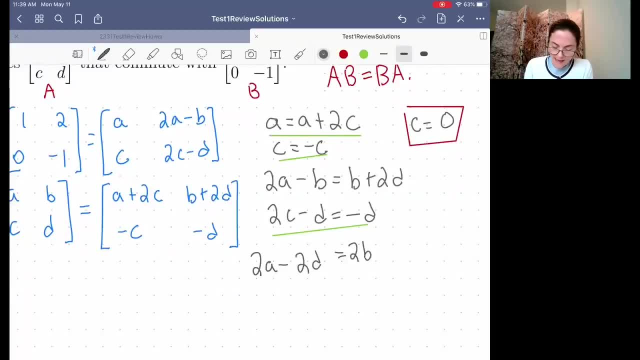 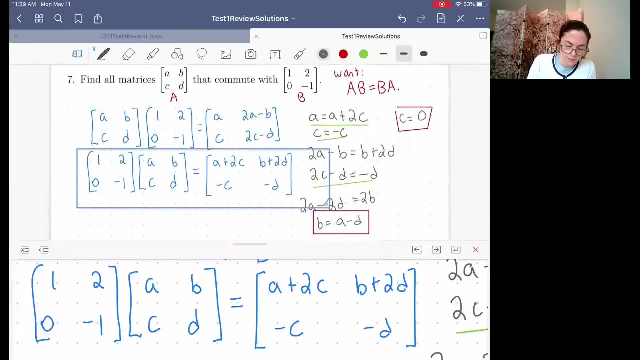 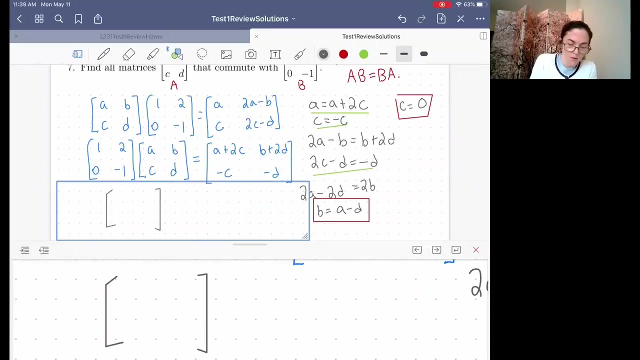 2A minus 2D And now divide everything by 2.. I get B is A minus D. Okay, So now we know what this matrix must look like. So the answer here. I'll do it in gray, Okay. 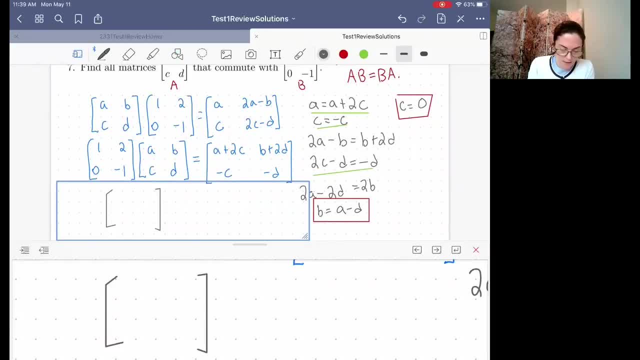 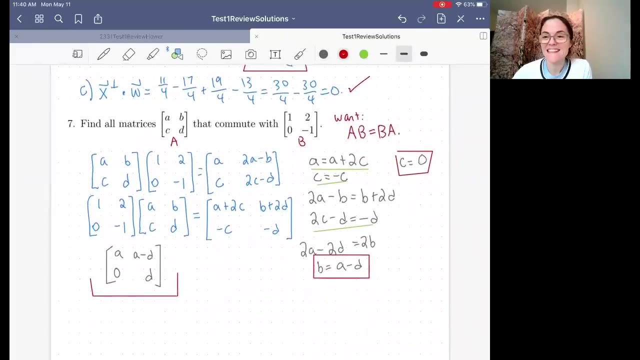 The answer is: what did I say? A and D can be anything. A and D can be anything. Z is zero, And then B is A minus D Here. Okay, Number seven. That was fun. Now for number eight. 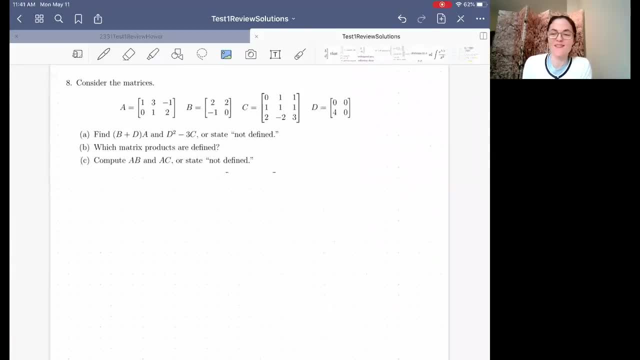 So I moved to the next page, so I really didn't have enough space for this problem On the page I was on. Okay, Great. Now, in order to answer a lot of these questions, we have to think about the sizes. So let me do that. 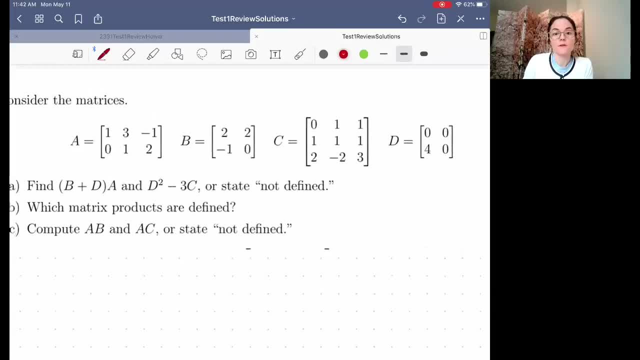 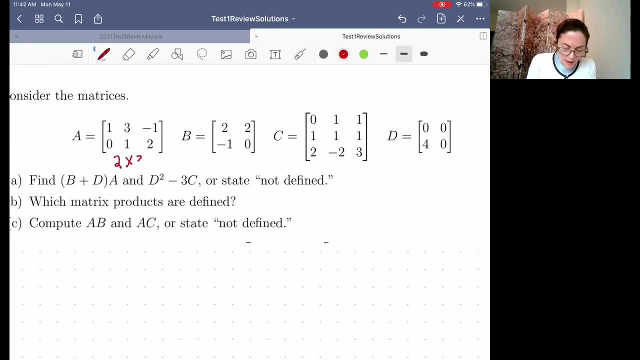 I'll zoom in and we're going to do that first. Okay, A is two rows by three columns. B is two rows by two columns. C is three rows- Oh, let me make that nicer to read: Three rows by three columns. 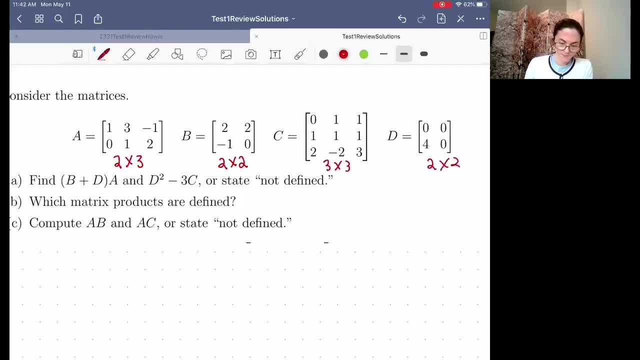 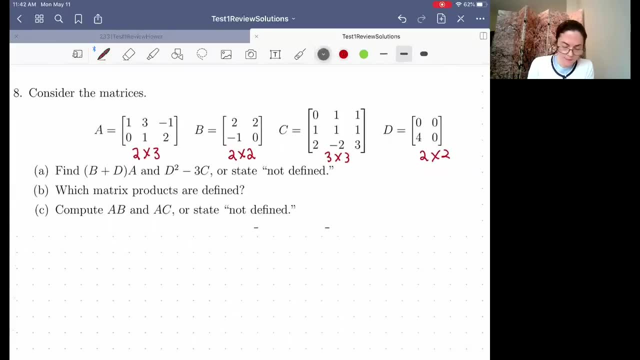 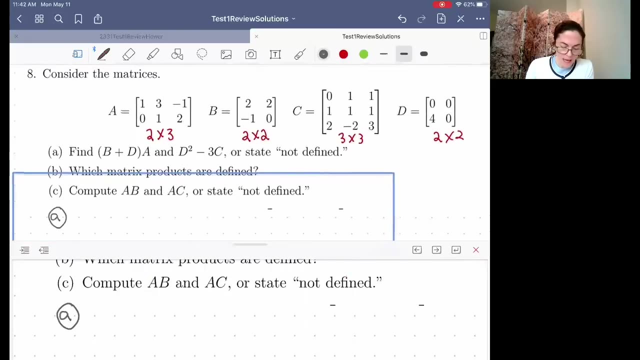 And D is two rows by two columns. Okay. So what can we do? Let's look at A and figure out what of these operations we can do. A is B plus D. That's okay, We can do that. They're both the same size. 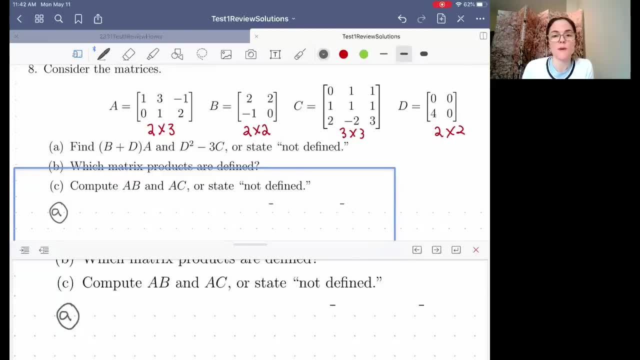 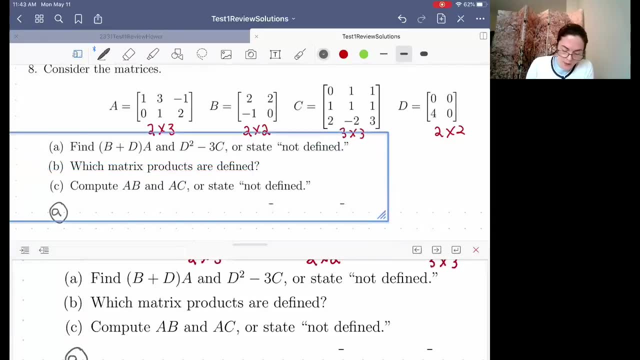 You can add two matrices, Provided they're the same size. we can add B plus D And then we multiply, So we're going to be able to do this Why? So? let me write underneath. Oh well, maybe I'll just zoom in here. 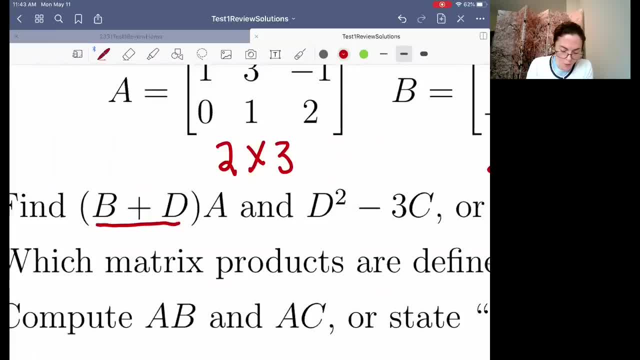 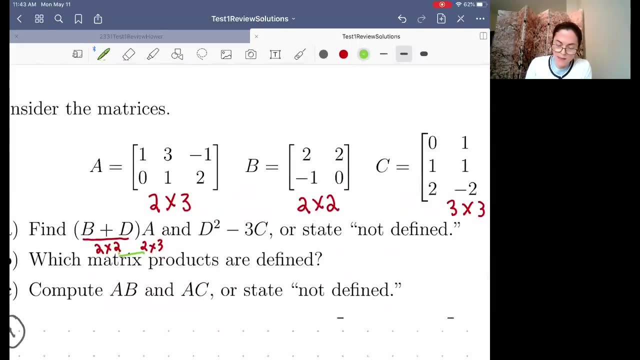 B plus D. once we add this will be two by two. A is two by three And you see, these two match, So we can make this product. Let's do the same over here. just thinking about size, D is two by two. 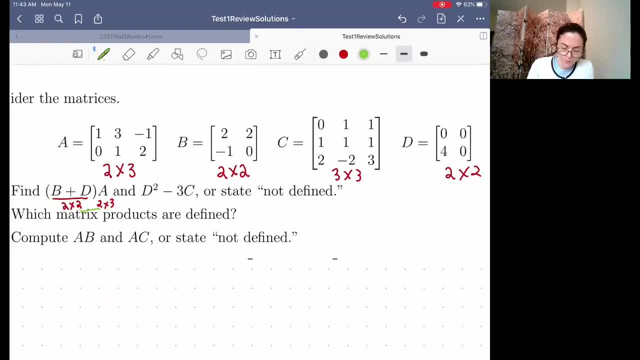 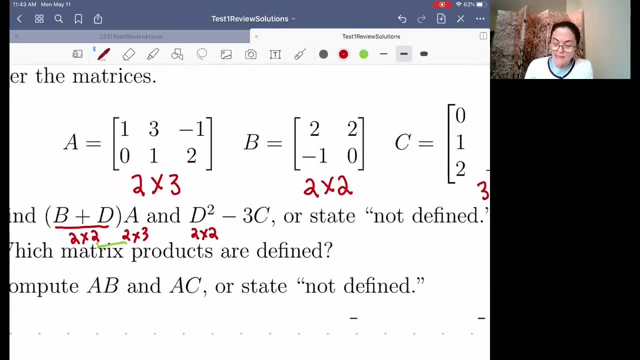 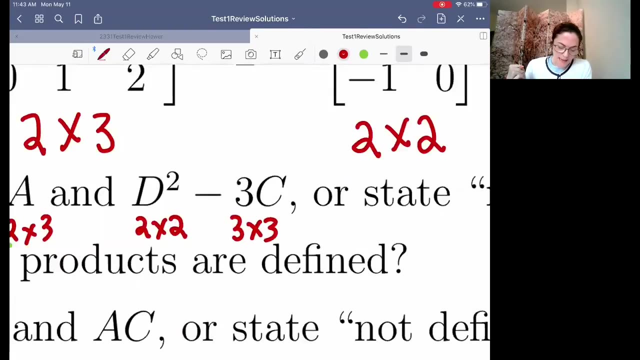 You can certainly take D squared. It will be two by two. So this will be two by two. C is three by three. Multiply C by a constant: It will still be three by three. So this will be three by three. Now you cannot subtract or add. 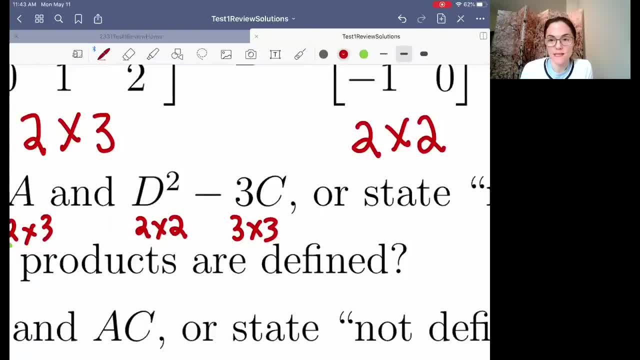 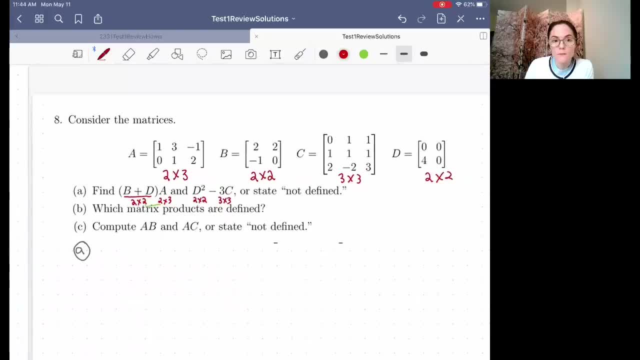 Matrices that one is a two by two and one is a three by three. You can't. They have to be the same size, So this one maybe. I will start with that observation. Okay, I'm sorry if I'm making you dizzy. 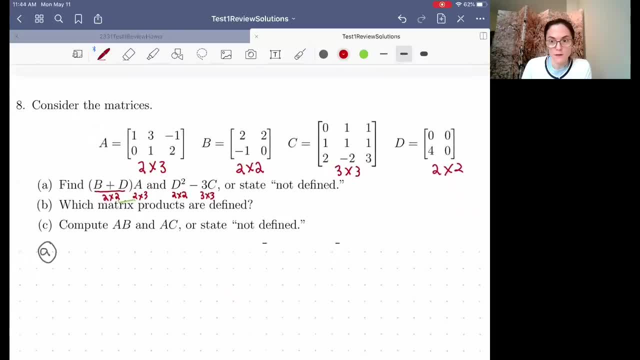 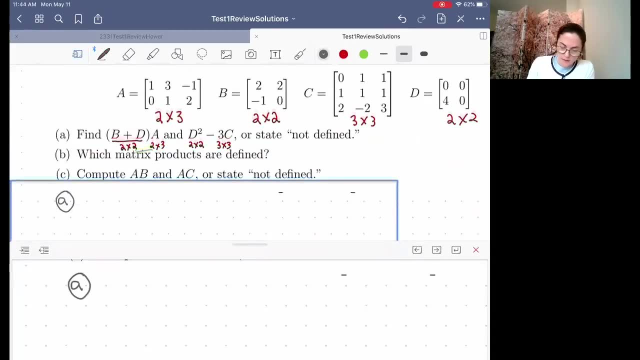 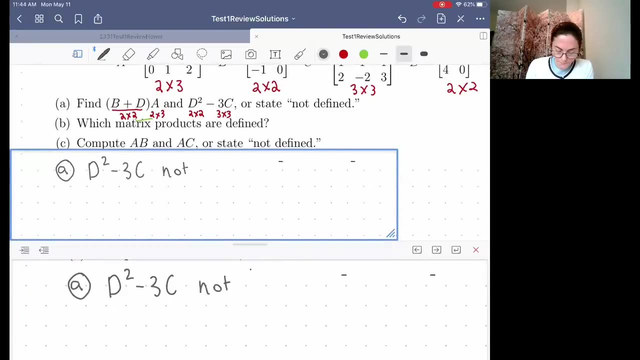 I'm trying to get the right view. Okay, let's start with the observation that this one D squared minus three C, not defined, But the other one is B plus D times A. like this, This will be two by three. Okay, so first let's do this. 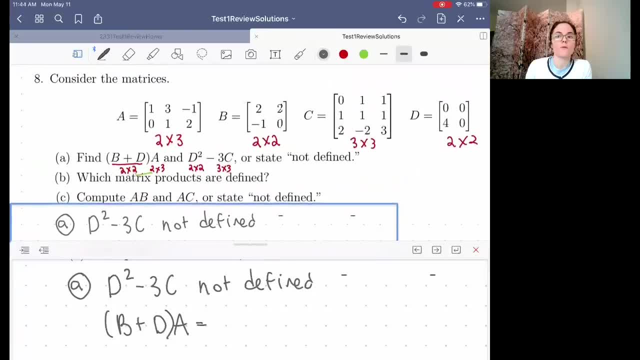 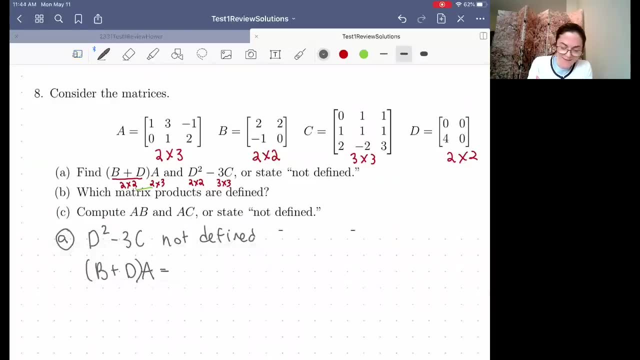 I need to see my matrices, though. Okay, let's B plus D. Oh, let's see, Maybe I'm going to have to X that and then write like this. Let us write: I'm going to have a two by two. 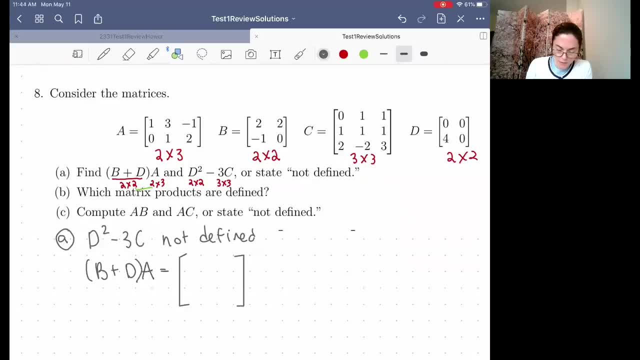 And then I'm going to have a two by three. I'll go ahead and copy: A: A is one three minus one zero one two. And when I add B plus D, well, I get two two zero three. Now I need to multiply. 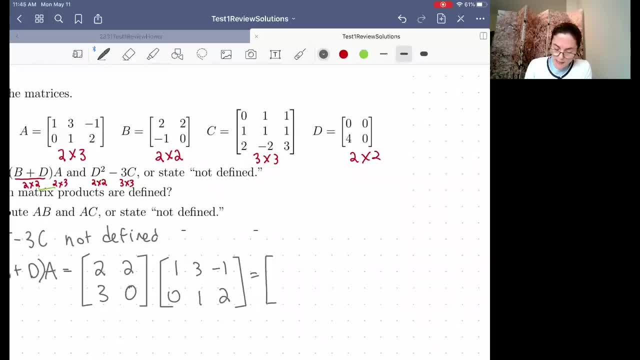 And this will be, as I said, two by three. Okay, well, let's think about this: We get two, We have six plus two, And we have minus two plus four, And then we have three, Then we have nine. 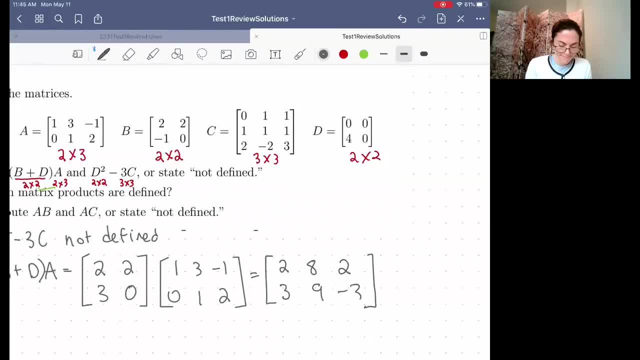 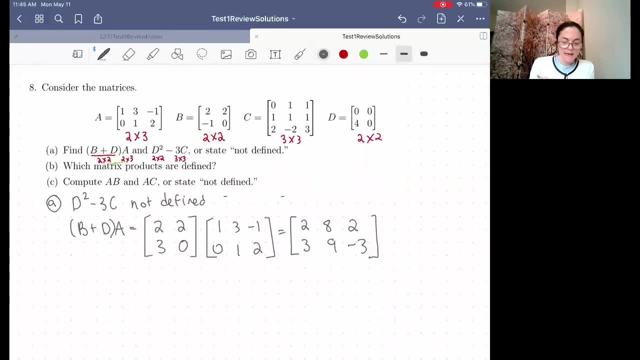 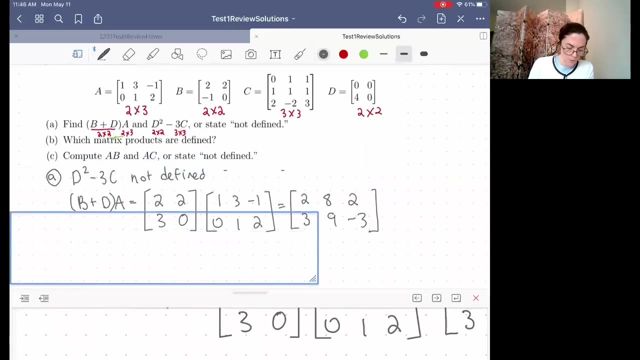 And then we have minus three. Okay, Okay, great. So now we have done part A, Now part B. we're not having to compute anything. We just have to think about all possible products which are defined, And we have to think about the order of them too. 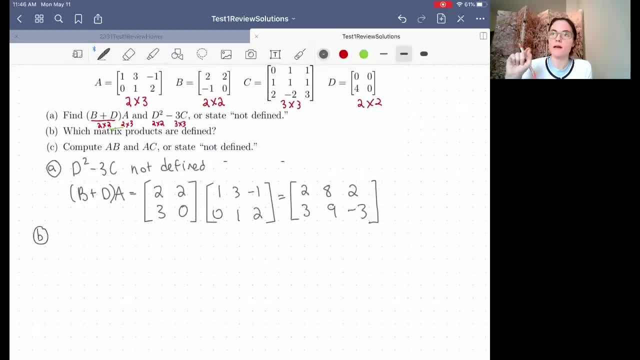 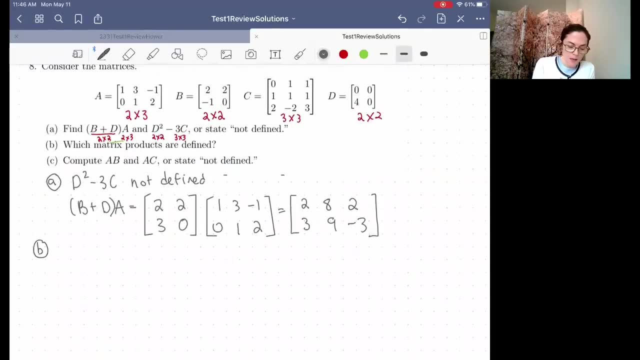 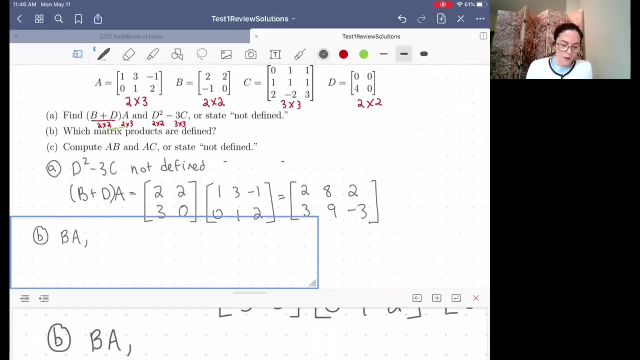 because just because you can multiply two matrices in one direction doesn't mean you can multiply in the other direction, For example: Okay, so what's the first one that we see that is defined? BA is defined, But A times B is not. 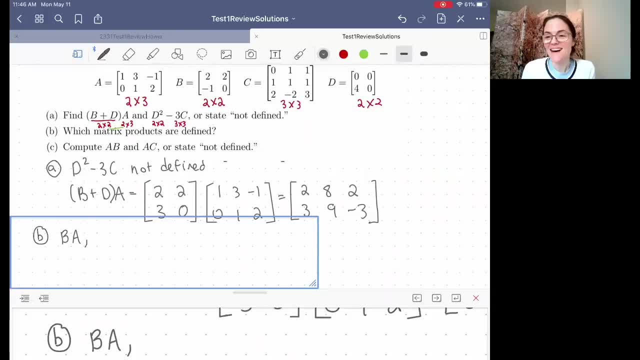 In fact that is part of C, although I'll get there when I get there, Because if you look at the dimensions A times B, we have two by three, two by two. The middle ones don't match, But we do have. AC is defined. 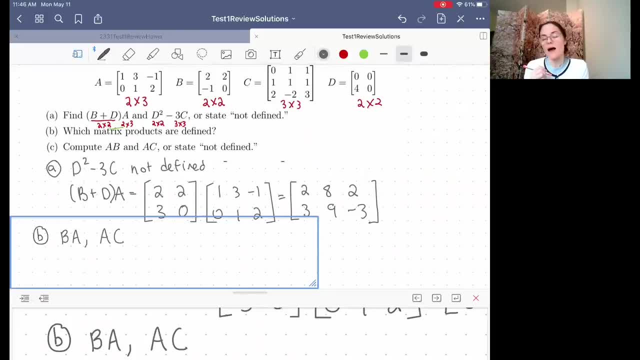 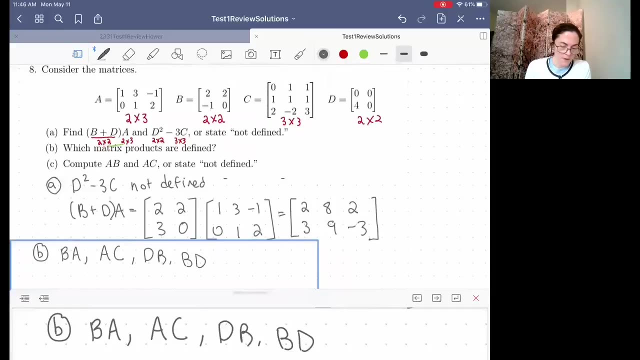 This is fine, The middle ones will match, But CA is not, For example. Okay, And then what else? Well, DB is defined, BD is defined, BA was defined. That means DA also. they're the same size, but not AD. 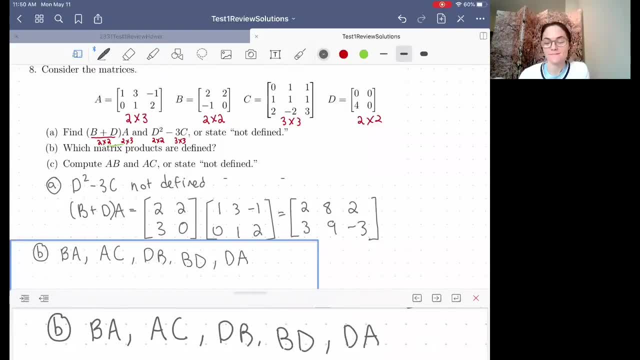 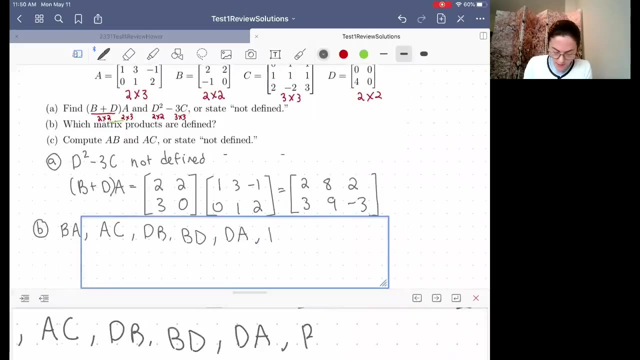 So am I missing anything here? Ah, yes, okay, I'm missing. Here's the only thing I'm missing: The squares. Okay, good, So we have also. we can do B squared, We can do C squared. 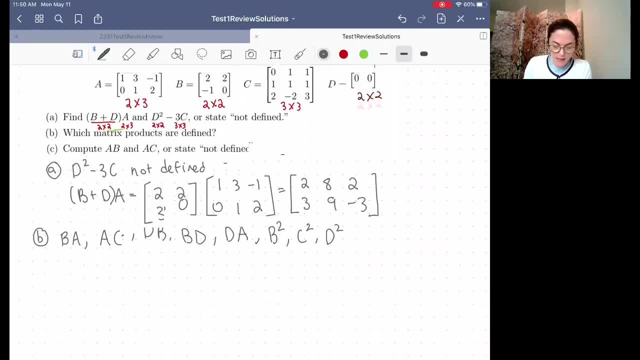 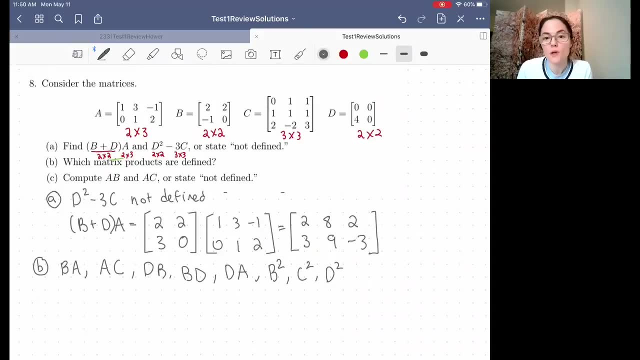 And we can do D squared. That would be taking B times B And C times C And D times D, So I was missing multiplying a matrix to itself. Now you cannot make A squared, For example, because it's not squared. 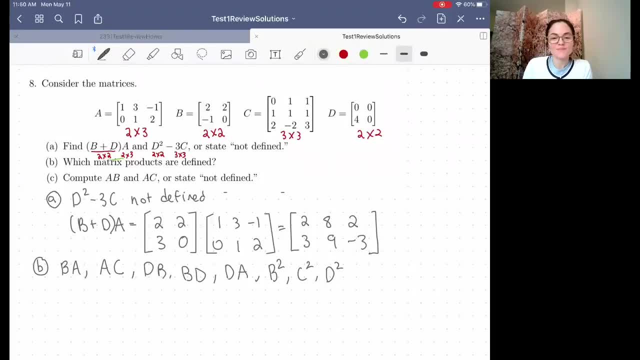 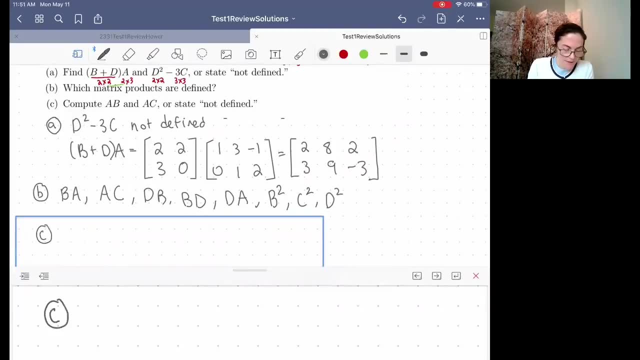 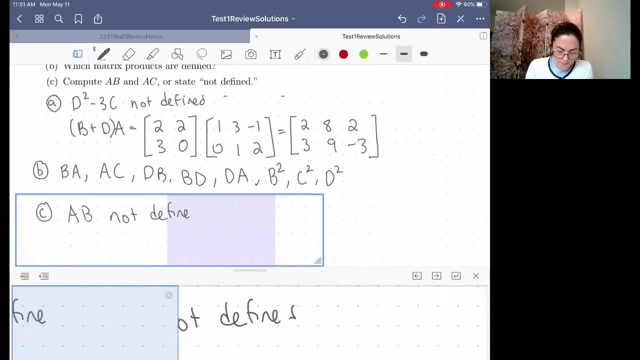 You can't multiply A times A. It doesn't work out like that. So these are the ones that are defined. Well, I already mentioned- In fact we already know- AB not defined. Okay, The sizes don't work out. So now what we need to do is just compute A. 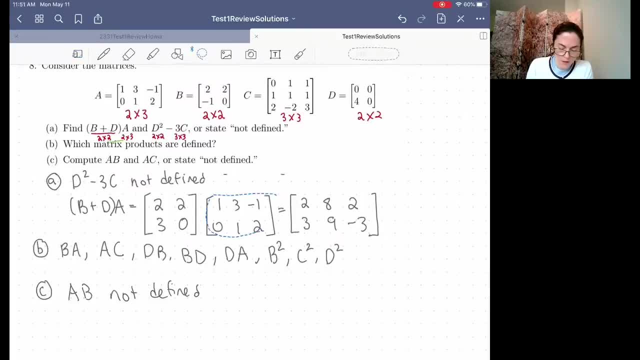 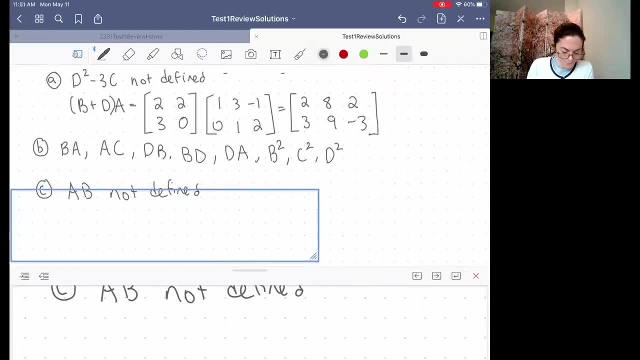 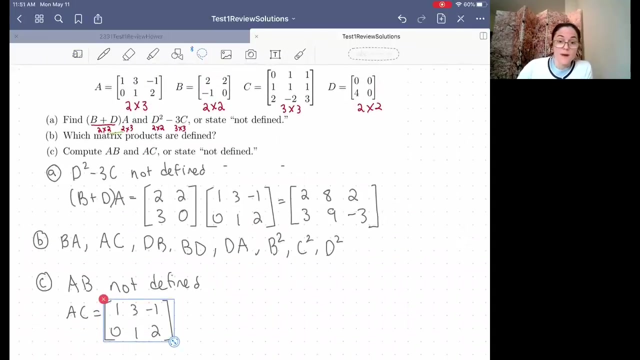 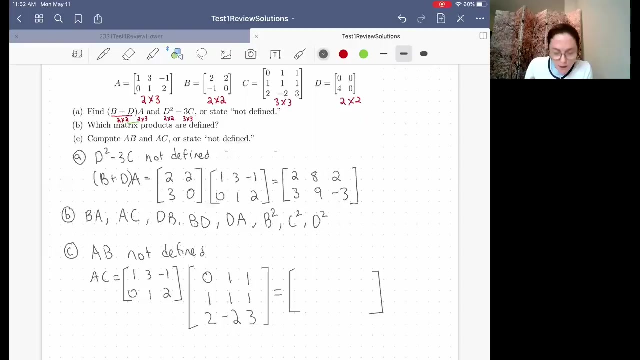 which I've already written. So I will copy this AC. Here's A And then C, Three by three. Okay, Here we have A times C at least written. Let's make sure I copied everything, right, Okay, good. 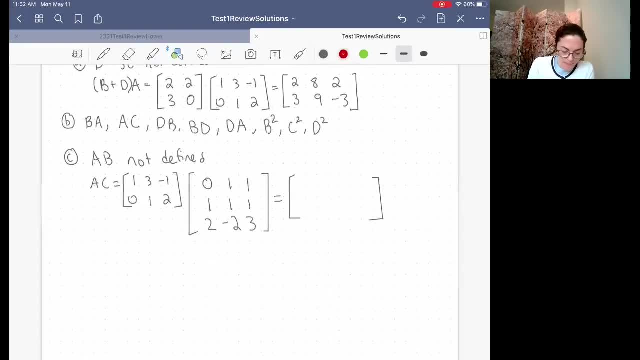 And then, if you think about sizes here, as I was, as I've been doing this whole problem, A has two rows. Oh, sorry about that. Two rows, three columns, Three rows, three columns. This will have two rows and three columns. 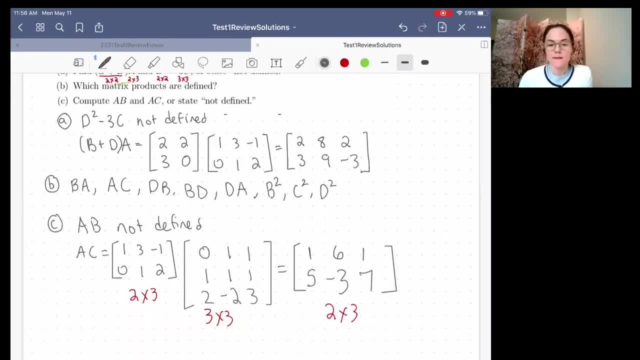 So let's do this here. So here I have written A times C, But let's talk about it because I didn't show the steps in the video. So what did I do? So what did I do? I took this row, dotted this first entry. 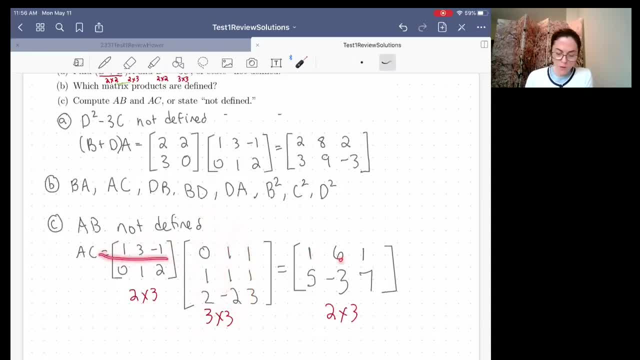 Row dot column. second entry: Row dot column. third entry Right. This is how we multiply two matrices And then I move down. this row dot column is the five Row dot column minus three. 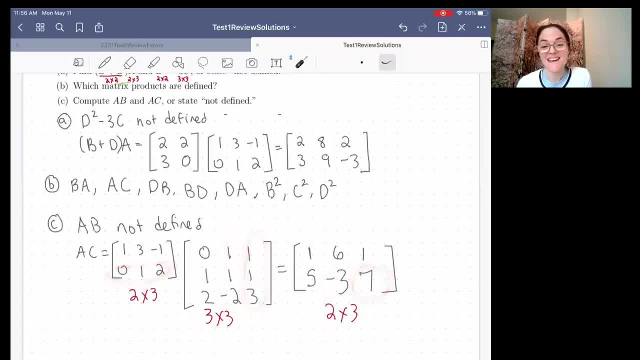 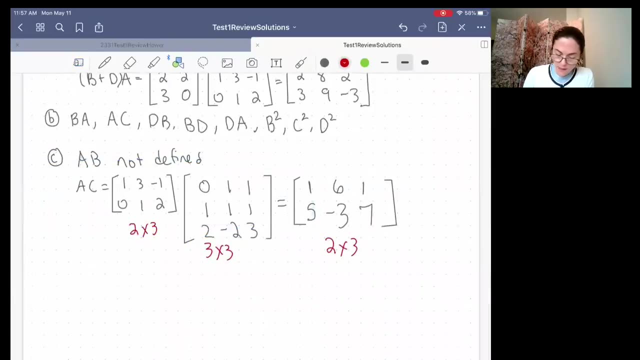 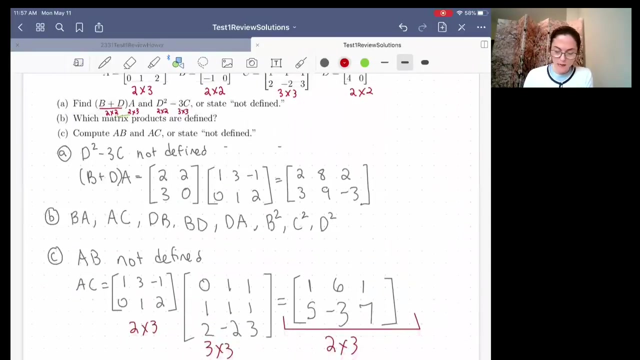 Row dot, column positive seven. And this is how we compute the matrix product. And so here is the final answer in C: Oh, maybe I don't need that. Is this matrix here? Okay, A times C. And then, as we discussed, AB is not defined. 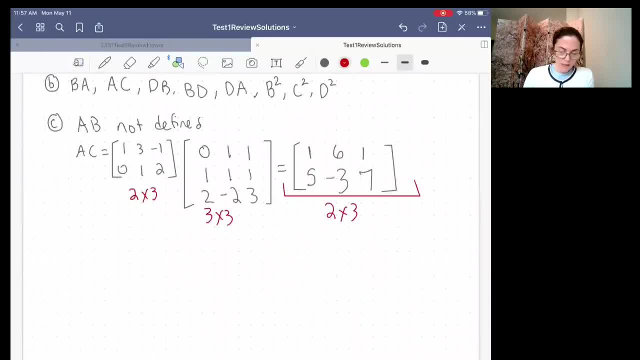 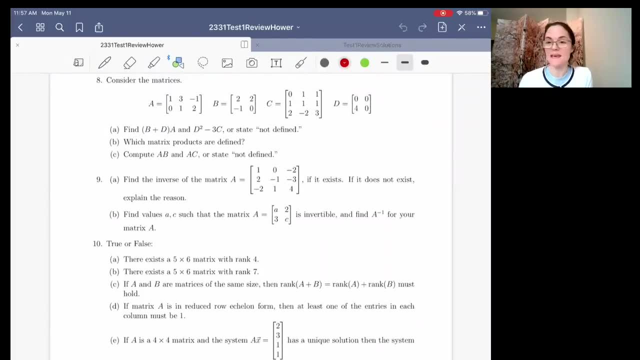 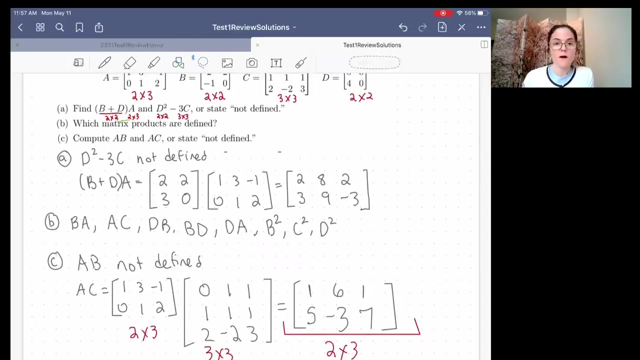 Now let's see what I have left. Oh, so we have nine. We have to find the inverse of two matrices, And then we have the true, false questions. Let me maybe reduce the size here And we will move on to number nine. 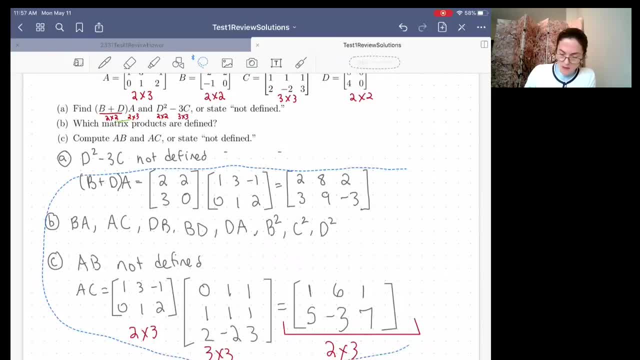 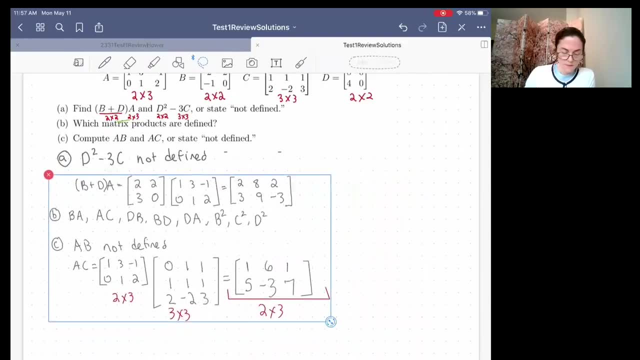 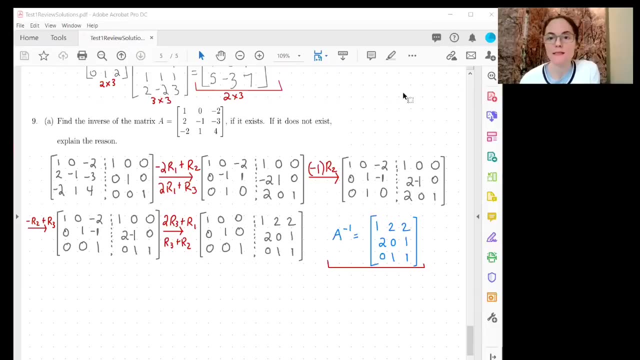 Give me some more space. Let's go over here. Let's go over 9A this way as well, in part because so much of well. just like number one and two, the operations in finding an inverse matrix involve elementary row operations. 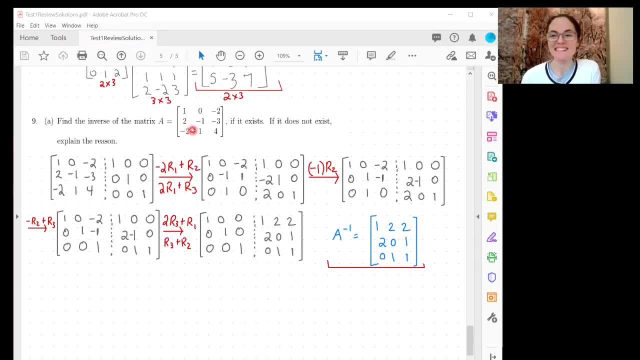 And so I have them written out and we will discuss. However. well, how do we find the inverse of a matrix? Okay, This is what's new. Well, it must be square. Okay, This is three by three, Then we form what you see here. 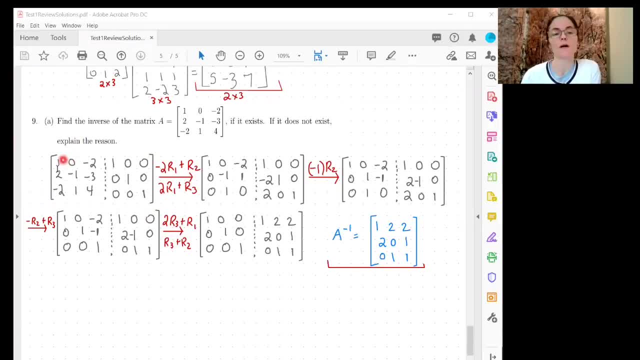 This is an augmented matrix where we put the matrix A and then, on the right, we put the N by N- identity, So this will be N by 2N. In this case it's three by six. Okay, Then you row reduce with everything that we practiced in 1, 1, 1, 2, 1, 3, like this: 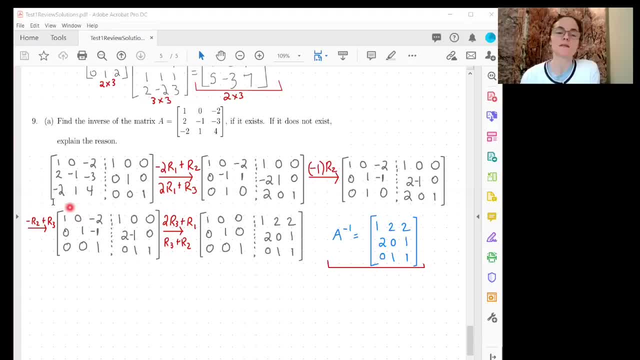 row operations, Let's say row operations, to transform this, this N by 2N matrix, into reduced row echelon form, And this is what you see here When you do this. well, if the matrix is invertible, namely a inverse exists, then your reduced 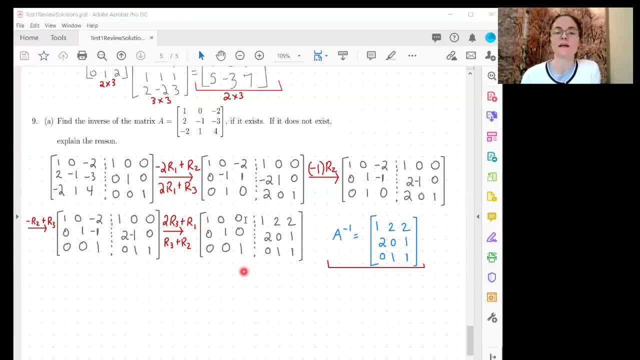 row echelon form will have on the left an N by N identity And on the right, this will be the inverse. Okay, And here if you read this, if it does not exist, explain the reason. Well, one reason you could give, let's say it didn't exist. 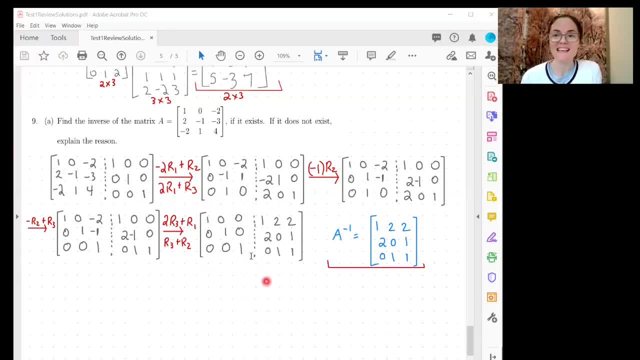 Here it does, You'll know through this process. So if I reduce this n by 2n augmented matrix and in reduced row echelon form here on the left it is not the identity. n by n identity, then you know the matrix is not invertible. 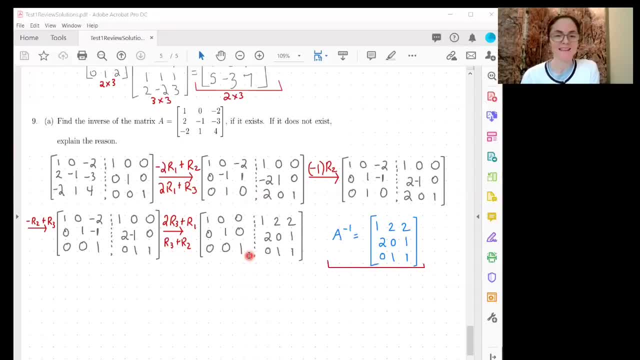 So if I had a row of zeros here, or something like this, yeah well, that would be the problem. If you don't get the identity on the left when you do this, your matrix is not invertible. So let's talk about these steps. 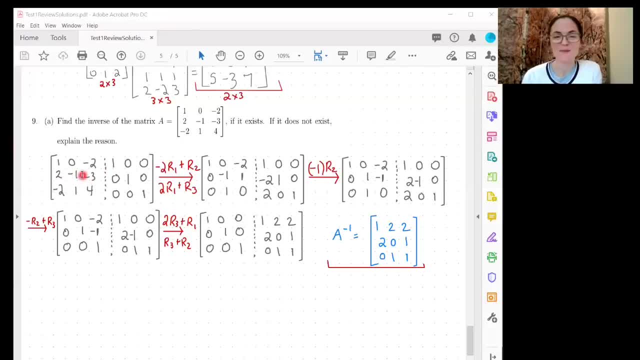 Okay, this kind of thing we have done many times, right, But doing it to find an inverse matrix is what's new. I want to put zeros Underneath this first leading one. I take minus 2 row 1, add it to row 2, 2 row 1, add it to row 3.. 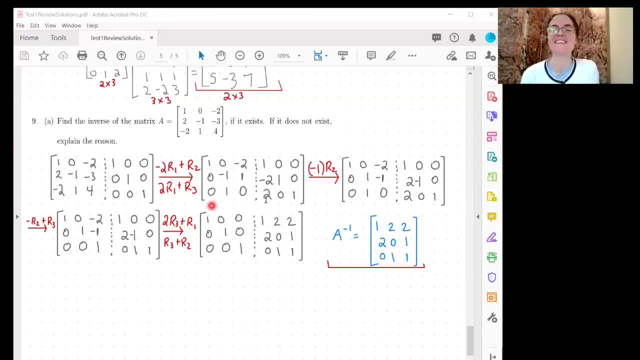 And ta-da, Here is what we get. This is the result, right here. Then I already see my second leading one will be in the 2, 2 position. I take minus 1 times row 2, and here it is. 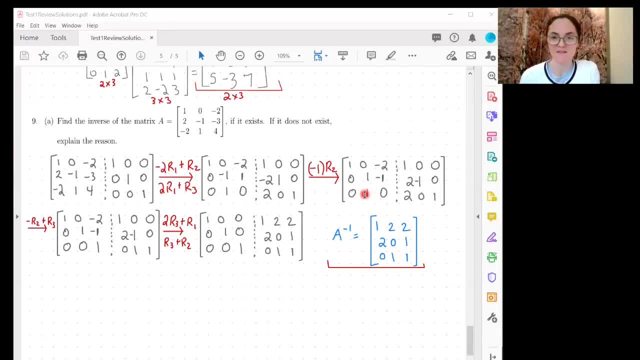 And then I would like to make this entry a 0. So I just take negative row 2, add it to row 3.. Ta-da Again. Now, if you look at this matrix, you will realize we are in row echelon form, because here: 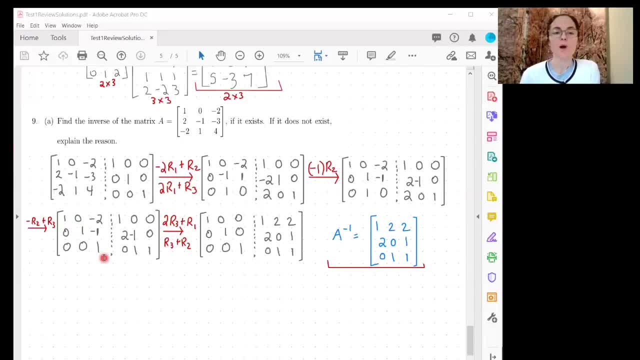 Right, But row echelon form really doesn't do anything for us when we're looking for a inverse, because we're not finished. So what I need to do, in fact this leading one is okay. I only have zeros in this column. 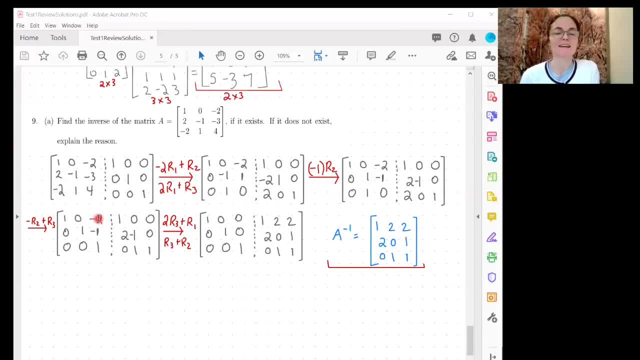 But I need to do this. But this entry here and this entry here, I need them to be 0, to be in reduced row echelon form, And I can do that in one step. 2, row 3, add it to row 1.. 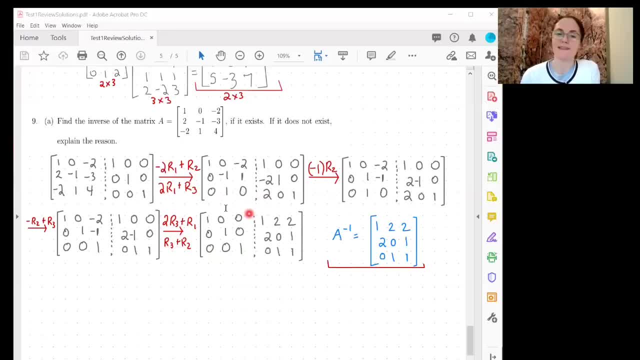 Row 3, add it to row 2.. And now we are in the final step. We see the identity, And that means this 3 by 3 matrix here, as you see, this is the inverse of A. Let me label this A. 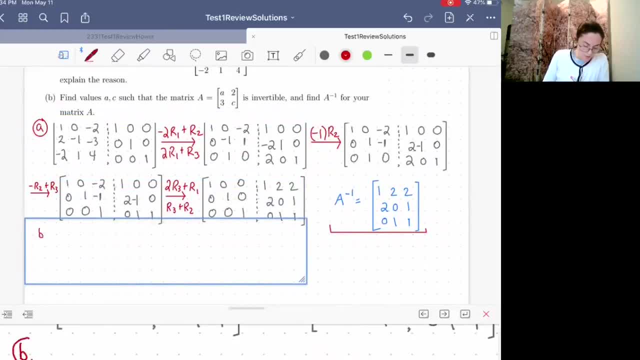 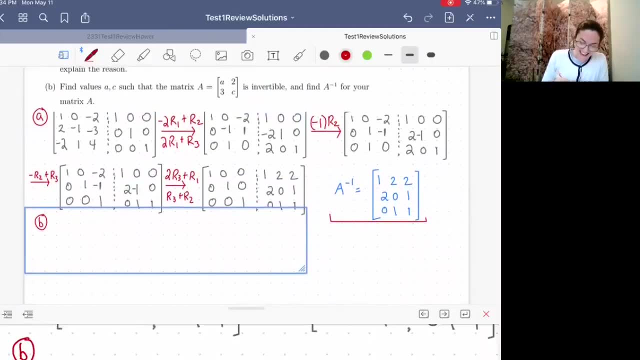 And now I'll move on and do B Right here. There's not a lot of space on the page, but I have room for B. Okay, This is a 2 by 2 matrix Here: A, 2,, 3, C. 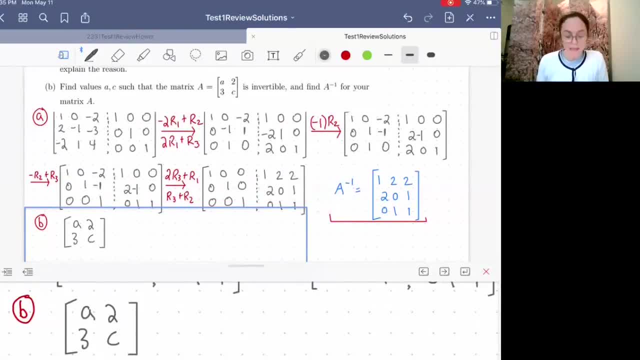 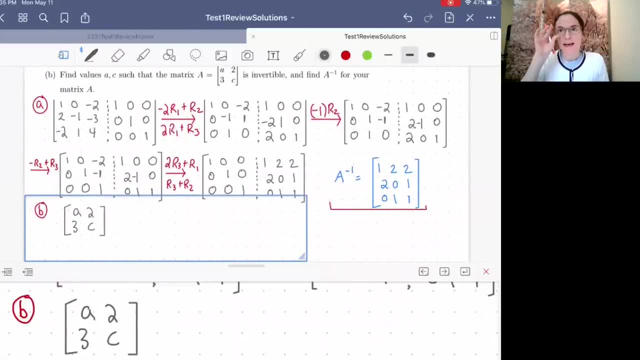 And this is something we discussed. I mentioned the word determinant, And for a general matrix, you don't have to worry about what a determinant is yet, because that's coming later in the semester. But for 2 by 2s, the determinant of this is: well, let me get my laser. 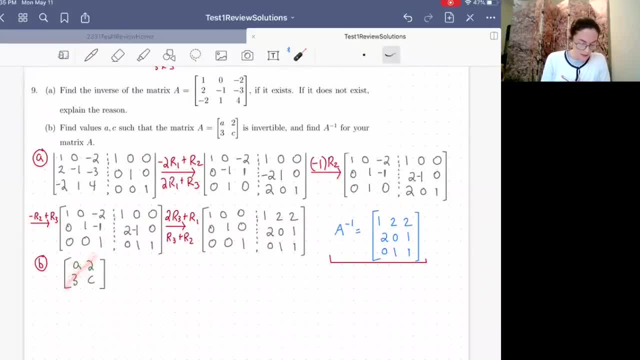 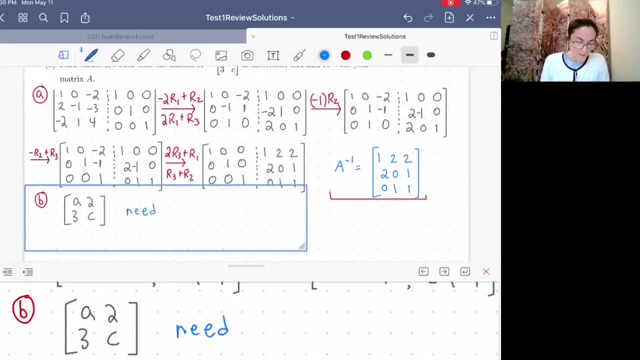 It's this minus this, So this gives us a characterization of exactly when 2 by 2 matrices are invertible. So let's write that here What I need for this to be invertible, because it says: find values A and C. 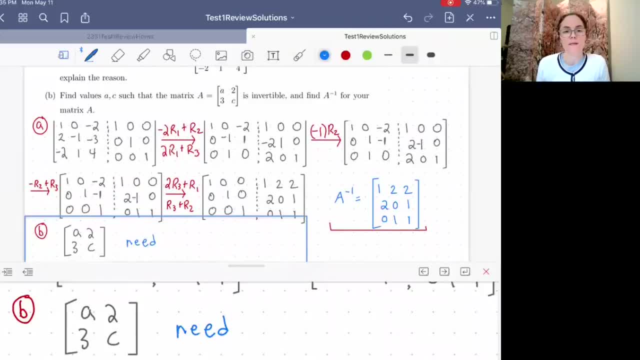 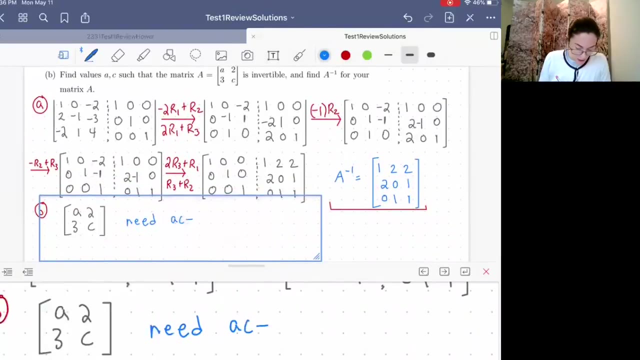 we can just find one set, One A, one C that work together such that this little 2 by 2 matrix is invertible, And then we'll find A inverse for our specific choice. Okay, So what we need is that a C minus 2 times 3 is not equal to 0. 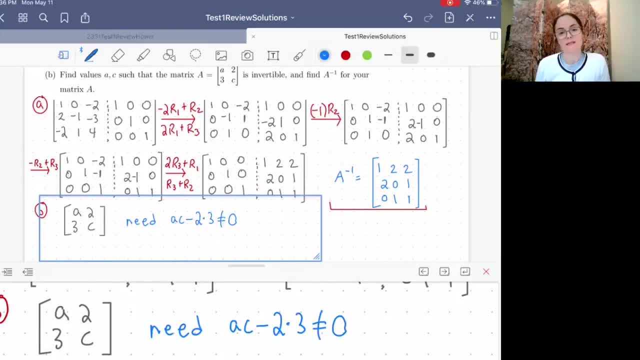 So you have a lot of freedom with your choice of A and C. Just don't make them multiply to 6, and you're good. But I'm going to pick – what's the easiest we could pick. Well, either both 1 or both 0, because that would make the matrix pretty easy. 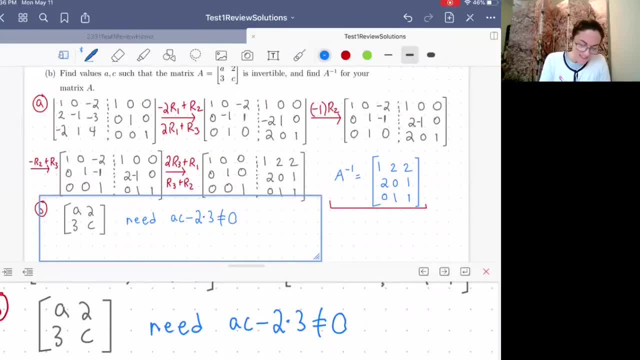 So let's make them both 0.. So I'm going to choose: A is C is 0.. Okay, So here's part of the problem right here. But, like I said, any two numbers, as long as their product is not 6, will work. 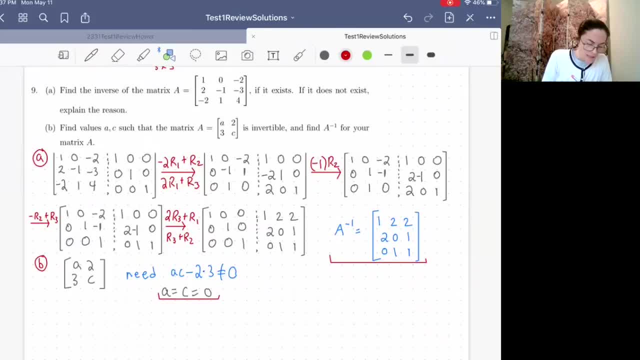 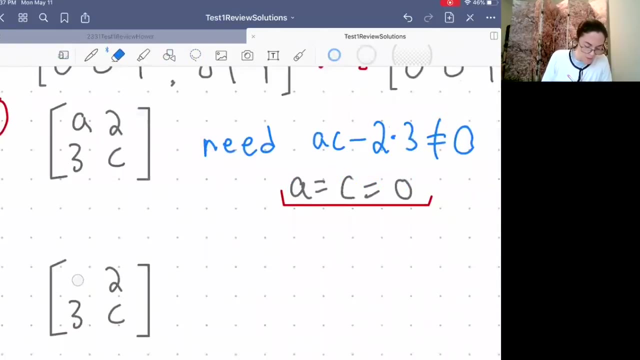 and the matrix will be invertible. Now let's write this matrix And I will recall or mention the formula for an inverse of a 2 by 2 matrix. So what I need to do is fill it in with my choice. I chose 0.. 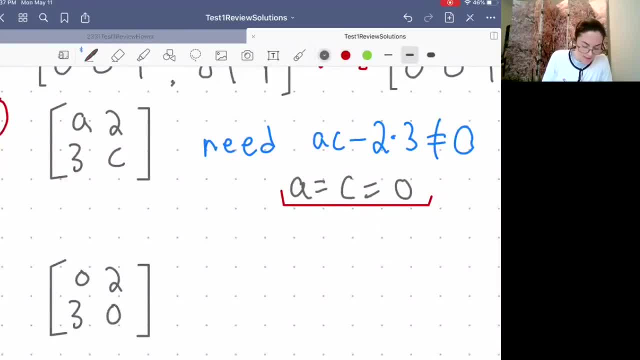 0. 0.. And then the formula for the inverse is – okay, Well, you take 1 over the determinant, which is this: Okay, So we take 1 over – in this case it's minus 6.. And then you flip the diagonal or you interchange the diagonal. 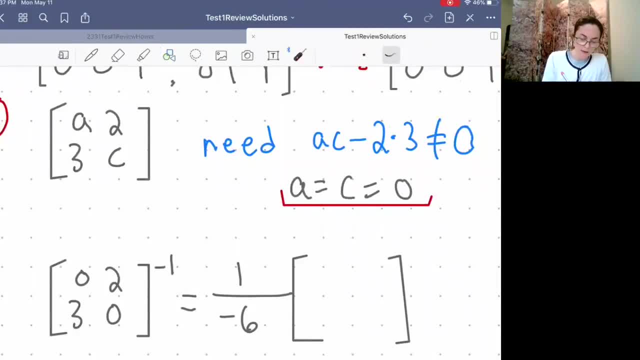 Okay, Or you interchange – maybe that's a better thing. You interchange these two. Well, I interchange two 0s and they are two 0s, And then you take negative of the off-diagonal, So this will be negative 2, negative 3.. 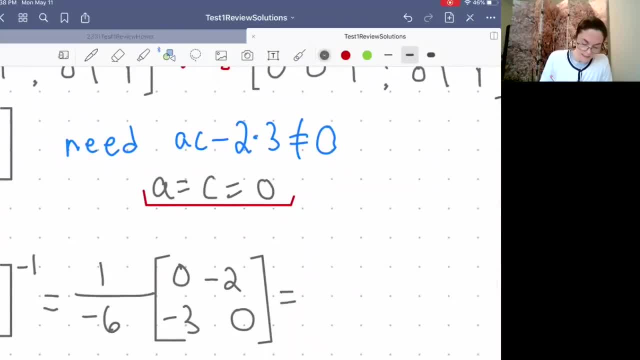 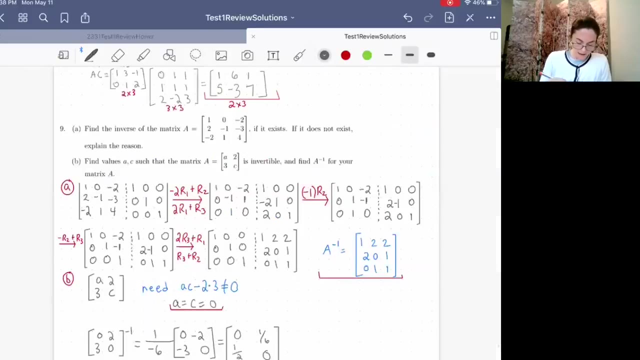 And this simplifies some right. In fact, I will make it simpler. We will have – when I multiply, I will have 0.. 0.. This is a third and this is one-half. And if you'd like – maybe I will, because I have space. 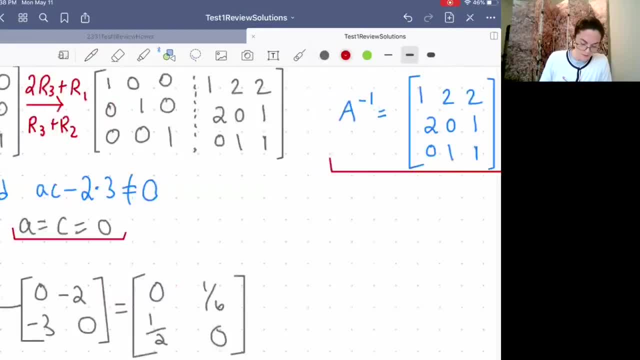 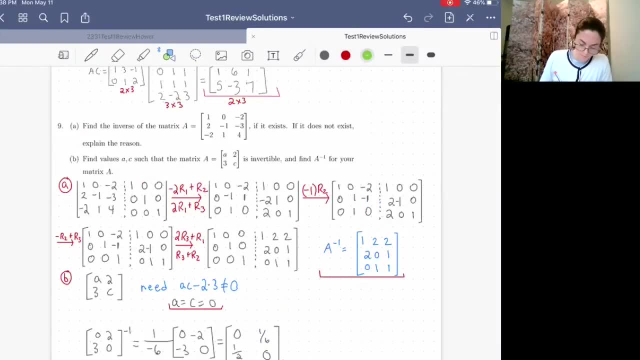 So first of all let me box my answer here, But then let me draw a little box over here You can check. We should get that A times this matrix is the identity And similarly, this matrix times A is the identity. 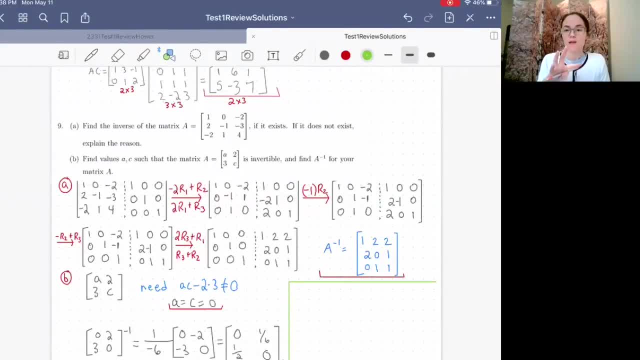 But you know, whenever you have an n-by-n matrix and you have another n-by-n matrix, you only have to check one side, since the product of the two is the identity, And then automatically that matrix is the inverse, And if you multiply the other way, you would also get the identity. 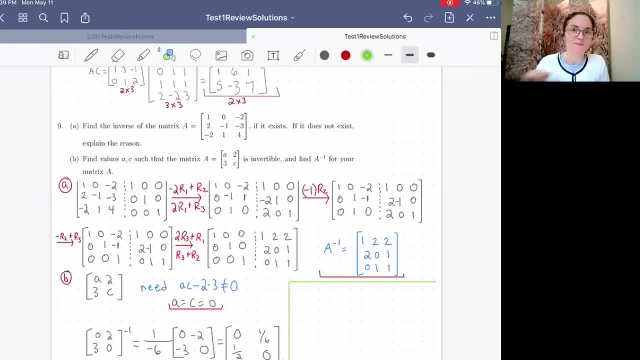 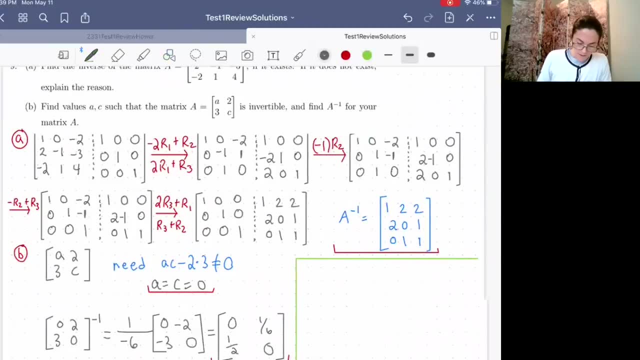 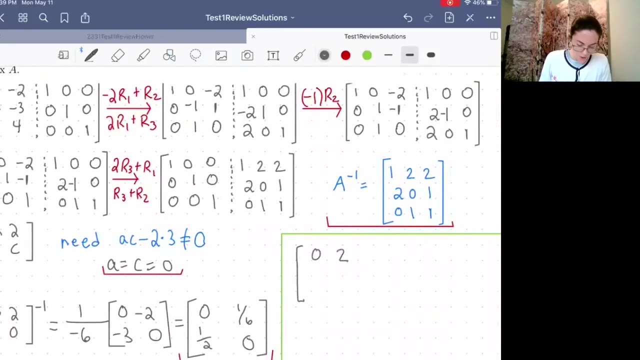 And this is really important to understand. It only holds for square matrices. Okay, So let's just check And then we will move into multiple choice. If I take –, what's my matrix? 0,, 2,, 3,, 0.. 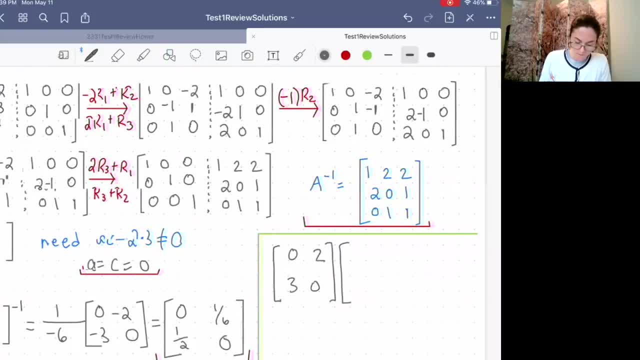 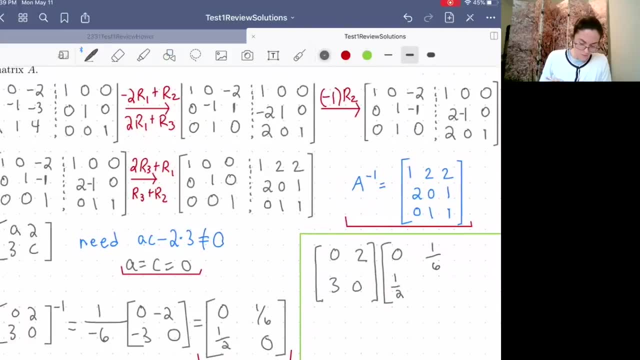 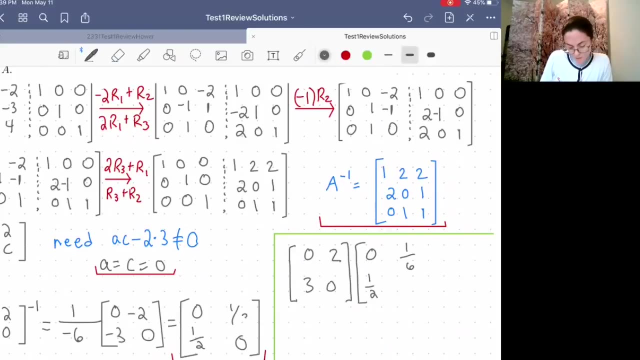 So now I'm doing A times A inverse, although I could have checked the other way. Oh Nope, The same. This is why it's good I checked. 2 over 6 is not 1 sixth, It's 1 third. 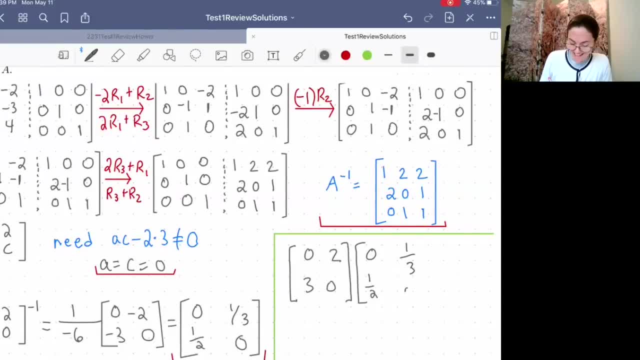 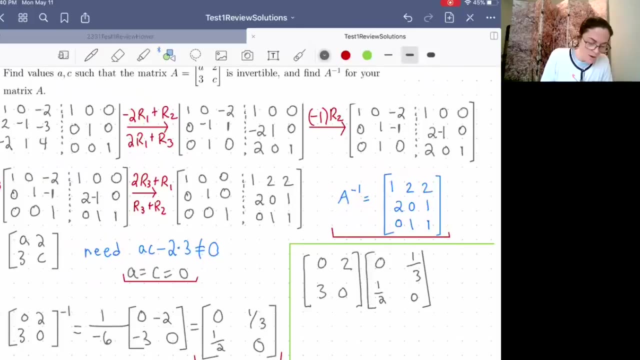 I was looking at it, realizing it wasn't going to multiply right, And then I realized I had written it wrong: 2 over 6, 1 third. Okay, Hope we're okay Now. this is why – well, you've probably seen me make mistakes before. 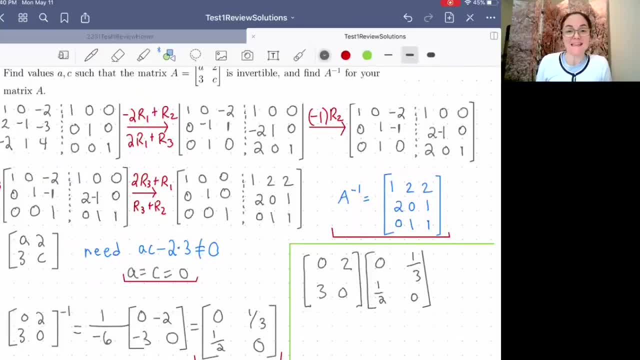 I try to edit them out of videos, But if you were actually in person in class, you would see more mistakes than you've seen in videos. So I would just say I am human, just as you are. It's why it's really good to check your work when you're taking an exam. 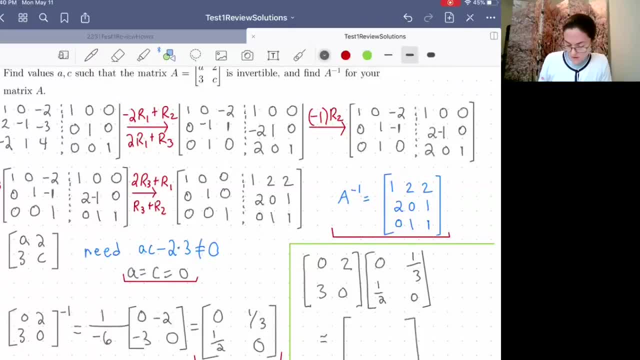 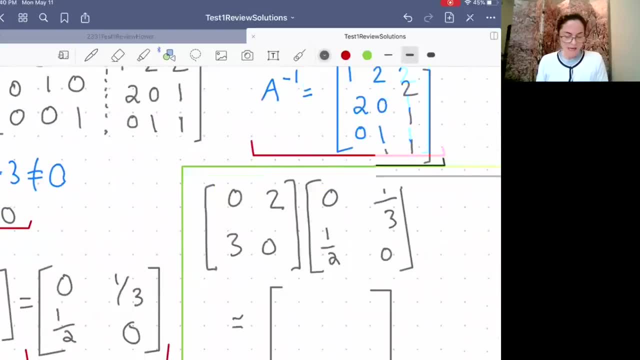 because mistakes happen to anyone, no matter how much you studied or how ready you are or any of that. Mistakes, they just happen. Okay, So now if we multiply these two, you see, in fact we get 1 here, We get 0 here. 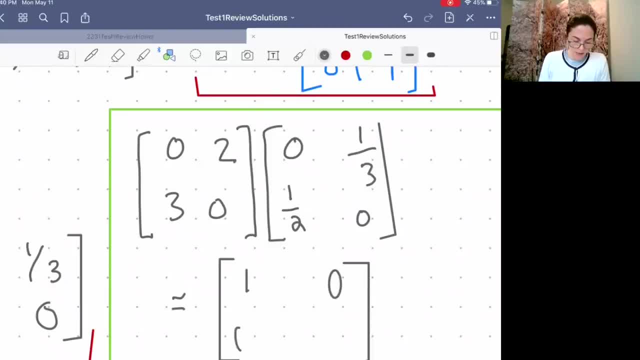 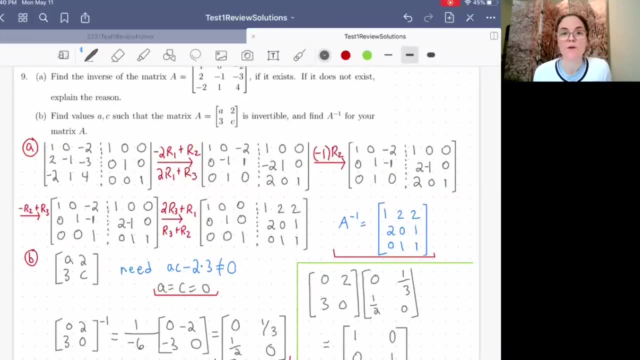 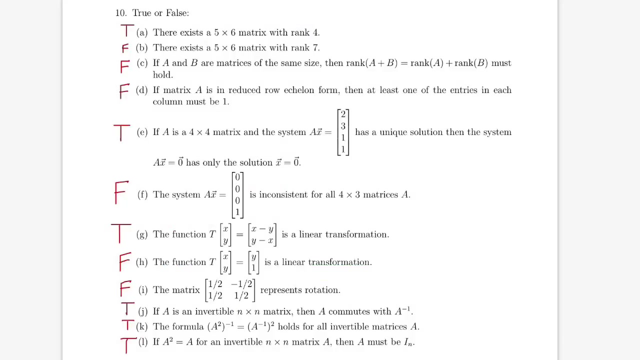 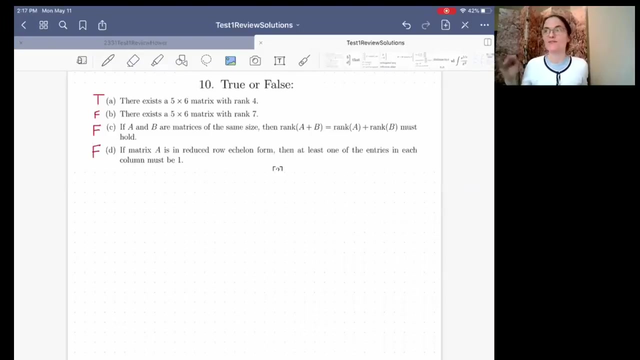 We get 0 here And we get –, oh goodness. And we get 1 here. So we do have the identity and this is the correct inverse. Okay, Now we move to multiple choice. I just flashed the –. I just flashed the answers: true, false, true, false, whatever. 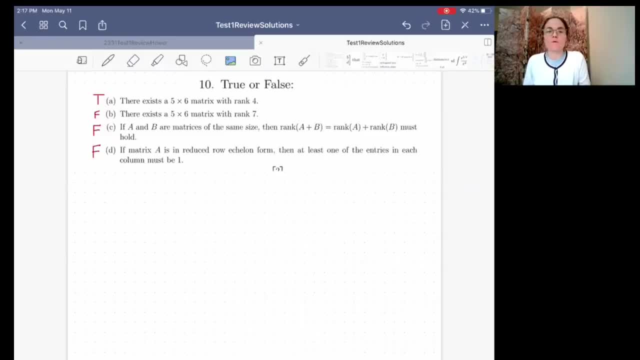 But I want to talk about why, because that's what really matters here. So I'm going to go through. I think there were 12, true, false. I'll put four per page and we will discuss. Okay, So here we go. 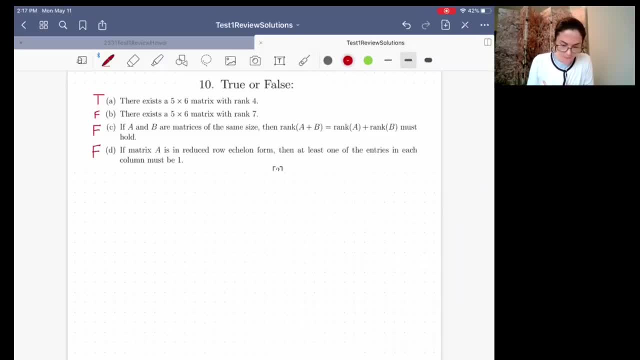 This page will be A through D. Maybe I will use different colors. Well, A, of course, to answer true, here we're going to use red, white and blue. There's the wrong way. There's another way. Let's just go to the opposite side. 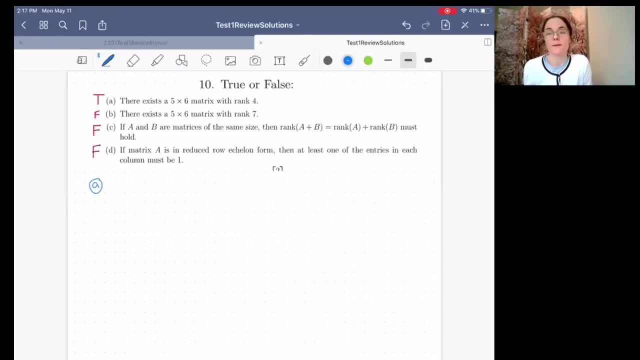 I think it's – Okay, So here I am. I'm going to choose this red, white and blue. I'm going to pull up all the reds And I'm going to drag over to the left. I'm going to go to the right here. 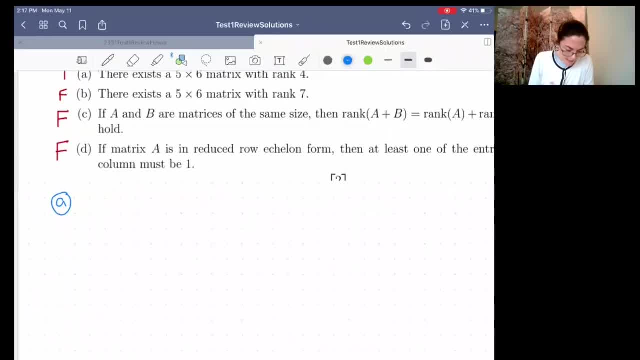 I'm going to click this and I'm going to pick these reds. Is this the right way? Then I just to this. I just click this Again. I can make this switch. I can change the color. I can choose to change the color. 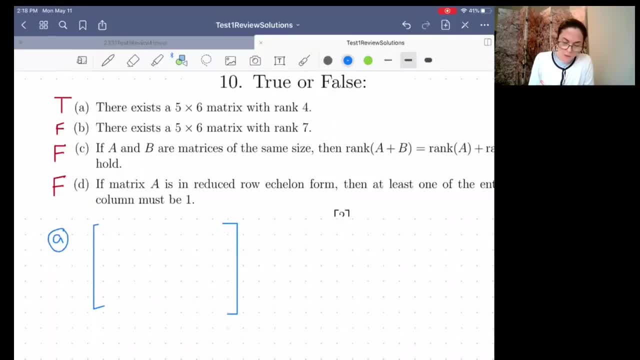 This way I can see exactly the same color as the former, And here the color that I'm looking for is this white, and then I can change that. columns of all zeros. There we go. There is a five by six matrix of rank four. Very nice. 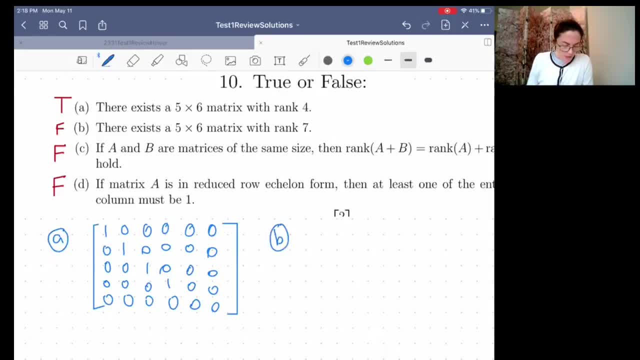 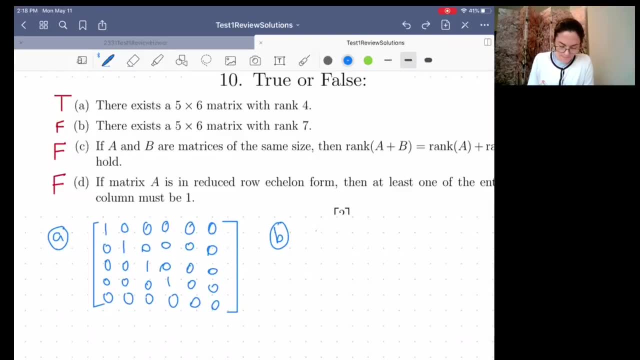 Now, what about B? Well, the answer isn't false, because we know the rank of A. Let's say A is N by M, then the rank of A must be less than or equal to N, and the rank of A must be less than or equal to M because, well, the rank is defined to be the number. 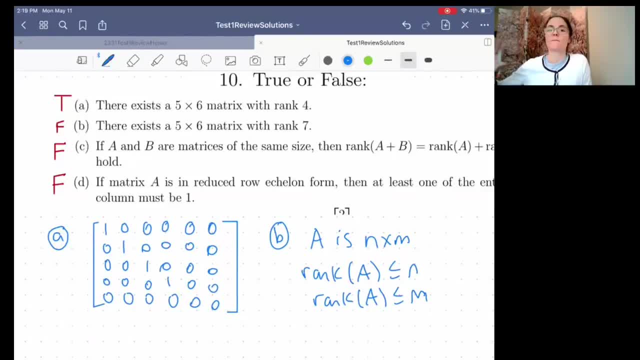 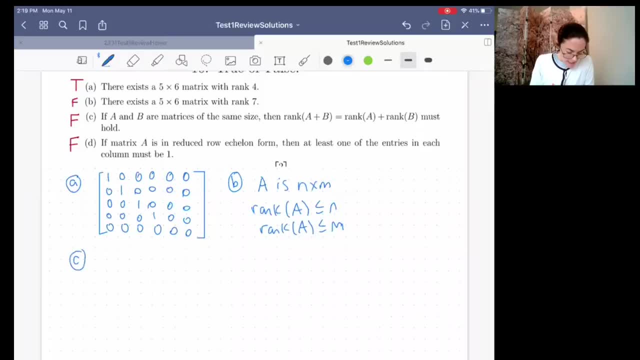 of leading ones in the reduced row echelon form of A, We are moving on to C. This is definitely not the case. In fact, I can find it. I can find some two by twos that fail. Here's a two by two. What's the rank of this? It's. 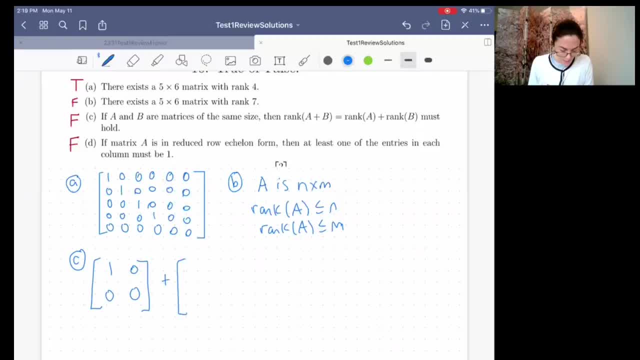 one. Here's a two by two. And what's the rank of this? It's one Right Good. The first one is already in reduced row echelon form. The second matrix I wrote. to get it to reduced row echelon form, just multiply through by minus one, But these two sum to 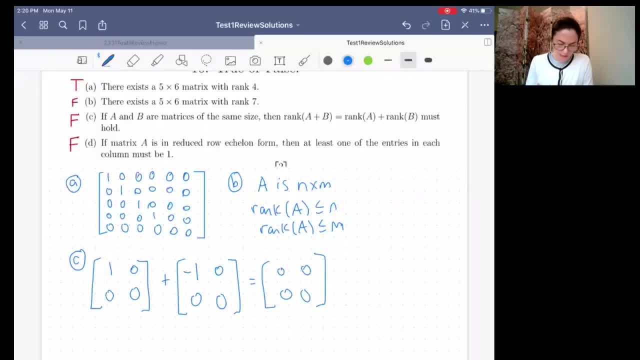 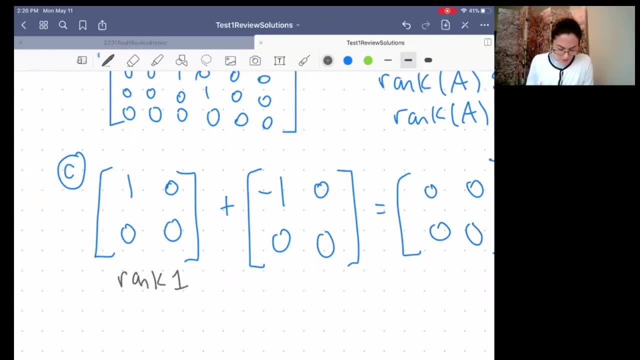 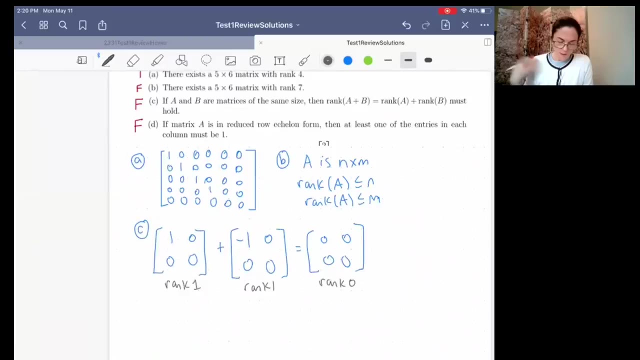 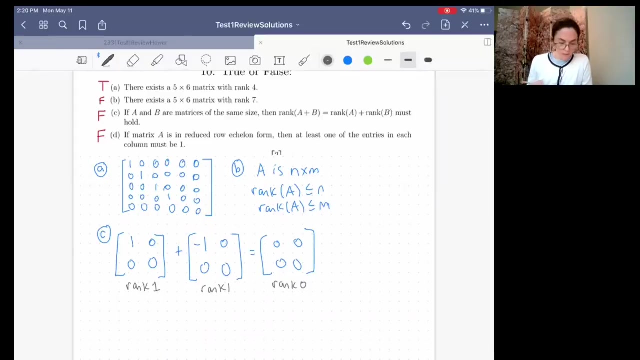 zero matrix, And here the rank is one, The rank is one, And we add them up and we get something of rank zero which is not one plus one. Okay, so this is why C is false And in fact, D we can use as false from the exact same or at least part of the exact same example. 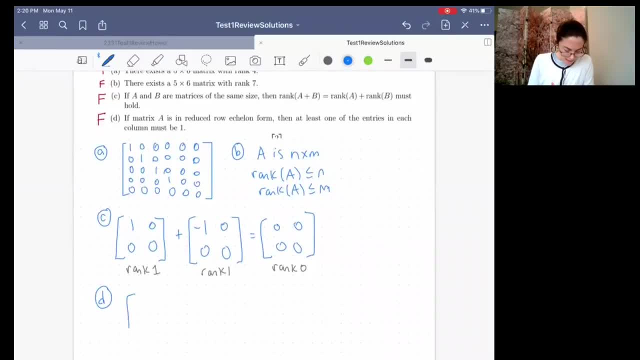 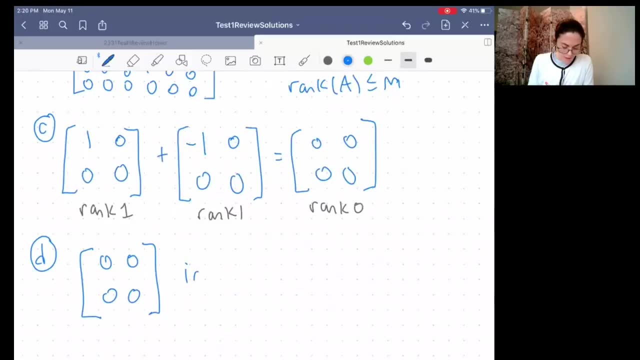 D is false Because this matrix here of all zeros, this is in reduced row echelon form. In fact, I had a question in teens. Somebody asked me: that Is the matrix of all zeros reduced row echelon form. Absolutely it is. It's rank zero. In fact, this is the only rank zero matrix is the zero matrix. 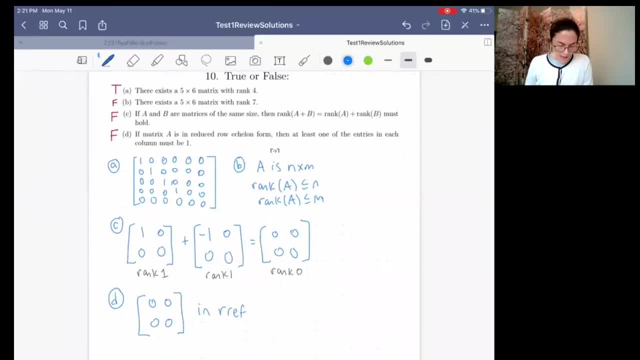 Okay, we have no leading ones. The rank is zero. So we see this matrix is in reduced row echelon form. At least one of the entries in each column must be one. Well, that's false, because the entries are all zero here. 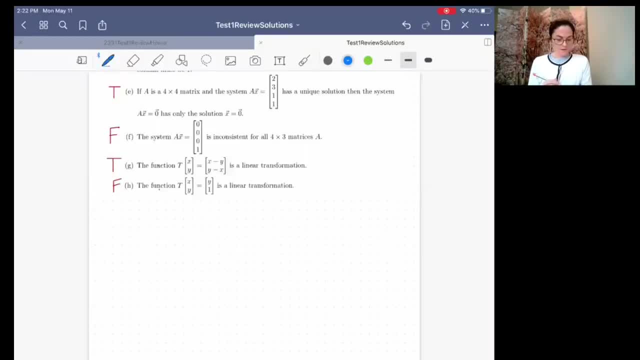 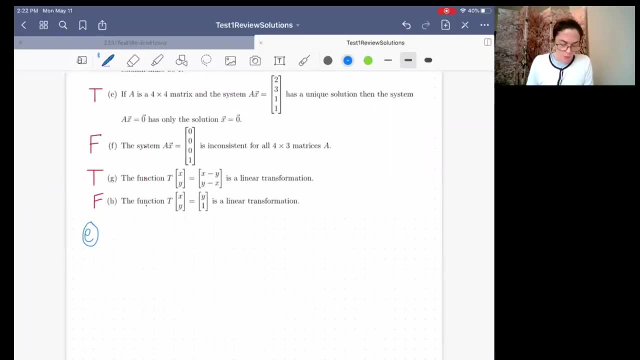 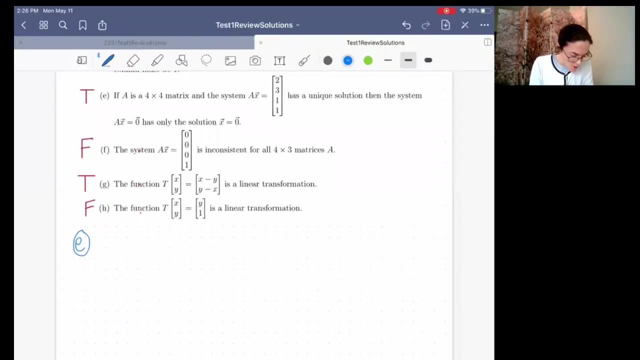 Okay, so here, what do we see? This is letter E. It says it's true. Well, let's discuss why. We have a unique solution. This means there are no free variables. If you have no free variables, well then the rank is the number of columns. It's a four by four matrix. 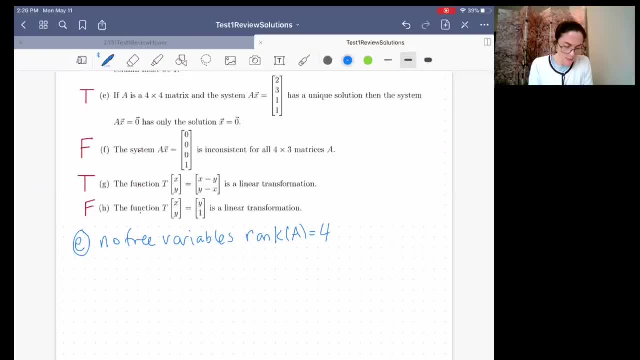 And then, in particular, just this part: having no free variables. AX equals zero will have only the solution X equals zero. Okay, this is true. Okay, Looks good. Well, in particular, it's good to observe that AX equals zero is never inconsistent. 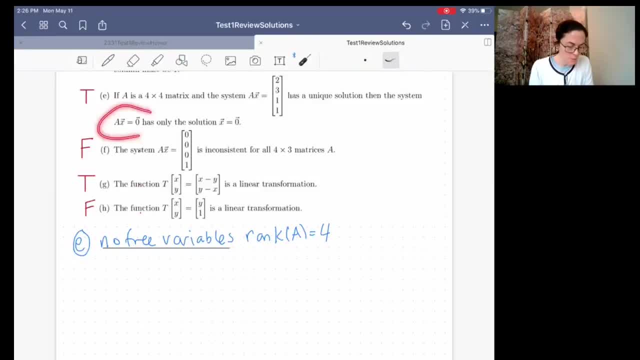 This one. this is a comment that we will come back to more when we talk about the kernel of things. This system that I have circled many, many times, no matter what your matrix is, even if we didn't have these hypotheses, it's never inconsistent because A times zero, the zero vector is always zero. 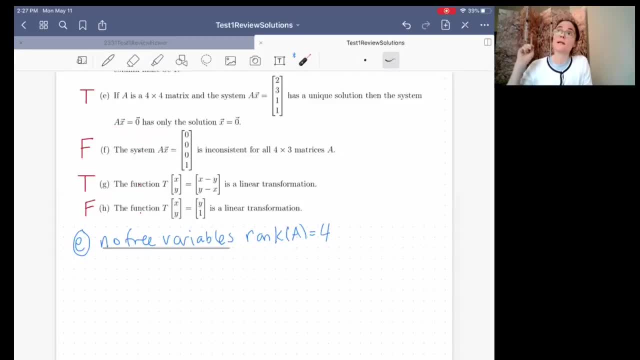 So this system, This system always has at least one solution, but given that we have no free variables- that comes from this part, we know it has- that's the only solution. Okay, very nice. Now let's think about F. 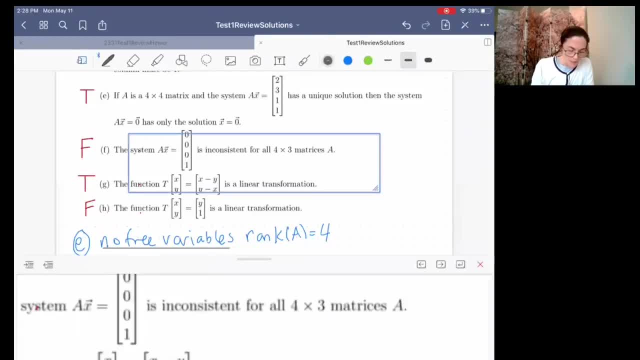 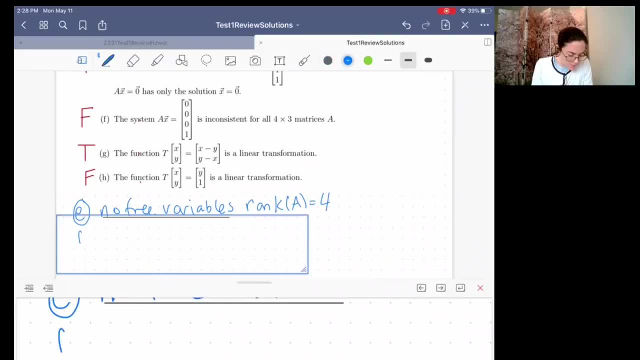 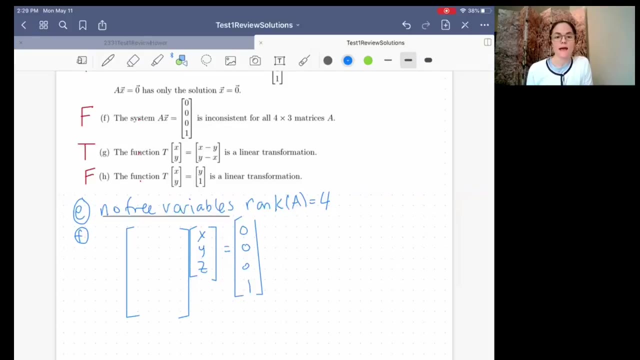 This is definitely false. Let's just come up with an example. So now I am on F. Now let's discuss Number F. well, this is definitely false and I just have put here this would be four by three. maybe I'll write that underneath, just to think about the sizes. this is four by three. this vector is three by one. the result will be four by one. but we have a lot of choice here. we can pick A and we can pick X. we just need there to be a solution. 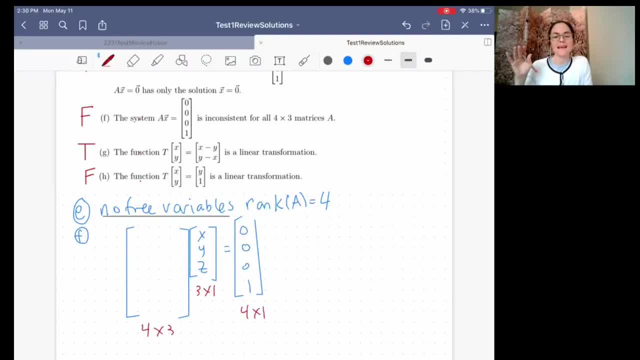 If you think about matrix Times vector as a linear combination of columns, it's very easy to construct something that works here. So what can I do? I can just put, And then literally anything, except this last column needs to be this, And then I can put anything in my first two columns. 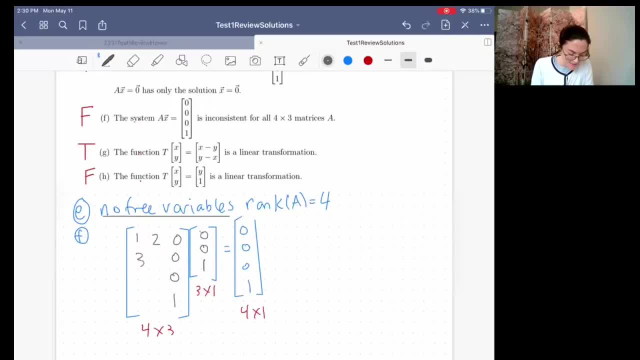 It really doesn't matter. so let's just do it: one, two, three, four, five, six, seven, eight. okay, And then linear combination of columns. you have zero times the first column, zero times the second column, one times the third column. this is exactly this vector. 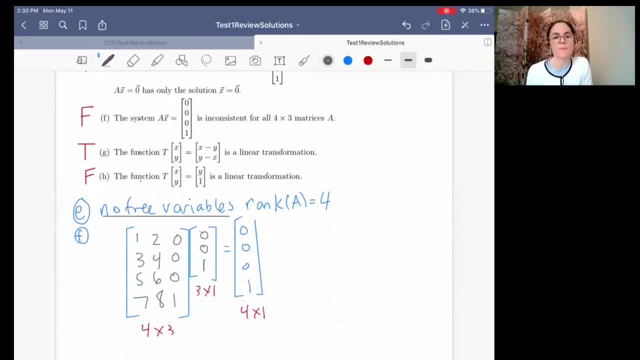 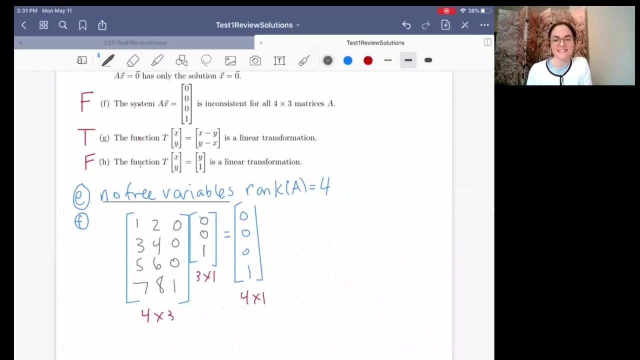 So you know, in fact, you can come up with many more examples, but this is definitely not inconsistent for all four by three matrices, These X, because I found one four by three and I found one X, for example. Okay, we could have come up with a lot of other examples on this one, but I just needed one. 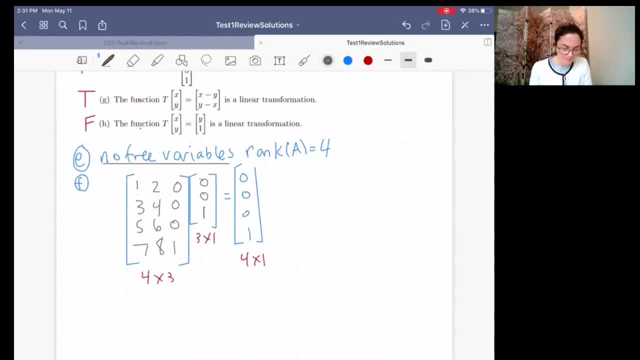 Okay, now let's do G and H. G is definitely true. Why would this be? Well, It might seem weird to just say, well, it just looks linear. You notice, zero goes to zero, and then I only see things that have power. one in them. 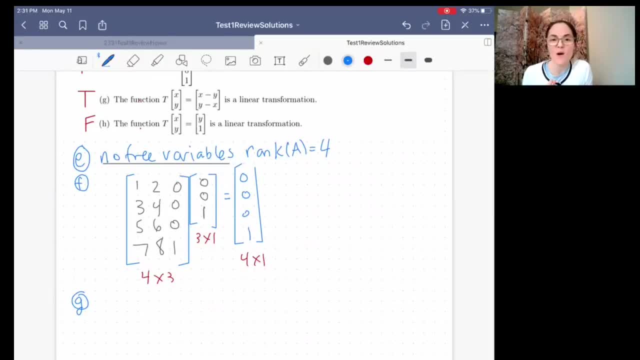 But if you wanted to prove it further than that, so I put a video of one of the homeworks where I justified why something was a linear transformation. You have two different ways. you could: One: you find the matrix and verify that that is what's happening. that T of, in this case would be an XY, is the matrix times XY. 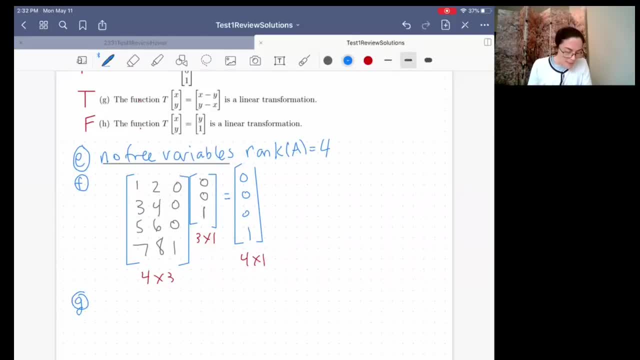 That's the definition, Okay, Or there are two properties you can check. Maybe here, just as an exercise, let's just show the matrix for this transformation, because this is part of the topics for this exam. Anyways, to get the matrix, I know the matrix would be T of E1 and T of E2.. 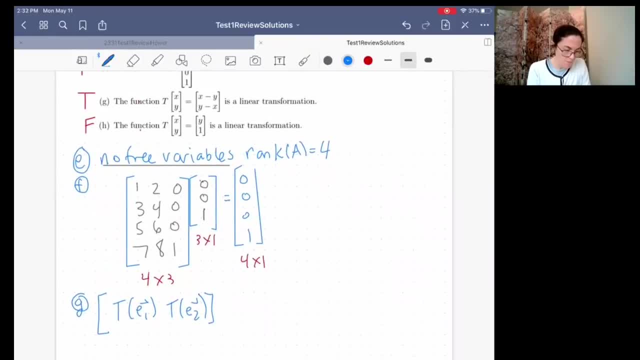 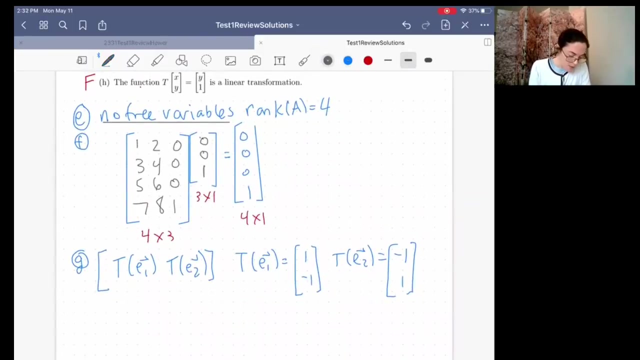 So let's calculate those here for this transformation. T of E1 is One minus one And T of E2 is minus one one, And so this says the matrix of this transformation better be one minus one, minus one one, And you can just check. A times XY will be: 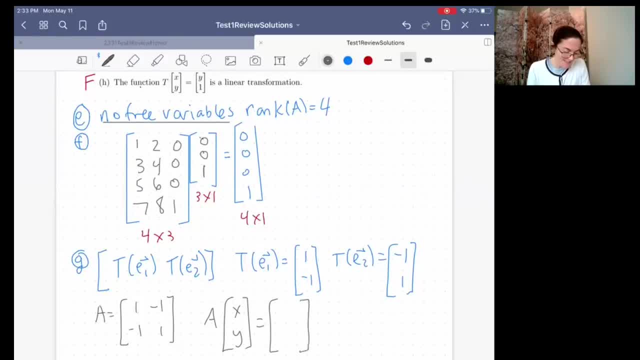 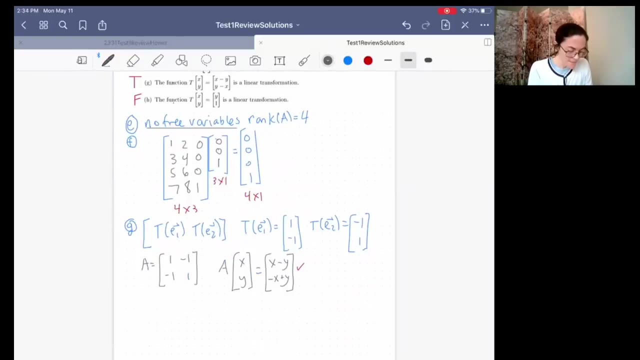 Oh, maybe I should leave a little bit of space here. Well, it's X minus Y, And it's minus X plus Y, which is exactly that. Well, it's exactly that operation, Right. Okay, Now let's do H. 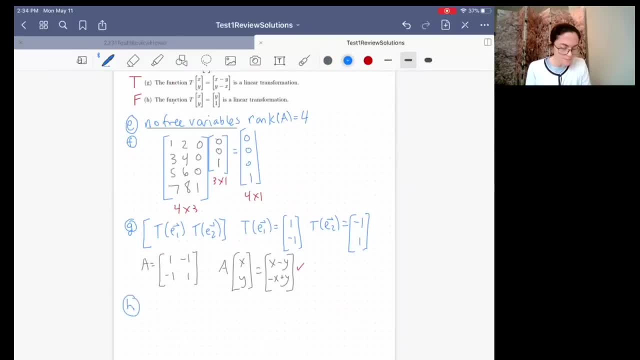 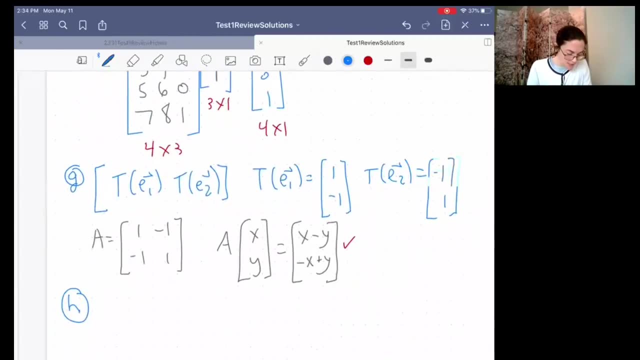 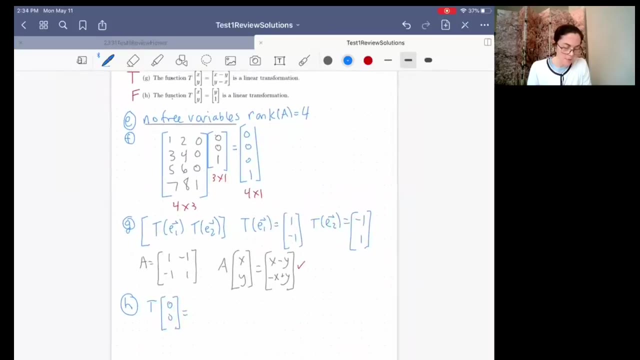 And then we have four more that I'll put on the last page. This is definitely false. The easiest way to see that this is not a linear transformation is This map on the zero vector gives us. well, look at the map: zero, one which is not equal to zero. 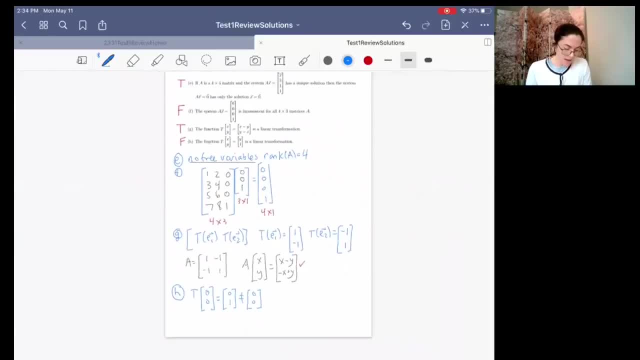 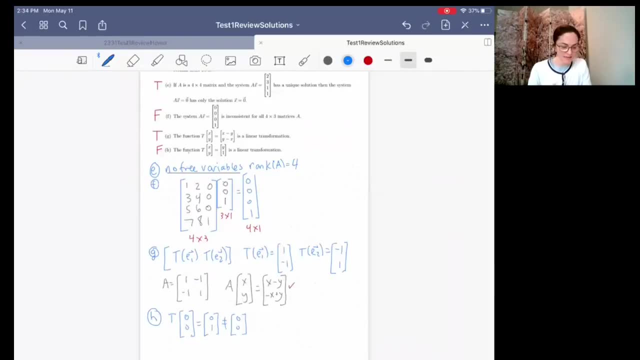 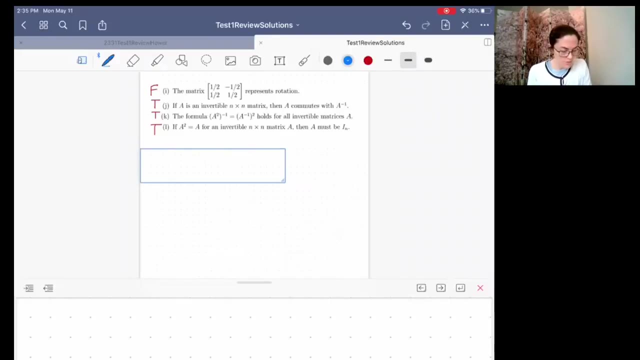 And any linear transformation must satisfy that. zero max to zero. Okay, And this one does not, So it's not a linear transformation. Here are the last four. Here are the last four. Um, Um, first of all, I false. 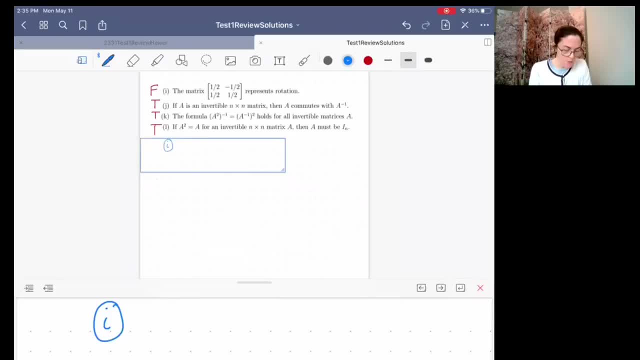 Well, what is a matrix that represents rotation? A matrix that represents rotation is of the following form: It is- uh-oh, maybe I'll get this- It is cosine theta, sine theta, minus sine theta and cosine theta, And this is the matrix for rotation. 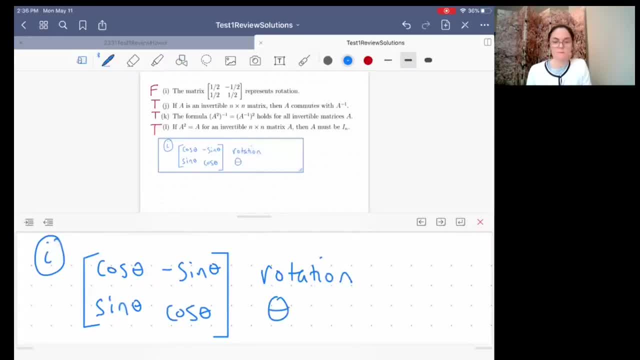 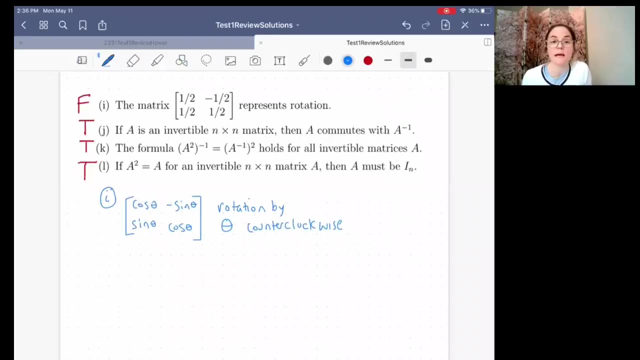 And so here is the cosine Theta, Maybe by theta, Counterclockwise. Okay, Now We do see a number, a number minus the number, A number. Except if the cosine of theta is a half, the sine is definitely not a half. 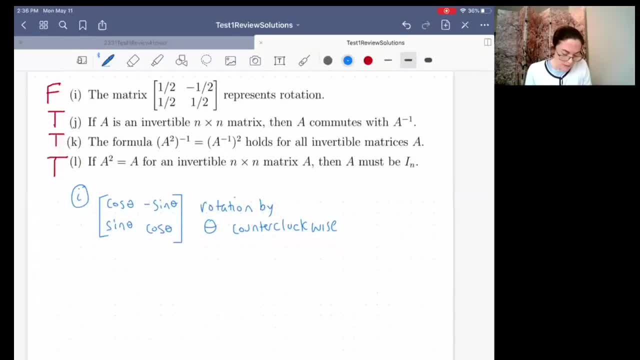 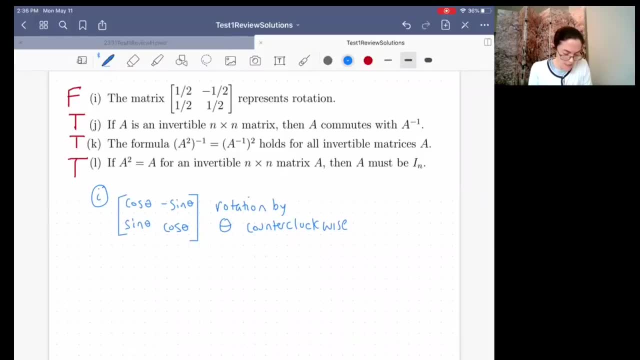 So, Um well, how could you argue that we need: cosine squared plus sine squared is one, and you notice that one half squared plus one half squared is a half, which is not equal to one, and so one half one half is not equal to cosine theta, sine theta, for any angle theta. but you could also just say: 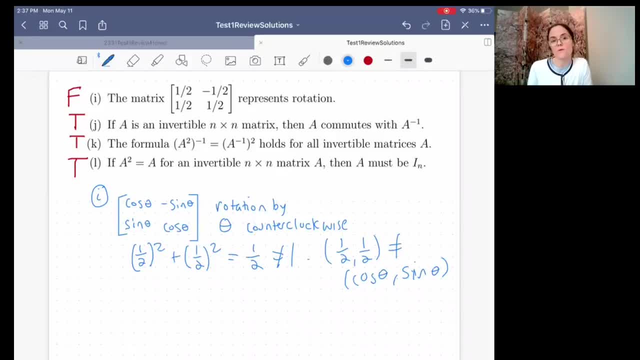 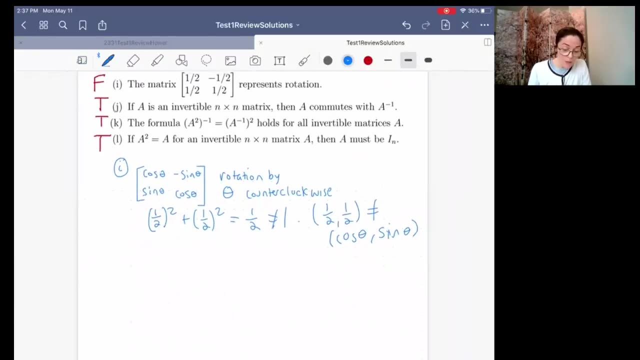 well, you know, the cosine is a half. the sine has to be square root of three over two. so this is not um rotation by any angle. okay, and the last three are all true. and the last three all have to do with um inverse, invertible matrices and inverses, and this is our newest topic for the exam. um, if a 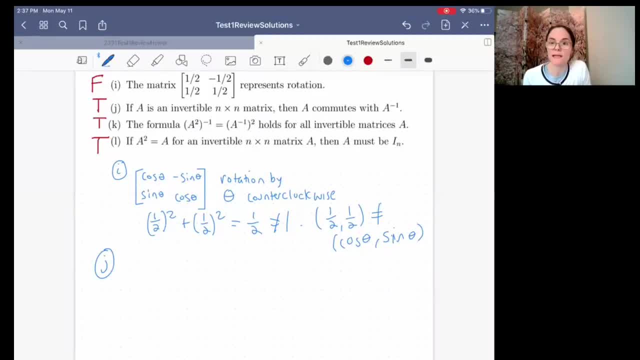 is invertible. a commutes with a inverse? absolutely it does. we've talked about commuting with a matrix, even in this review, but we know a, a inverse is a inverse, a uh-oh, which is the identity. okay, so that says exactly that a commutes with a inverse. k is true. and why is this? well, let's start. 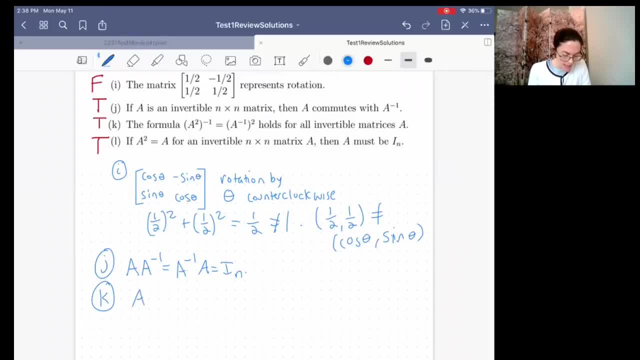 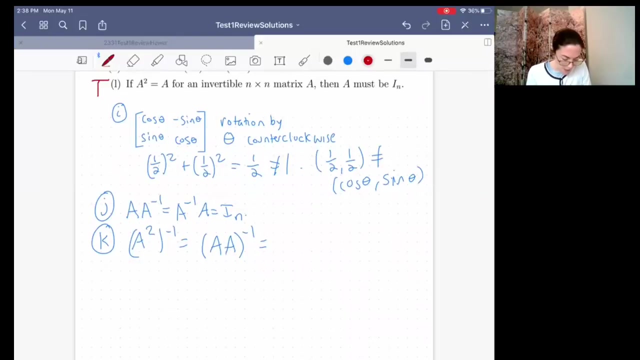 with the left hand side. we'll prove it. the left hand side- a squared inverse. well, we have formula. well, first of all, we know a squared is a times a, and then this is now. let's remind ourselves the formula underneath. there's another way i could argue this: that k is true, but we know if you have. 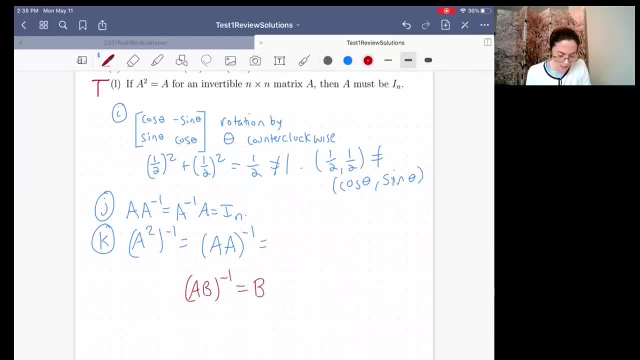 a- b inverse. this equals b inverse, a inverse. it's a property about inverses, assuming a and b are both invertible and they're both the same size, so that a times b is fine. so if they're both invertible and by n matrices, then this is a property. well, if i apply. 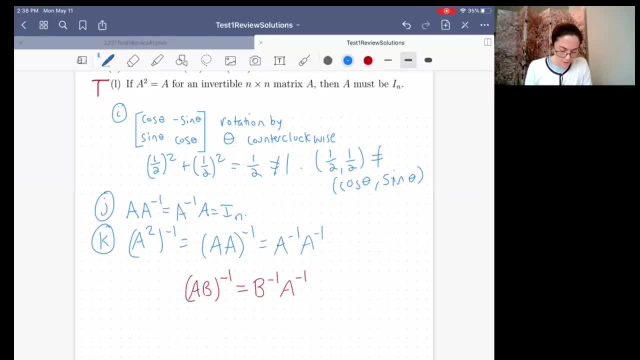 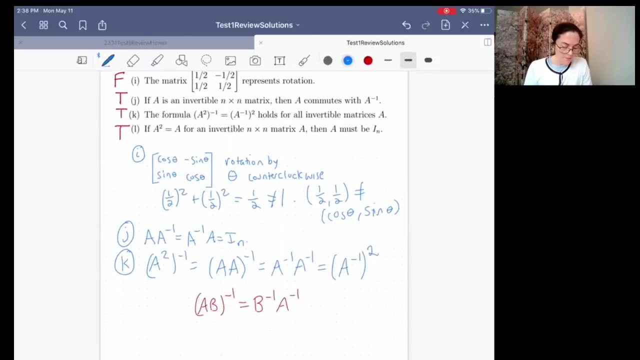 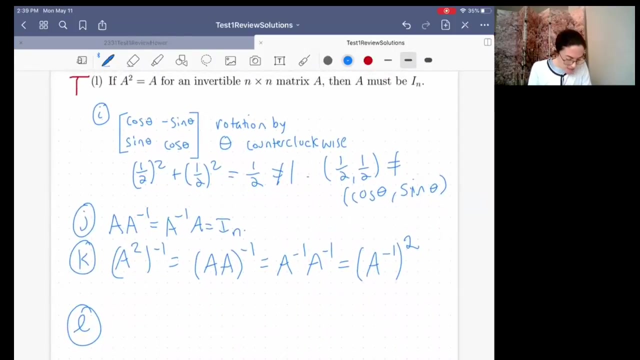 that here it just says a inverse, a inverse and this is a inverse squared. this is one way to to prove that formula. this one's interesting l is also true. okay, so a is invertible. this is an important part, because if a is not invertible, this last line would be false: a is invertible.